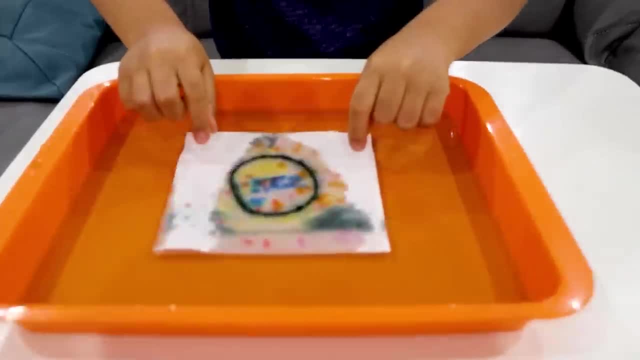 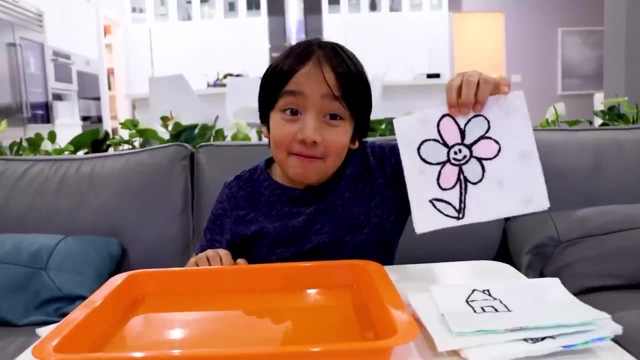 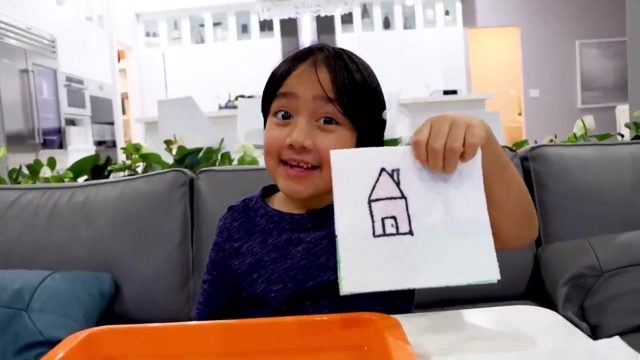 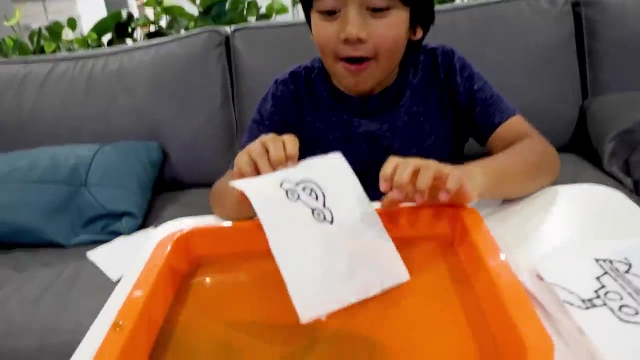 And then You see a super strong pizza getting delivered from the pizza factory. Okay, first you see a flower, Now you see A flower. Next, you see a house. Now you see A house with a tree. First you see a black and white car. 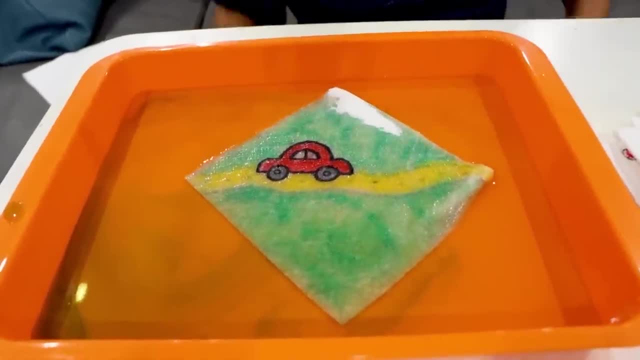 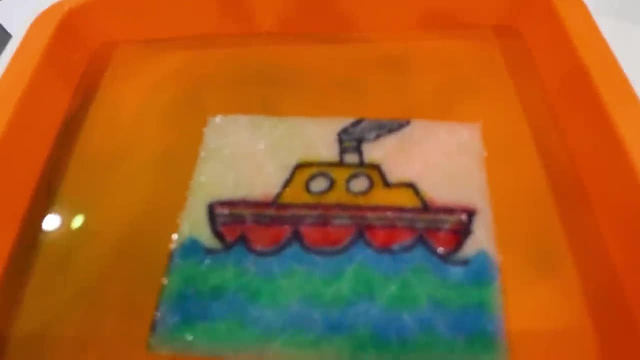 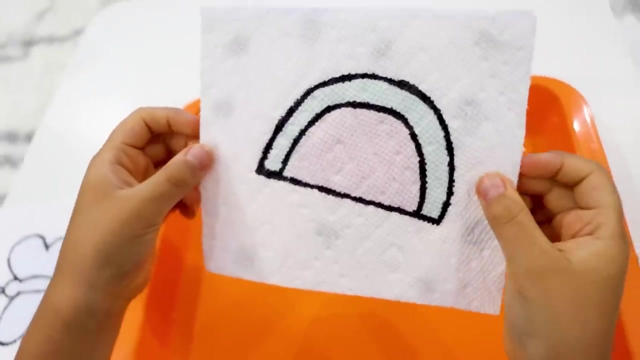 Now you see a car driving on the road. First you see a boat, Now you see A colorful boat. First you see ABC, Now you see ABC blocks. Now you see a mysterious portal, But now You see a. 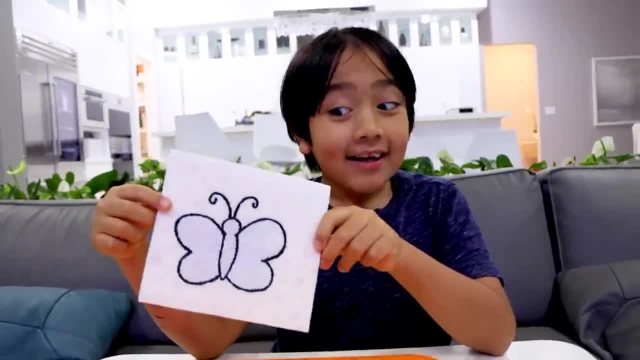 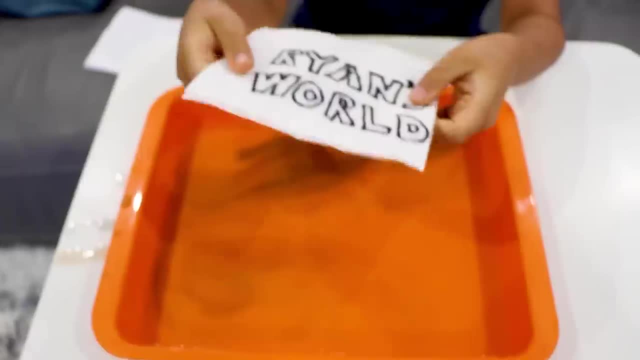 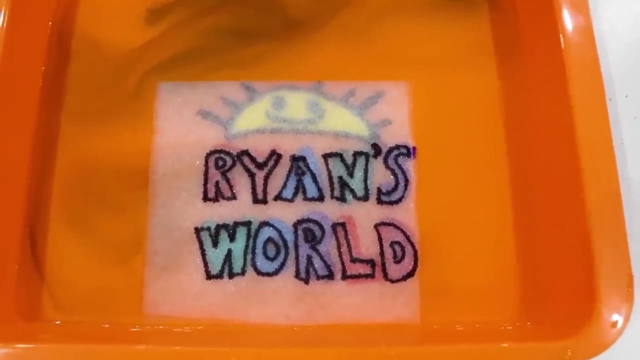 Watermelon. You see a black and white butterfly. Now you see A blue butterfly with a lot of stuff around it. You see Ryan's World. Now you see Ryan's World with colors. I hope you liked my paper towel and water magic trick. 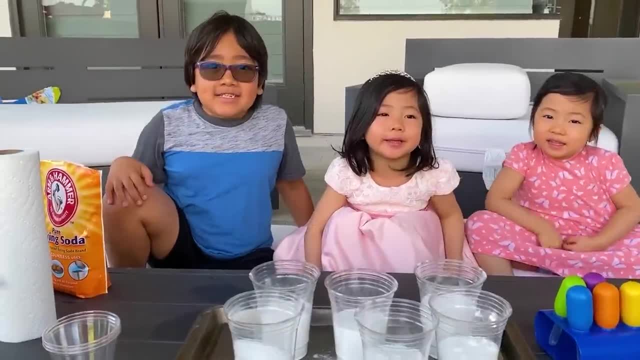 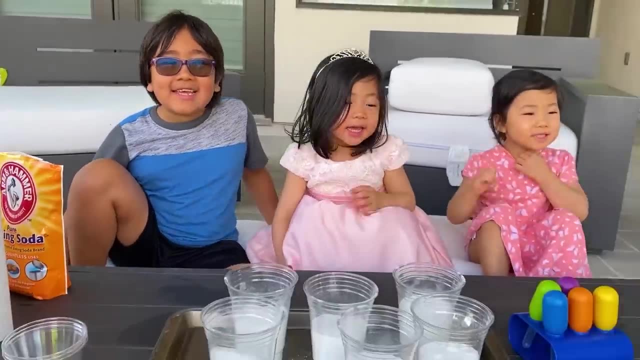 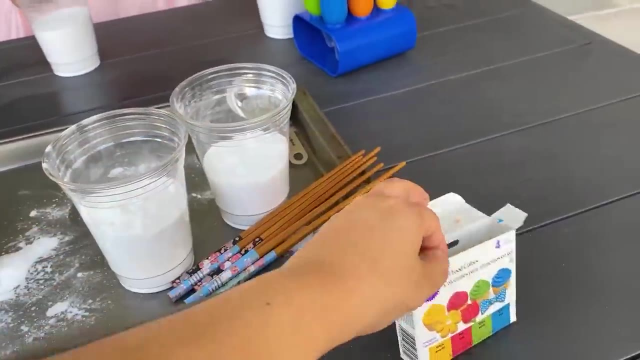 You don't see it, Now you do. Hi guys, Today we're going to be making a rainbow baking soda and vinegar science experiment. Are you guys ready? Yeah, Okay, guys. First step is you're just going to need a cup of baking soda and then your favorite color. 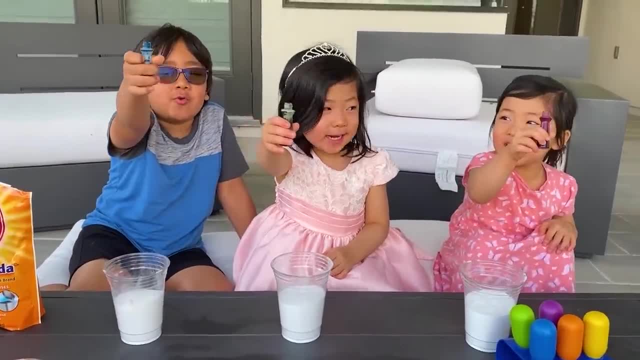 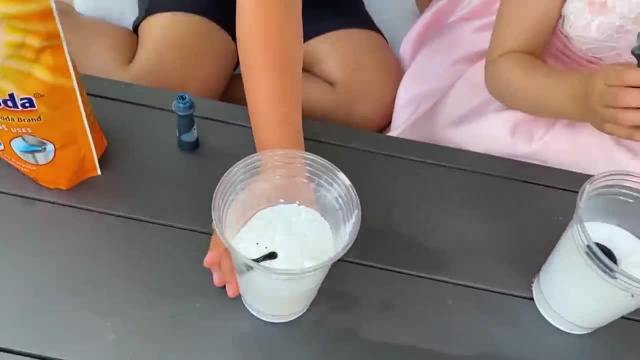 So what color are you guys going to add? Green? Okay, go ahead. Kate did some red, Emma did some green And Ryan did Blue. How do you even know Blue? Next, you're going to need to agitate to get something to agitate. 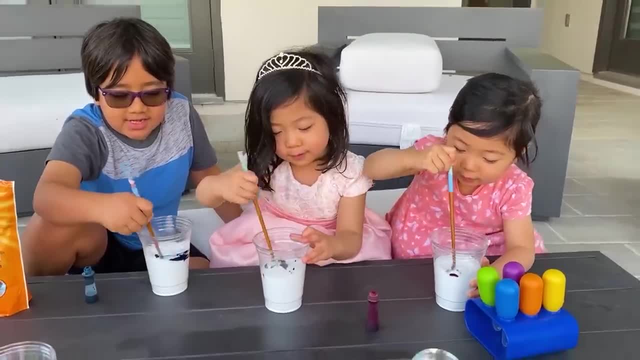 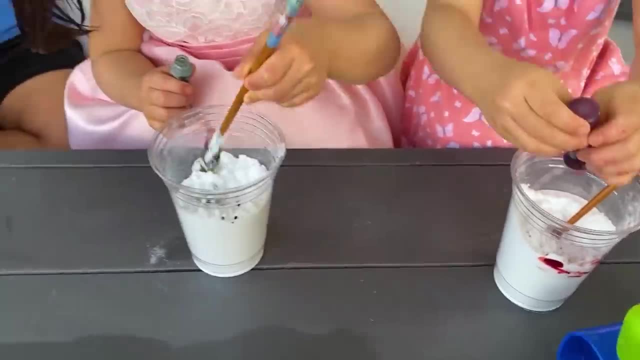 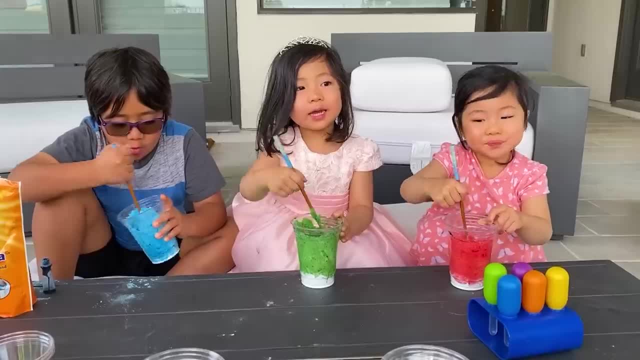 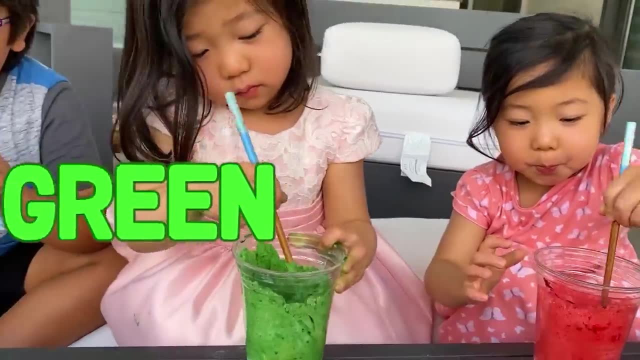 Wow, Yeah, Keep agitating. Good, I'm going to mix a little more. Yeah, so you guys' colors are going good, See red, green and blue. Good girls and boys. Okay, so we're done with our three cups. 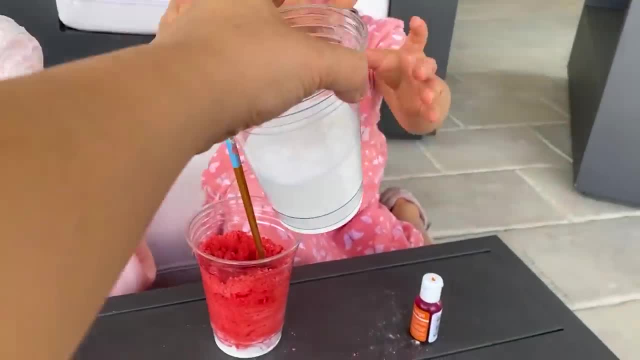 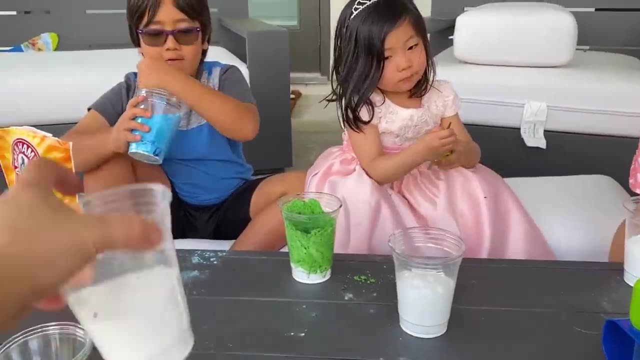 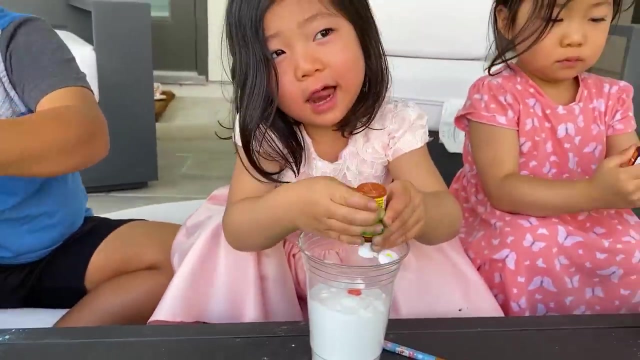 Now we're going to do these three. Okay, so Kate's going to do orange, And then Emma's going to do yellow, And then Ryan's going to do Purple. Good, There you go. add your color purple. It still doesn't look like yellow. 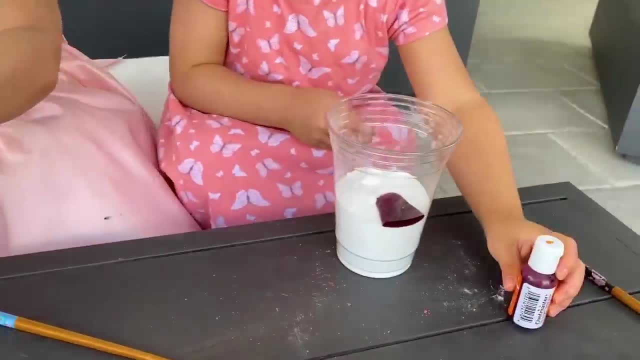 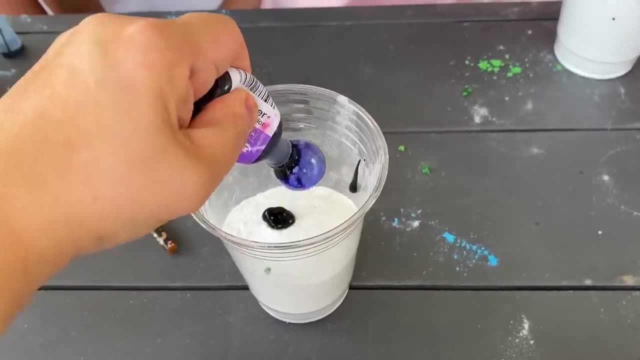 It will Good. there it goes. yellow Looks like orange. Kate got her orange. I think that's enough. Okay, there, it is Purple's out, but it's okay. Whew, look at the bubble. Look at that giant purple bubble. 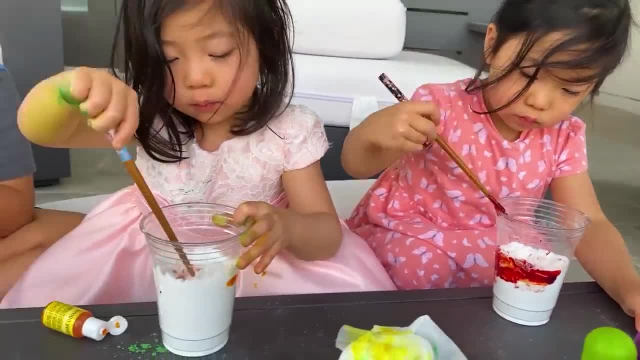 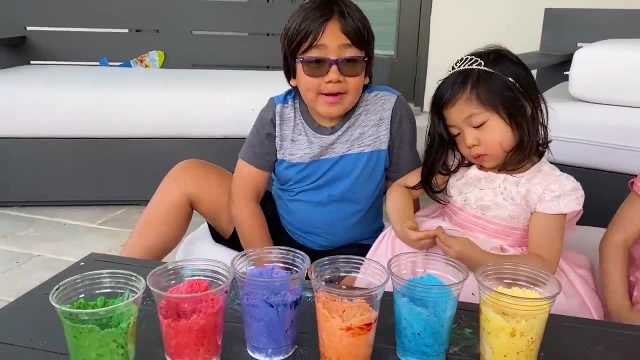 All right, start agitating. there you go, Agitate, agitate, Agitate, agitate, agitate, agitate, agitate. Okay, we got our rainbow colors. Nice Okay, guys. so now we're going to pour all the colors. 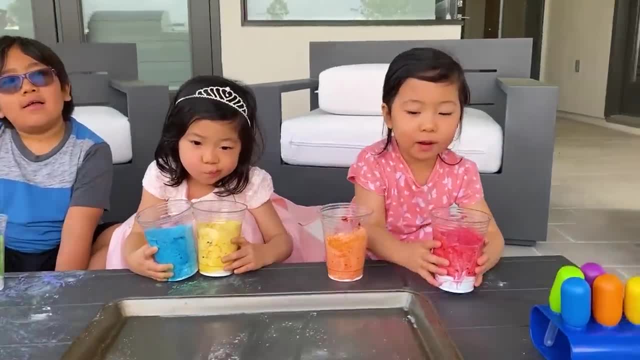 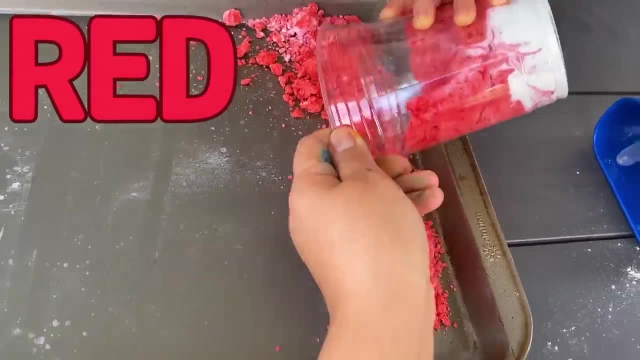 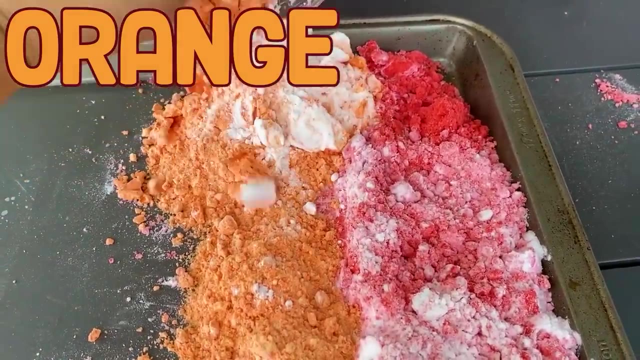 into this pan here. So, Kate, you can start first with red, Pour it in. Yeah, There we go. Okay, we got our red and now we're going to do our orange. All right, there we go- orange- Ooh nice. 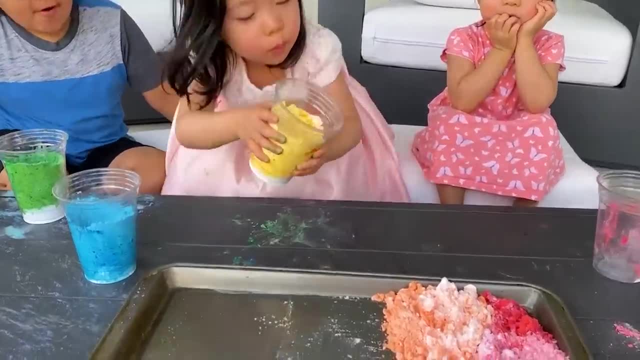 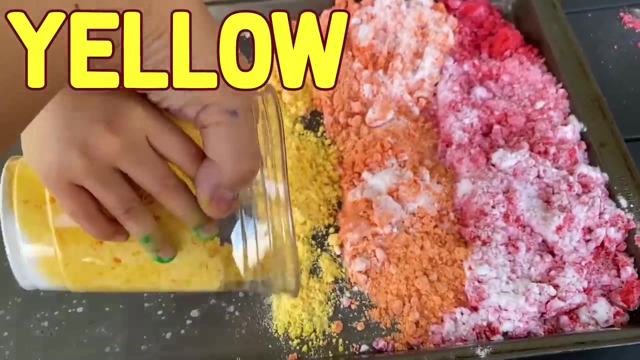 Good job, Kate, Let's go, There you go. good, I help you. There you go, It's okay. there you go. good girls. Wow, so beautiful, huh, Yeah, it's like a rainbow, Yeah. 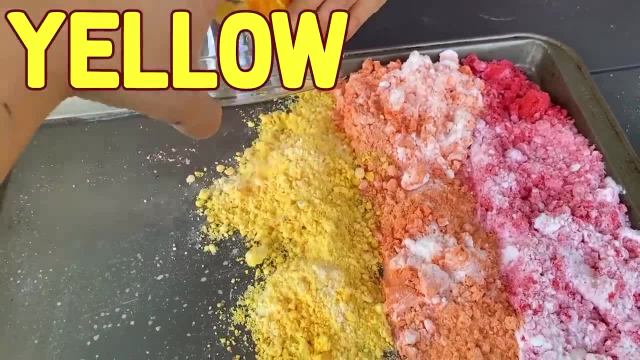 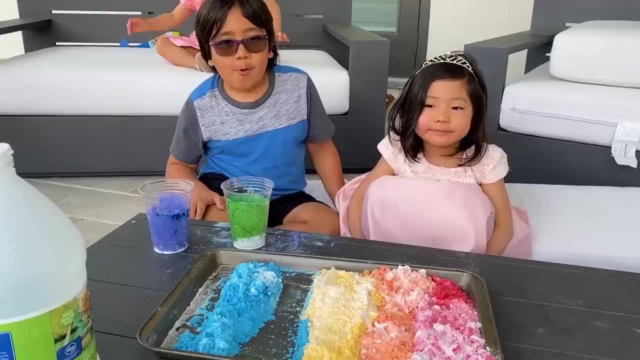 Can we pour the gold in? Can we pour the gold in? I want to do it myself. It's a rainbow. Now we do blue. Good, there you go. Yeah, beautiful. Okay, so we accidentally forgot the green here. 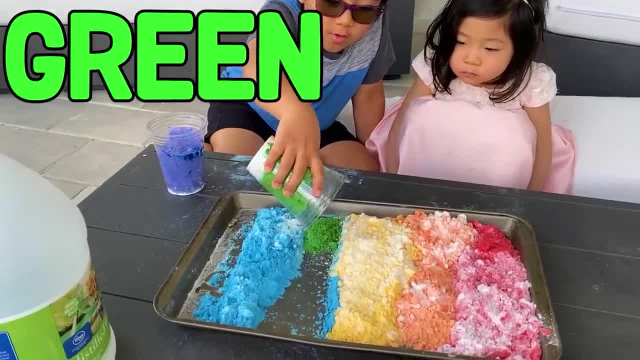 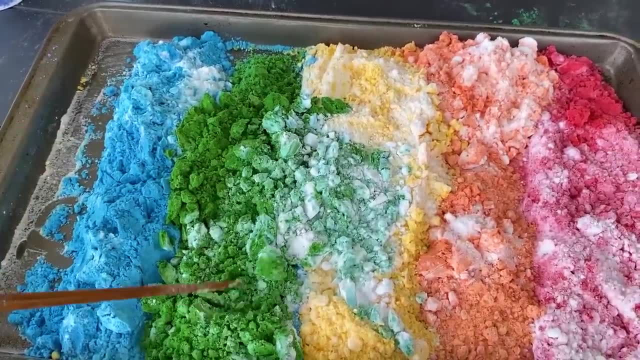 so Ryan's going to pour the green. Yeah, There we go. Whoa, It's okay, we can fix it. Spread out the green. It looks pretty. huh. Yeah, It's actually a lot of green. Yeah, It was like a rainbow, but now we need purple. 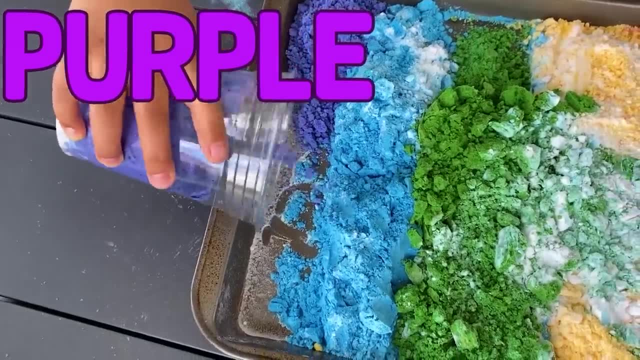 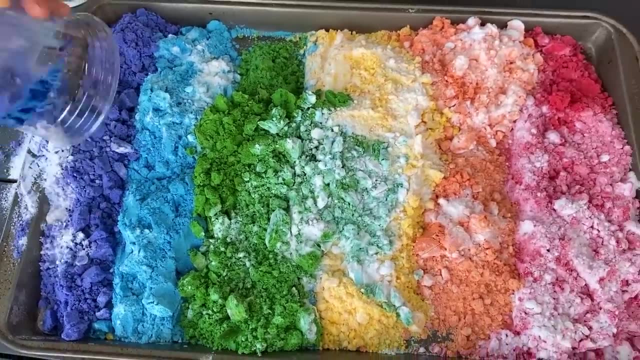 That's right. purple, Yeah, Wow, so beautiful. It looks like a rainbow It does. Now mom can do these things. Yeah, almost done. Good job guys. You're going to need some vinegar here. Can you help me? 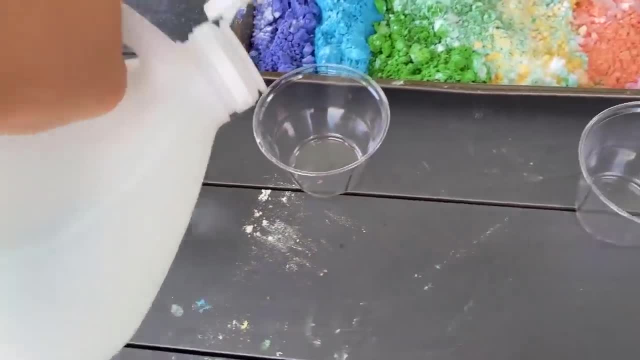 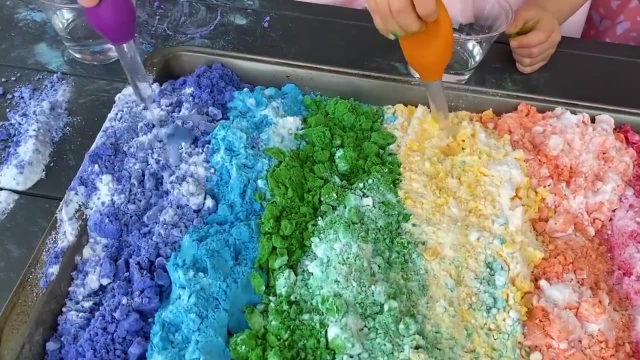 Yeah, of course. Okay, I'm going to pour some vinegar in each cup for you guys. Okay, there you go, Pick up some vinegar and then just do it. Yeah, I'm going to squeeze Like this. You see the bubbles. 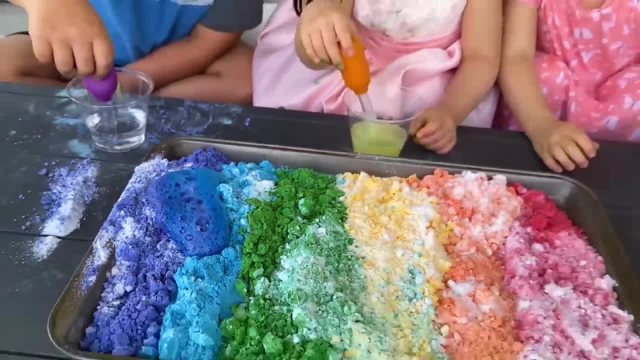 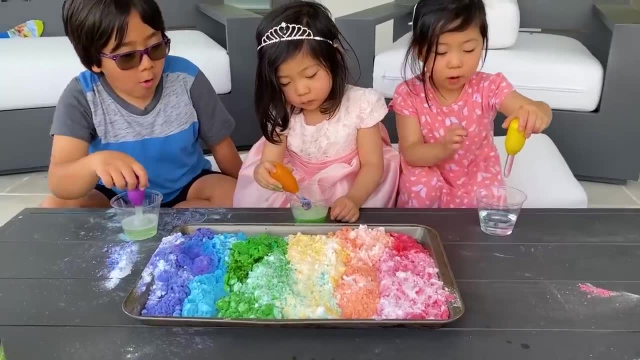 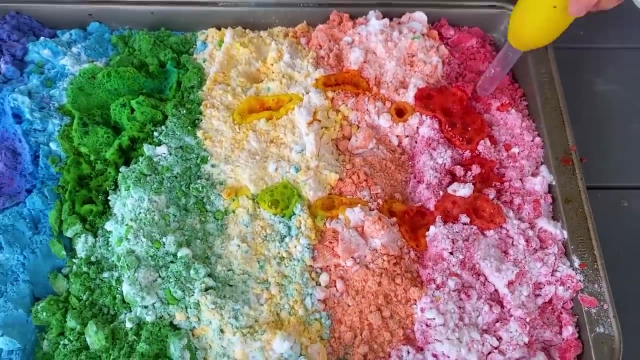 Emma: look, Whoa, Look, look, I put some bubbles. Wait, are you mixing it with the color Whoa, Whoa, Whoa, Look, mine is even getting taller. Wow, Mine is so many colors at the same time. 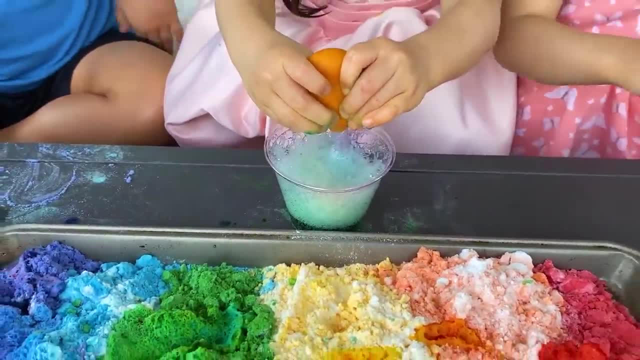 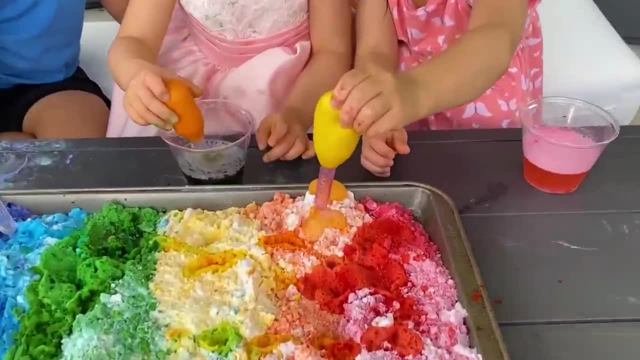 Yeah, Mine is growing. Emma's just mixing over there. I'm going to do both of them, all of the colors. Okay, Mine's just mixing together. Oh, that's cool. Whoa, Whoa, All right, Whoa. 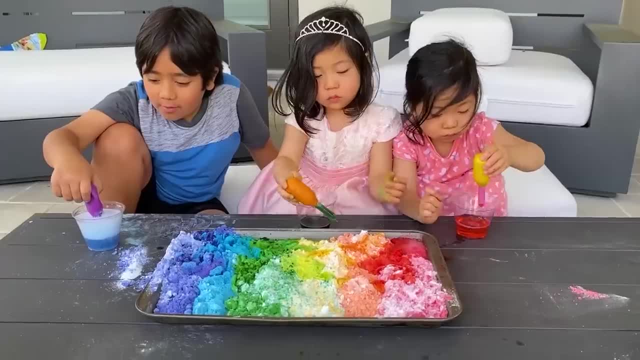 That's a big one. I have a reaction inside my cup: Whoa, Whoa, That's cool. Whoa, There's a spot you guys haven't done yet. Okay, I'm going to do it on one single spot. 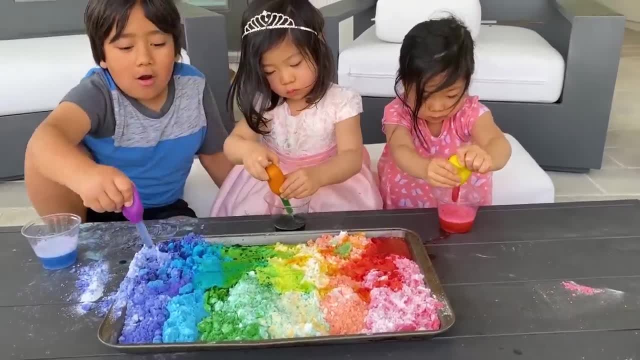 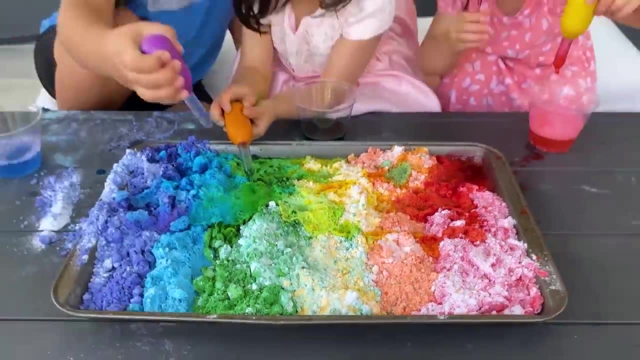 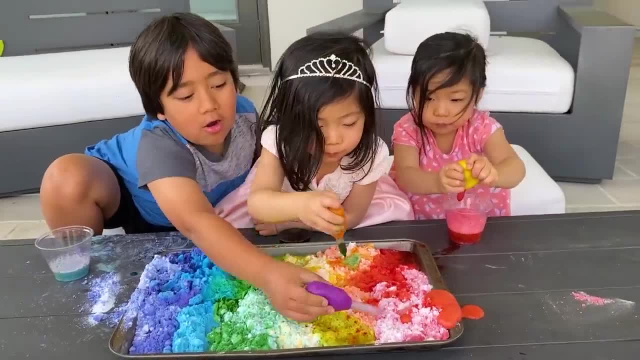 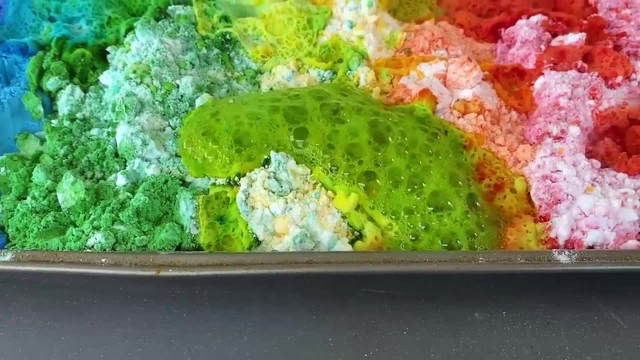 Whoa, Another one, Another one. Wow, Whoa, Sanjay has a real thingy. Okay, Eww, I love this. Oh my Welt, We've got to makedomo Yum, Yum, Yum. 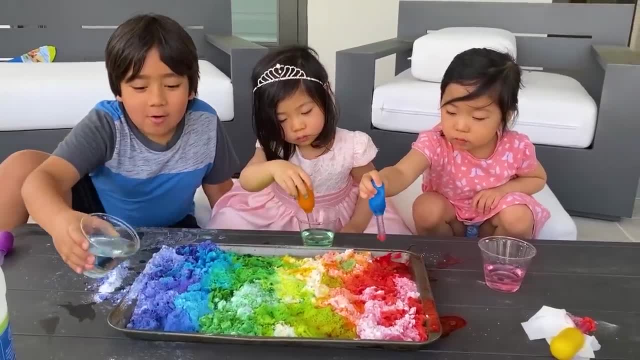 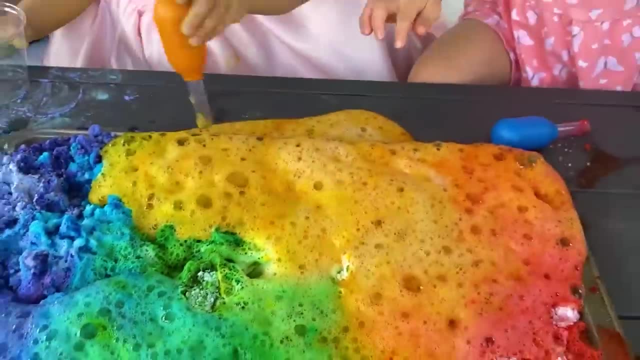 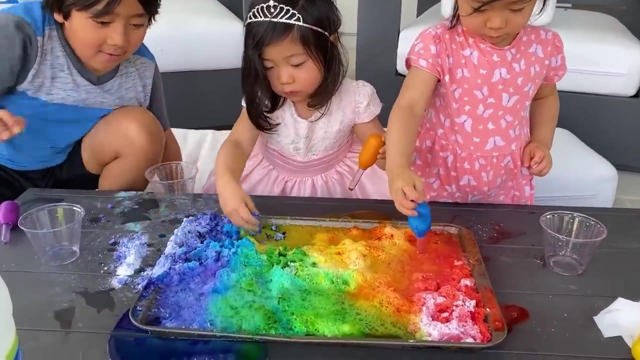 Yum, Yum, Yum, Yum, Yeah, Yum, Yum, Yum, Yeah, Yeah, Yeah, Cafe: Whoa, It looks delicious, Whoa, It looks so cool. That was fun, huh. 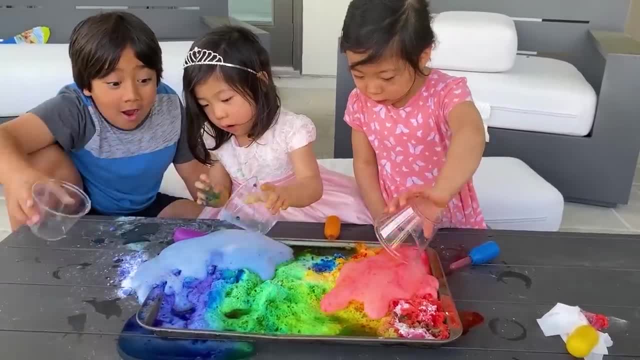 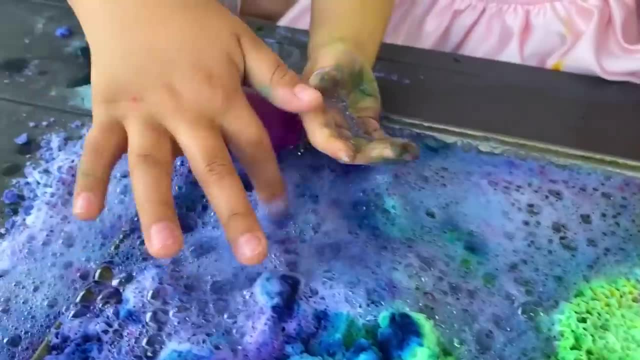 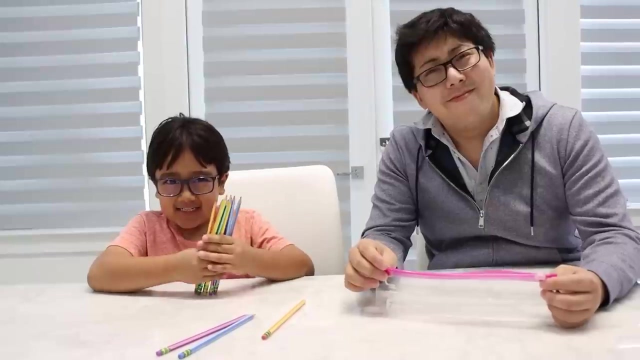 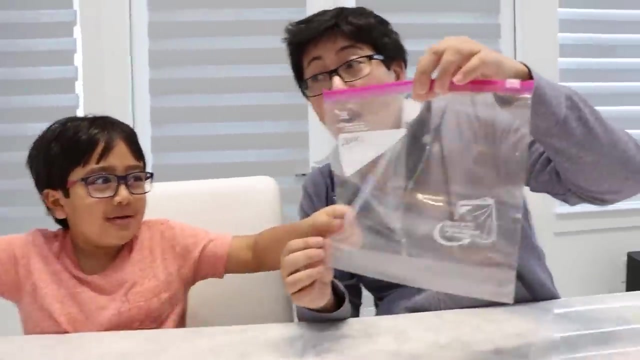 Yeah, Whoa, Can I touch it? Yeah, Whoa, That's super cool. Yeah, Hi guys, Today we're going to do a science experiment with pencils And we're going to poke these pencils through a Ziploc bag. 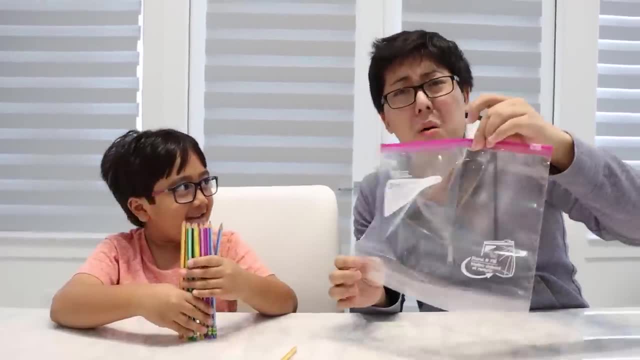 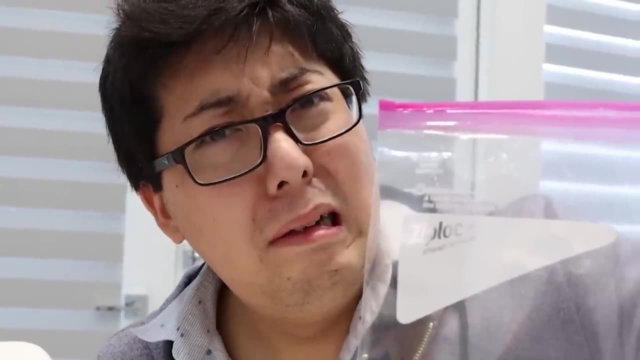 And the Ziploc bag will have water inside it. Whoa, whoa, Ryan. So that means all the water is going to leak through. Ryan. That's the chews bag, Uh-huh. First, let's put water inside the bag. 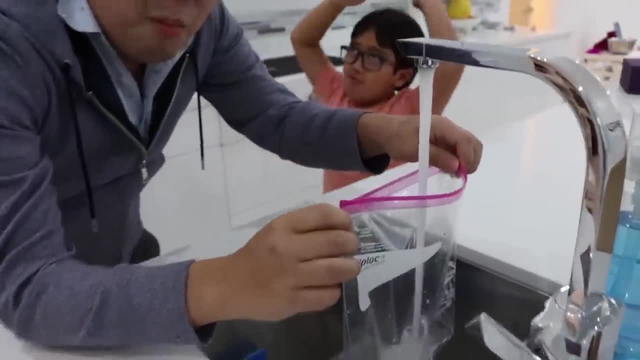 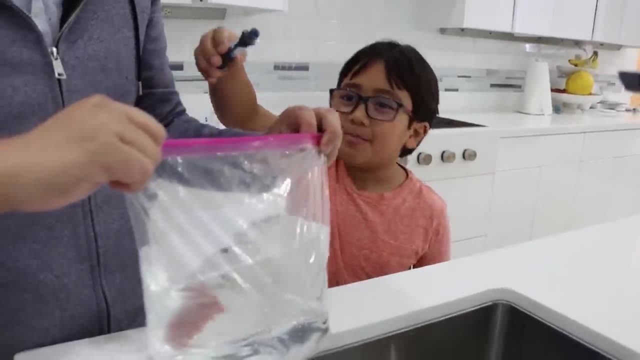 OK, Let's fill it up. Doo doo, doo doo- Hopefully Ryan's telling me the truth, because I don't want a big mess Now. we're going to put in food coloring. for fun, I'm going to use blue. 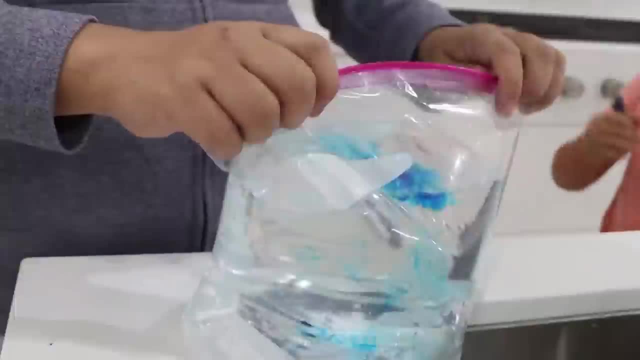 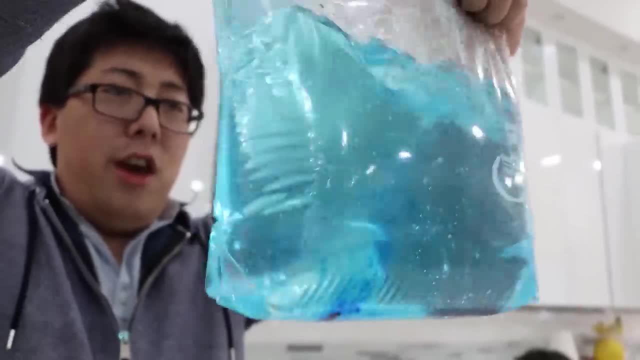 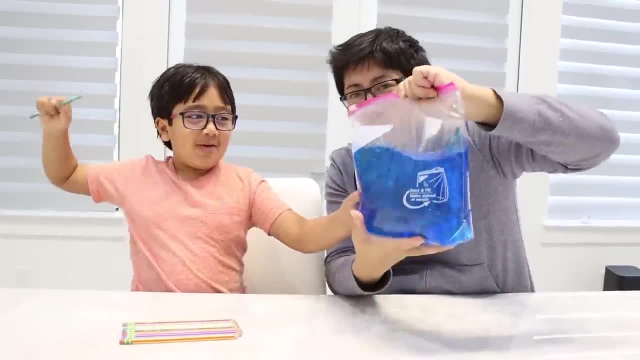 Don't forget to ask your grownup for help. All right, Here we go, We're going to poke it through. Three, two, one. Is it going to work? Yeah, It's not going to make a mess. Ah, it's poking through. 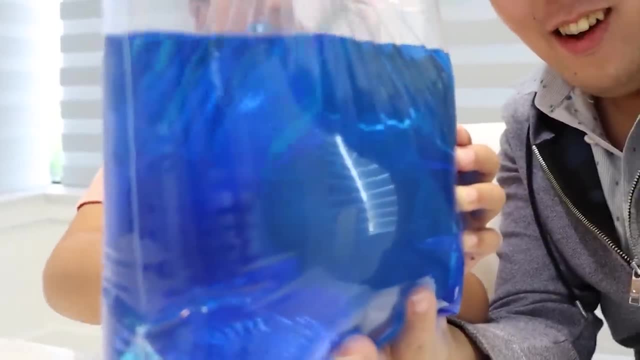 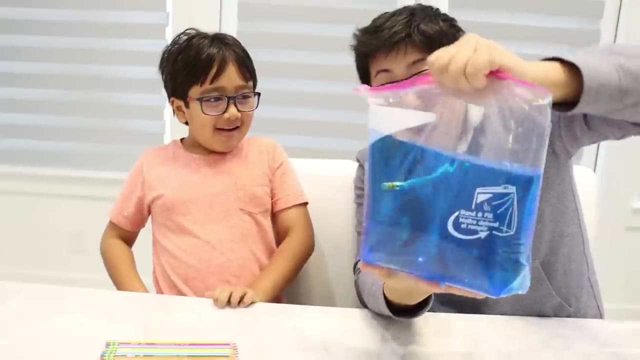 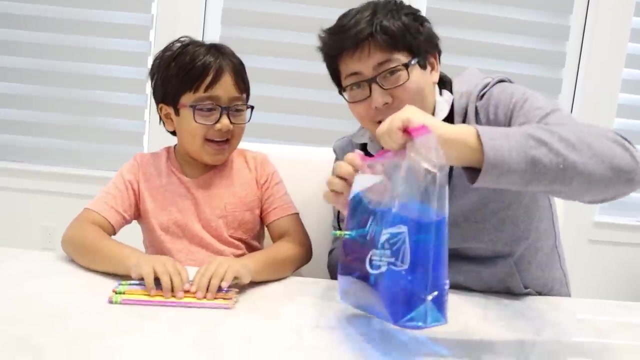 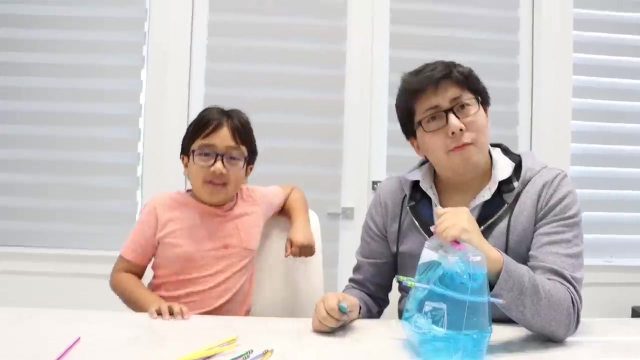 Whoa. Look the pencil's inside side. oh, no way, guys, there's no water coming out. what? why is it like this? how's it working? ryan, do more. ryan. okay, i'm gonna do a bunch of pencils. what about you? try, daddy, can i do it? all right, let's see, i'm gonna do it at the angle, does it? 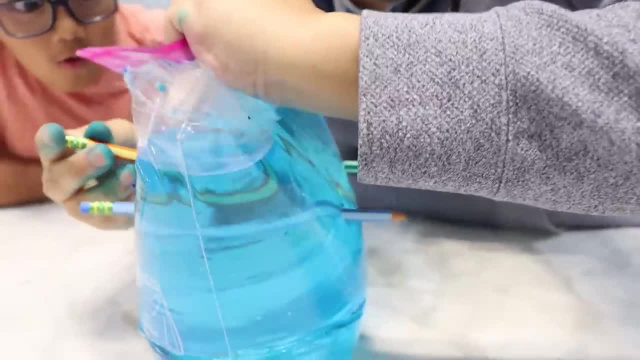 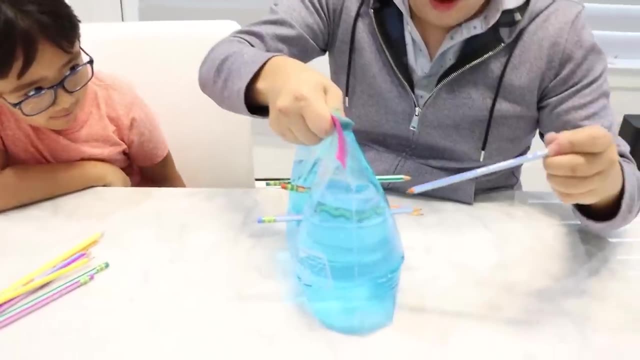 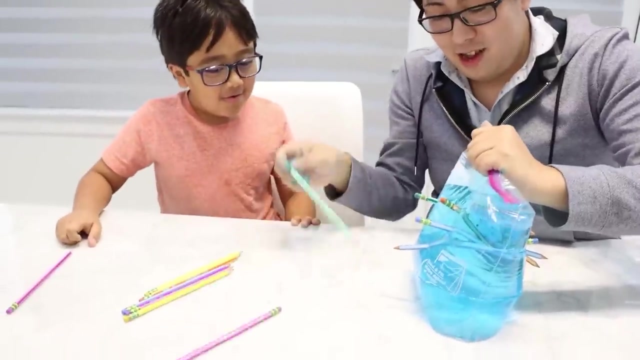 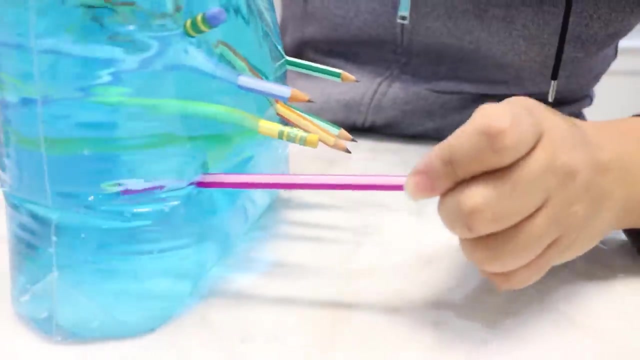 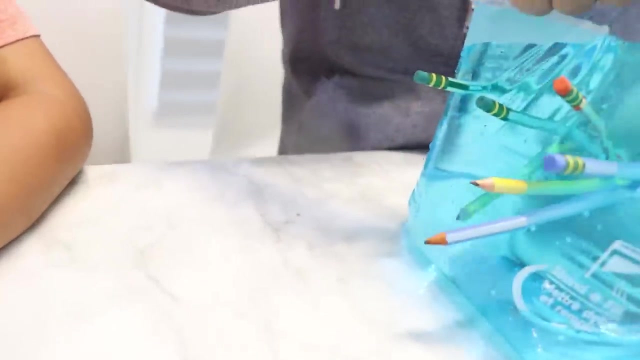 work, whoa, it works. whoa up down. all right, let me do it from opposite direction: up down, whoa, whoa, it's working. yeah, it is well, i'm gonna do more whoa, oh, whoa, pencils. all right, i'm gonna keep going. let's see if i can do all of them. 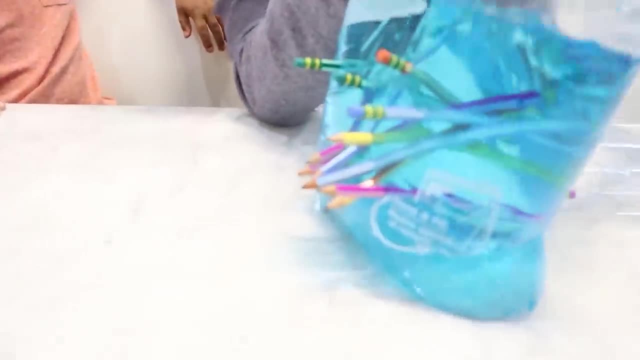 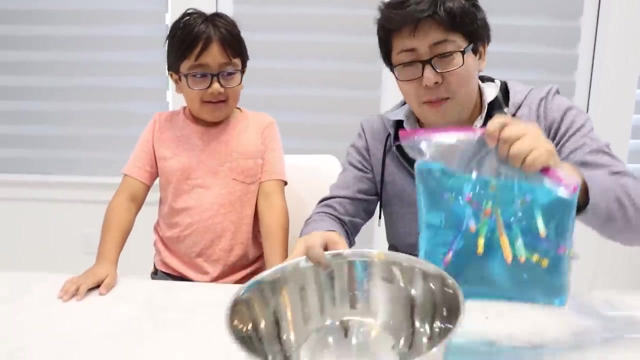 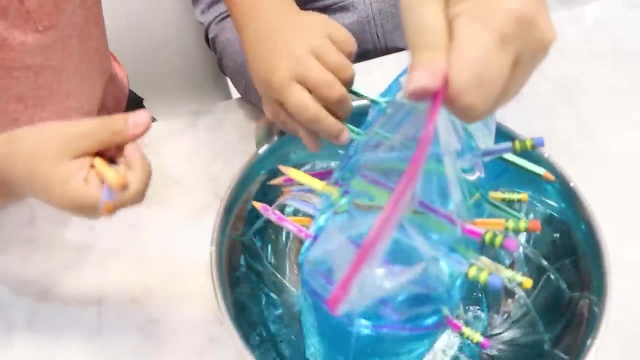 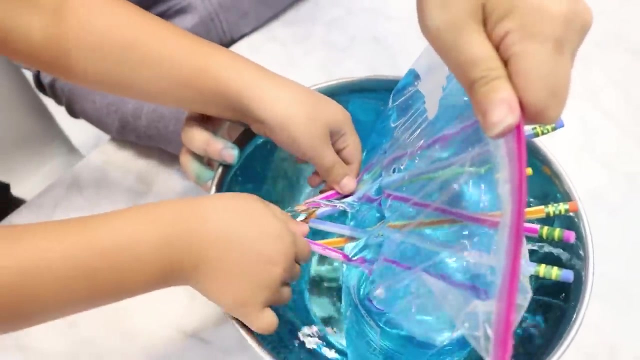 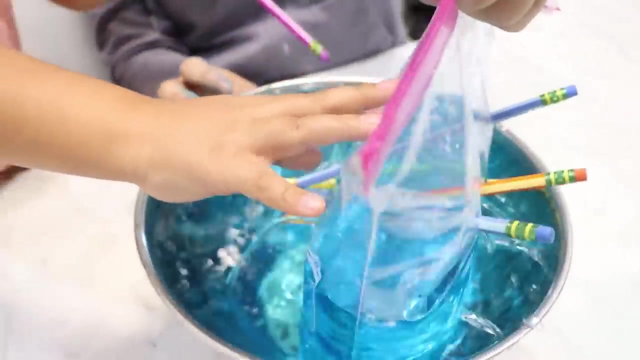 ah, i think i put too much daddy. what about we take out all the pencils and see what happens? oh, good idea, just in case, let's put in the ball right. all right, see what happens. oh, what's coming up. there's so much water, water, waterfall, water- those whoa look at that. well, there's so much water coming out- a shower. 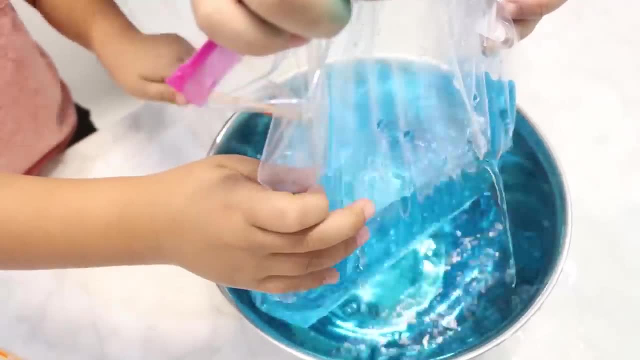 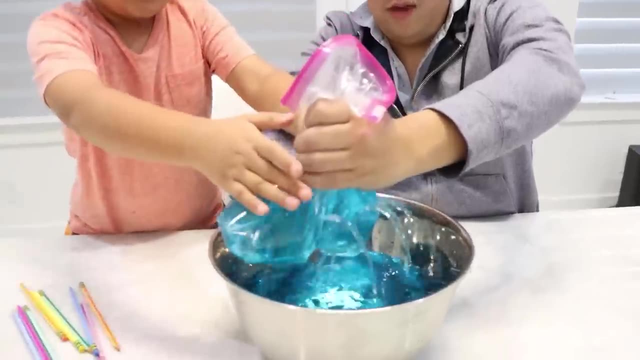 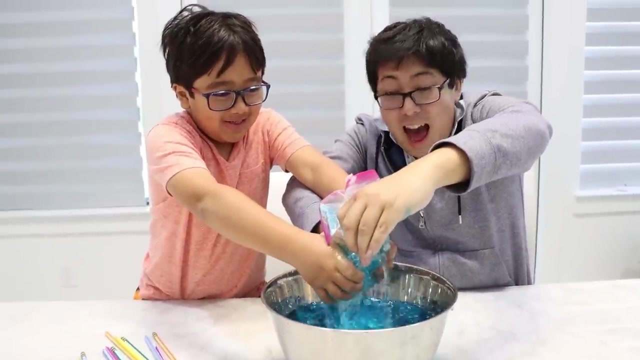 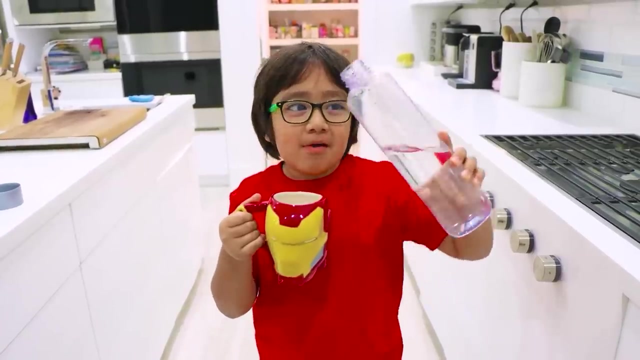 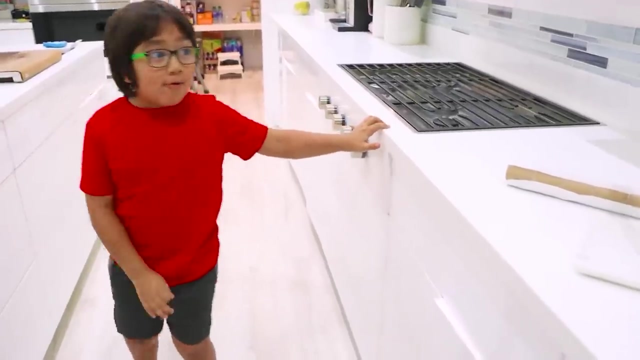 it's a waterfall of water. there's so much squeeze. ah, a refreshing cup of water. oh, no water spilled on the floor. i need paper towels. oh, there's no more paper towels. let's go ask mommy. mommy, i ran out of paper towels. i'm gonna have to ask momma. 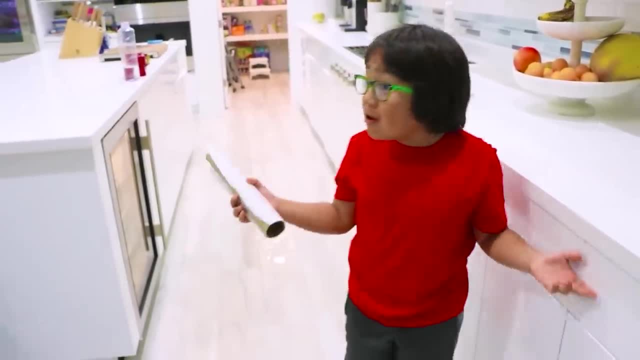 momma, i ran out of paper towels. let's go ask mommy. momma, i ran out of paper towels. let's go ask mommy, I ran out of paper towels. do you have any more? Ryan, Ryan, I have so many. is this what you need? 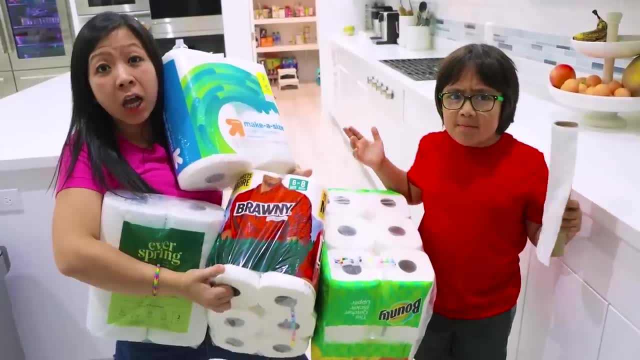 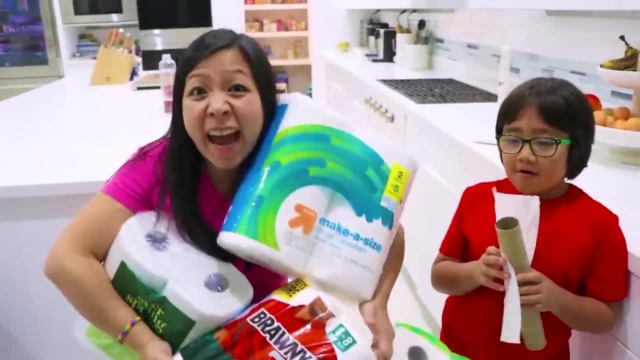 Yeah, but mommy, which one is the most absorbent? Good question, Ryan. Let's clean up that mess over there and do an experiment to find out. So we're gonna test out all of these different brand paper towels and we're gonna see. 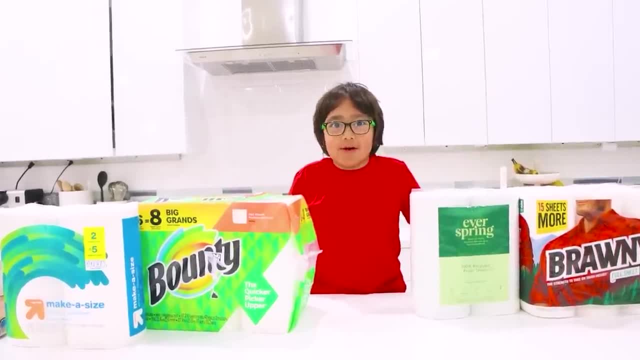 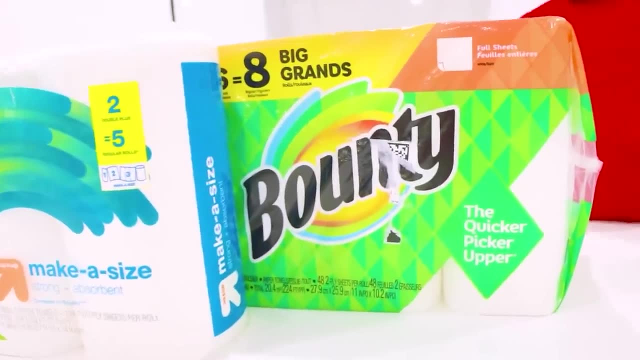 which one's the most strong and most absorbent. We got this Target brand here that says make a size. it says strong and absorbent. The Bounty brand: it also says the quicker picker upper, so it's supposed to be really quick. 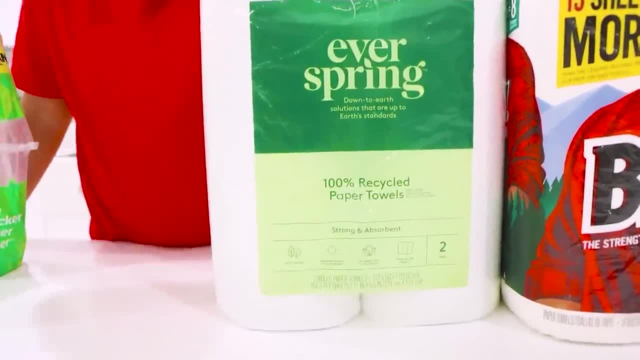 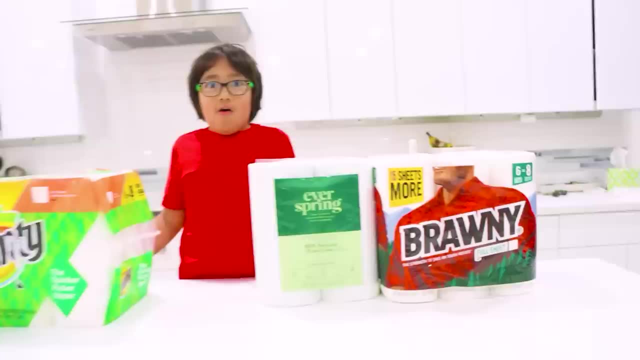 And this is the Recycle brand and also it says strong and absorbent And a Bronte brand that also says the strength to take on tough greases. Out of all of these, which one, Ryan, do you think is the most strong and most absorbent? 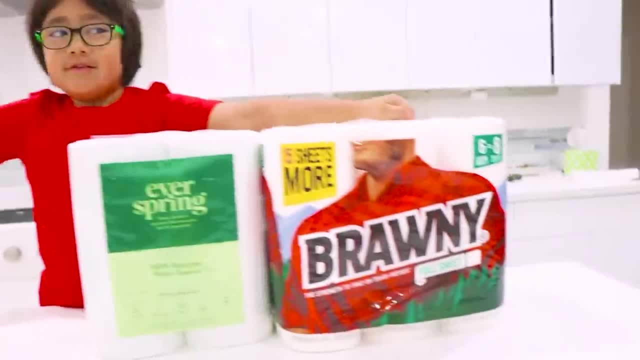 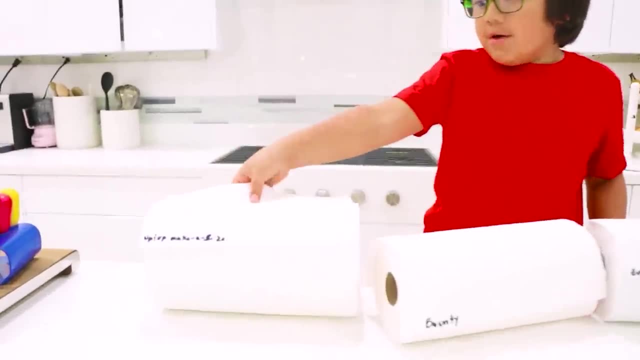 This one or this one? Oh really, The Bounty or the Bronte? All right, let's test it out. Yeah, So now we took out the wrapper and we labeled them. So first we have the up and up And look, it looks a little bit different. 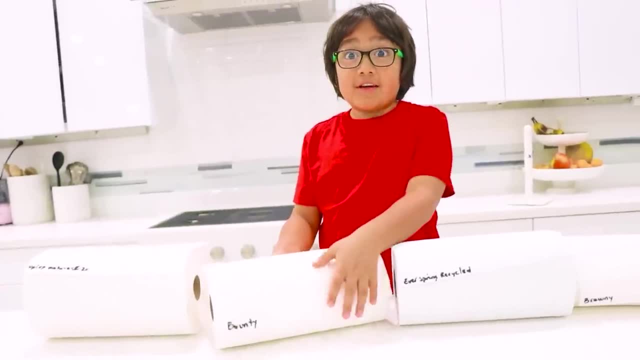 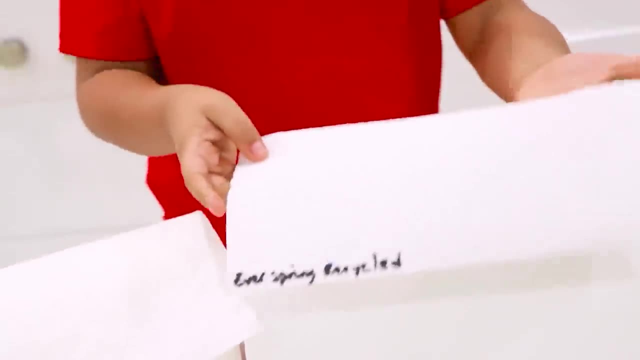 cause, like the lines and how it looks, And we got the one that I think is gonna win too the Bounty. We have the Recycle one And, look, it looks a little bit different than the others, darker, And we got the Bronte one. 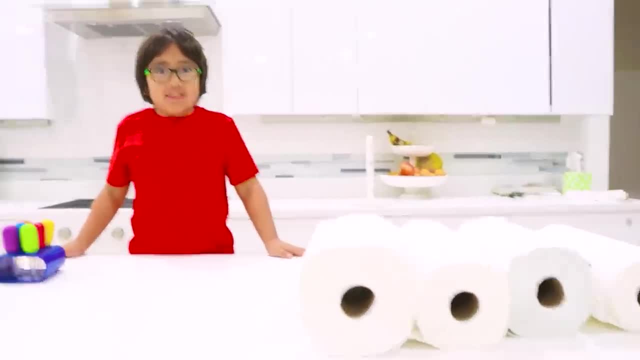 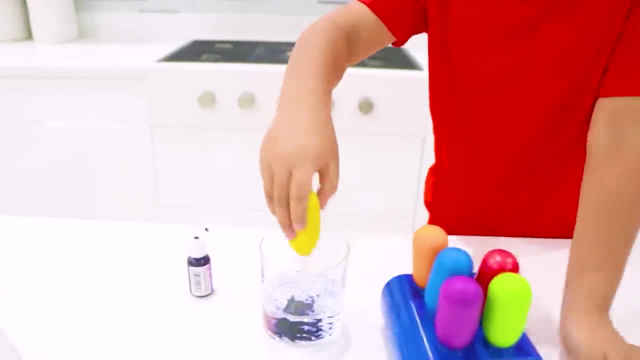 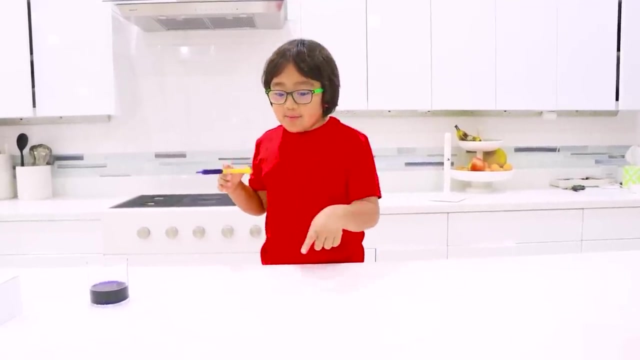 First I'm gonna test which paper towel is more absorbent. So first I'm gonna use purple. We can see better. Yeah, Okay, Perfect, Agitate, Agitate. So I'm gonna put the same amount of water on the table. 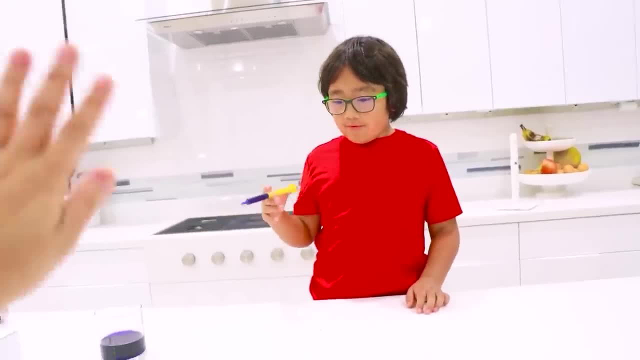 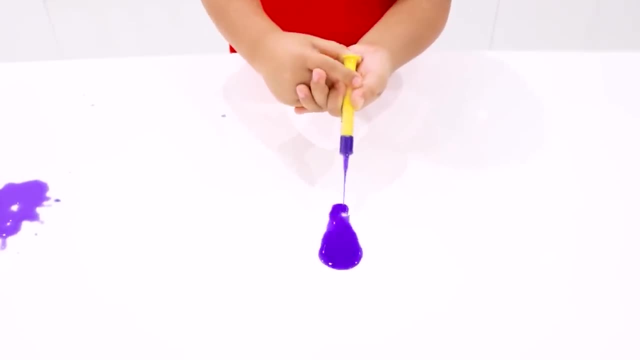 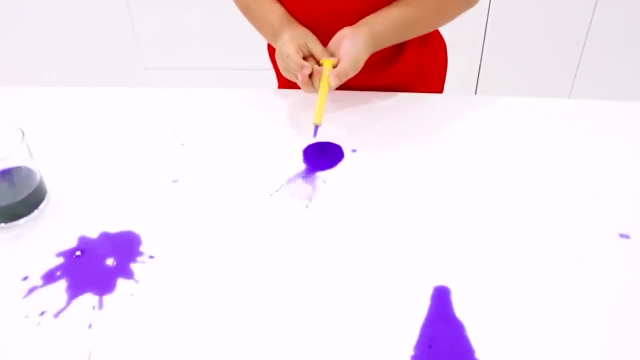 And don't forget to ask a grown up for help. Ryan has a grown up. Hi Do four different spots to test out four different paper towel brands. Mm-hmm, Sure Three, Four, Whoa. Now I'm gonna put each brand of paper towel on each spot. 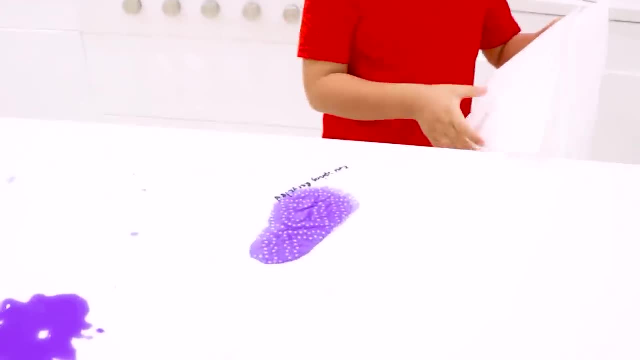 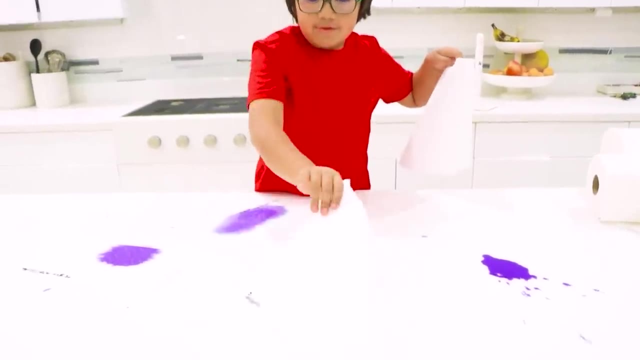 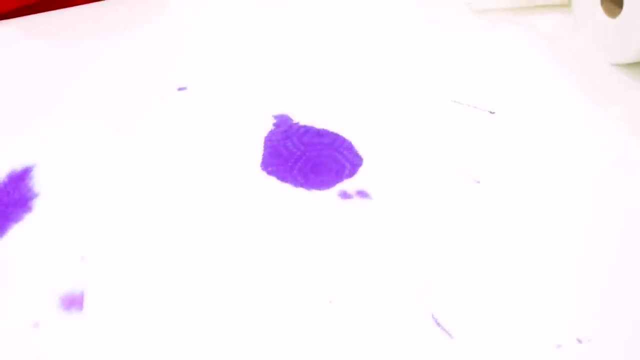 This is the Recycling, This is the Up and Up. This is Bounty And this is Bronte. We're gonna wait 60 seconds and we're gonna see which one absorbs the best. It's been 60 seconds. Let's see how they do. 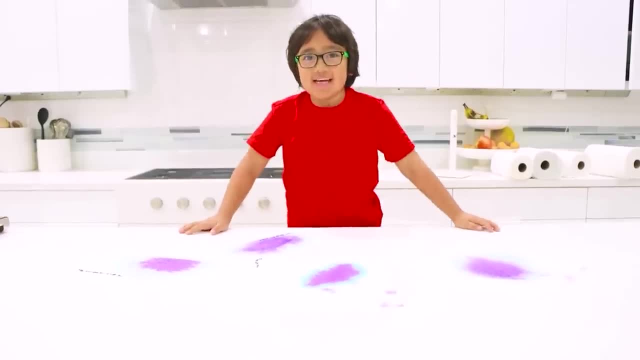 Whoa, This one is the Bronte. So that one's been pretty good. Yeah, Took away almost all of it. And this one is the Bounty one. Whoa, This one's pretty good too. Oh, I think this one is better. 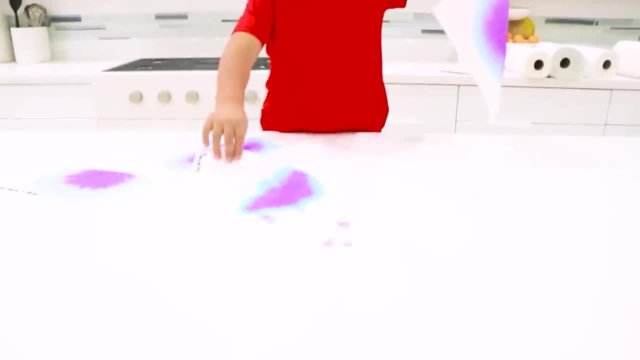 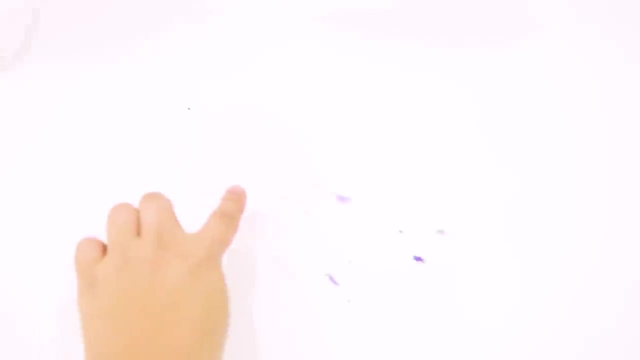 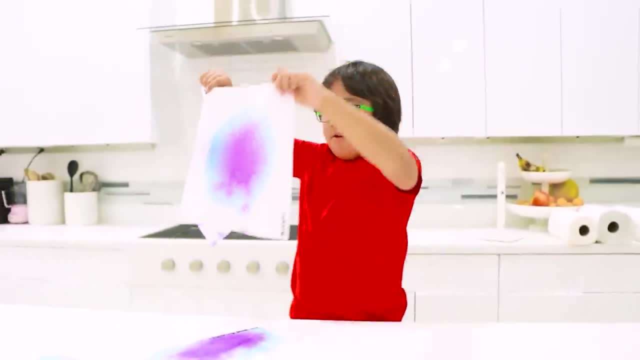 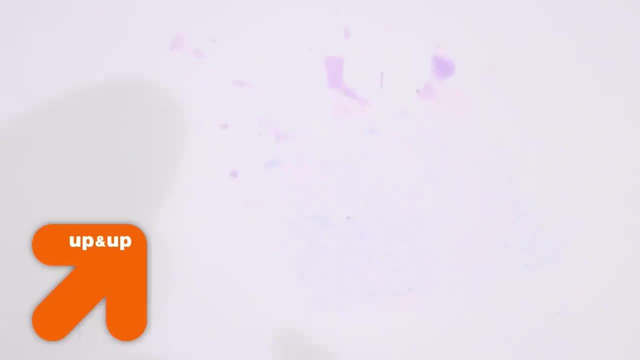 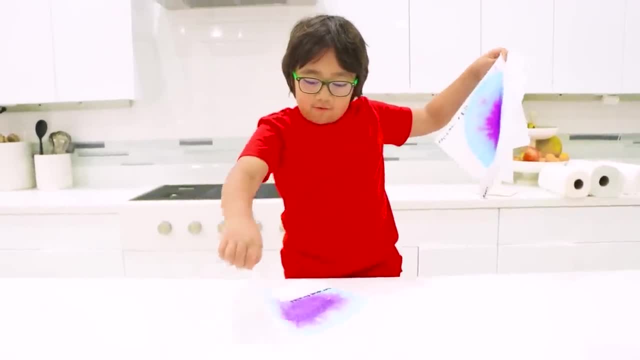 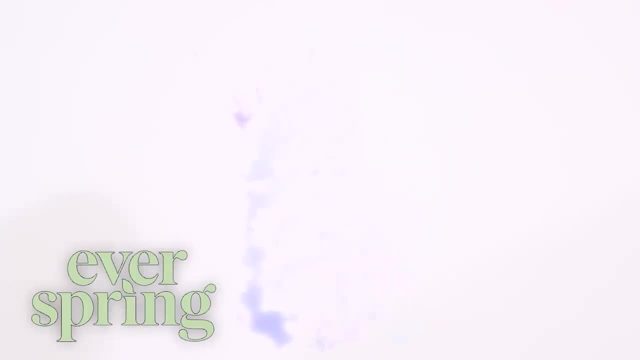 And this one is the recycle one. Oh, It's a little bit wet still. Oh yeah, The recycle one still left a lot of wetness. Out of all the four brands of paper towel, which one did you think Ryan is the most? 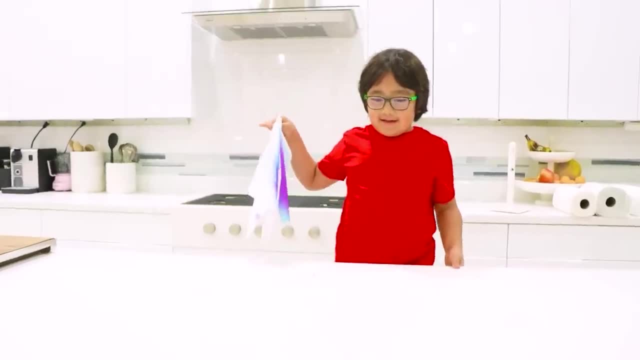 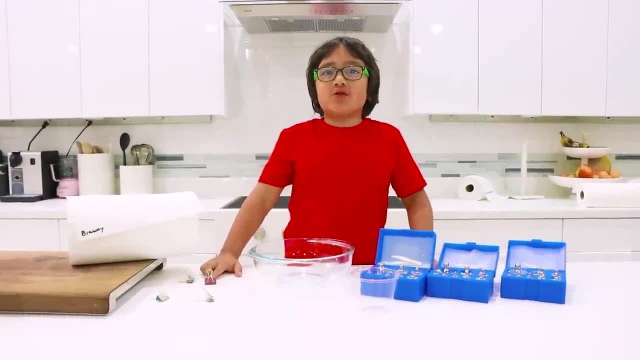 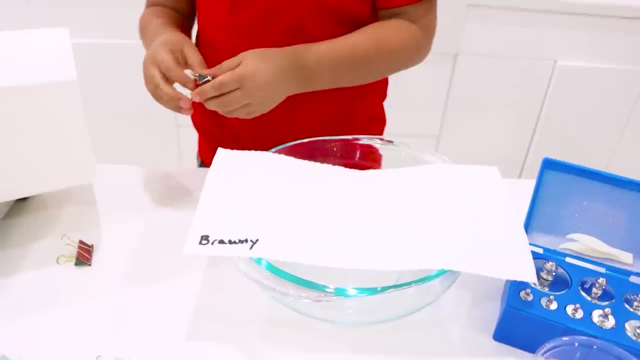 absorbent Bounty. Bounty is the winner for round one Bounty And it has a big bounty. Next we're gonna test out which paper towel is the strongest. So first we're gonna put Bronte on here And then we're going to clip it. 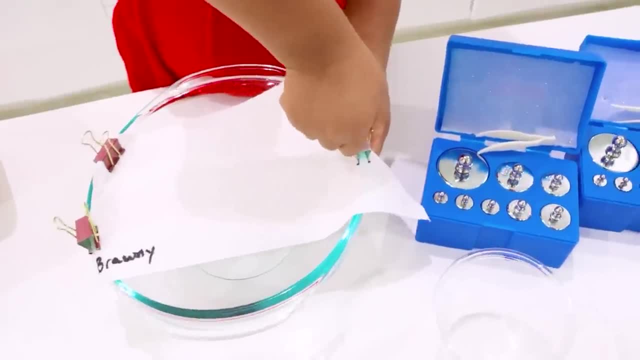 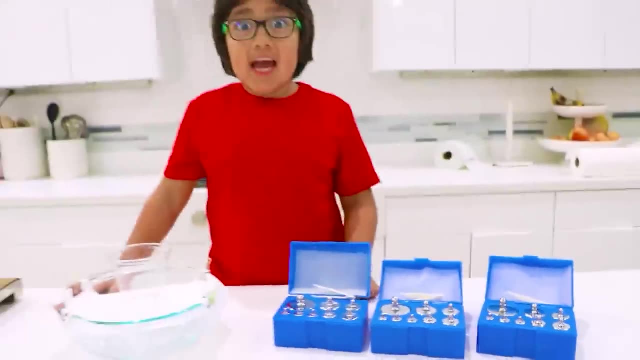 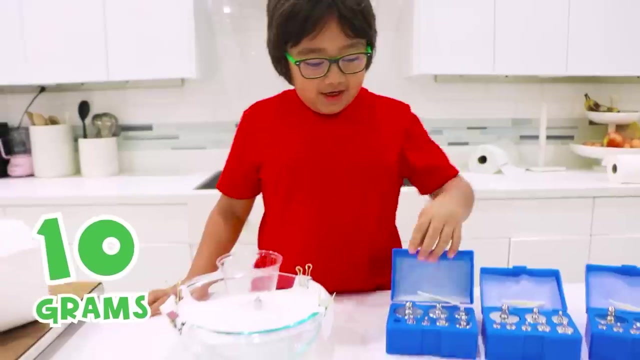 And the other side. Next we're gonna put on the cup And then we're gonna put on weights And we're gonna see how much weights it takes to break the towel. First, let's put the 10 weight. Okay, nothing happened. 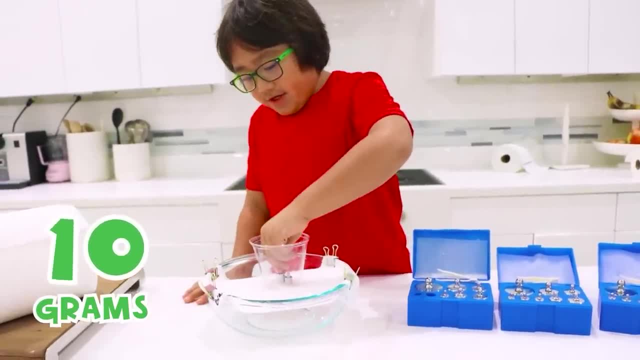 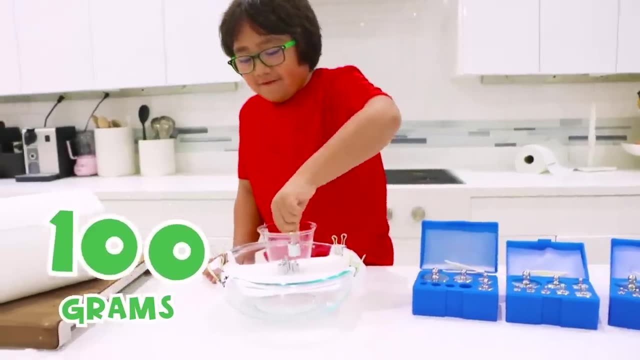 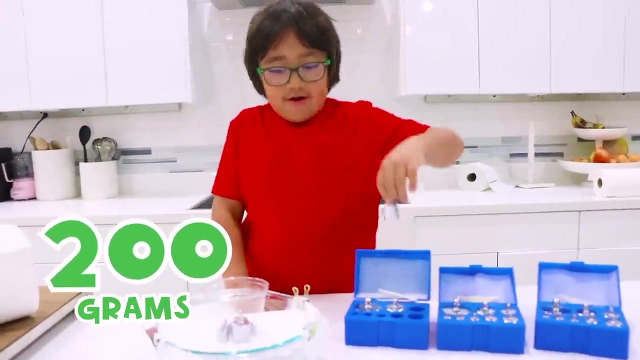 Then what about? we put the 20 weight, And then we're gonna put another 21.. And then 50.. Ooh, so far so good. And then 100.. Now we're gonna put another 100.. 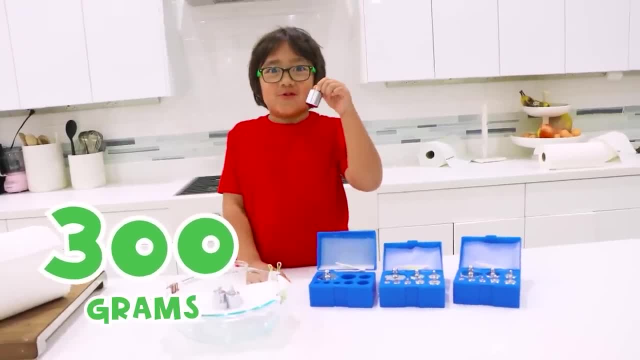 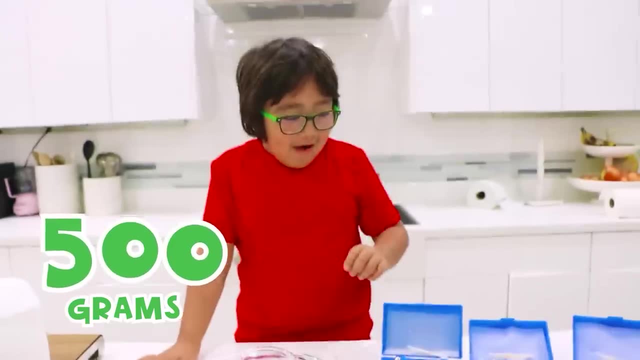 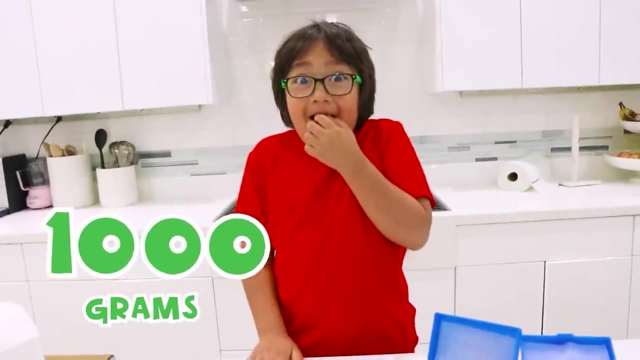 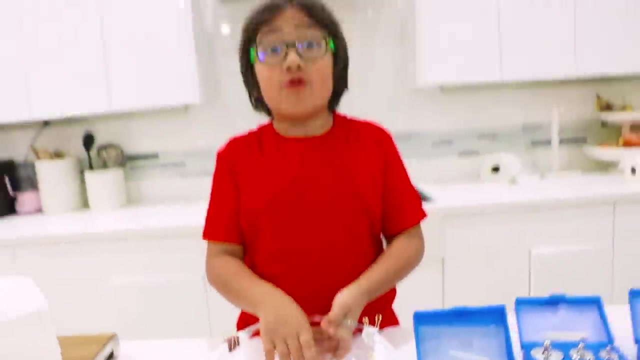 Okay, still good, And then the 200.. We're gonna have 500.. I think we have to put the 500 on. It's still still Dang. look guys, the paper towel broke And it took 1,000.. 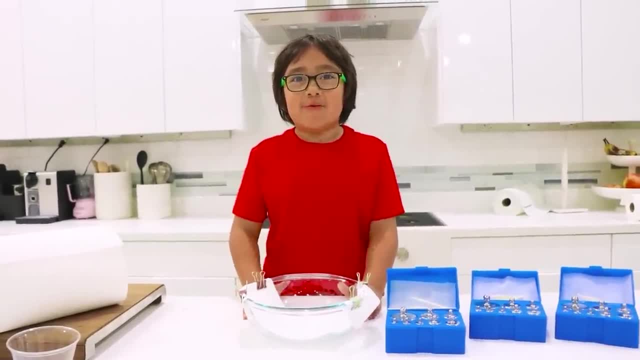 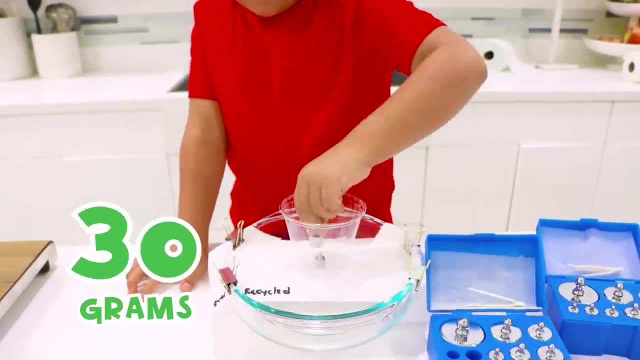 It took 1,000 grams to break the paper towel. Now let's do the other one. This is the recycle one. So first we're gonna put 10. And then 20. And then another 20.. 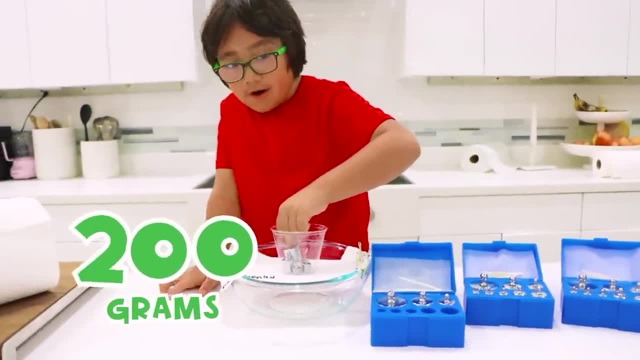 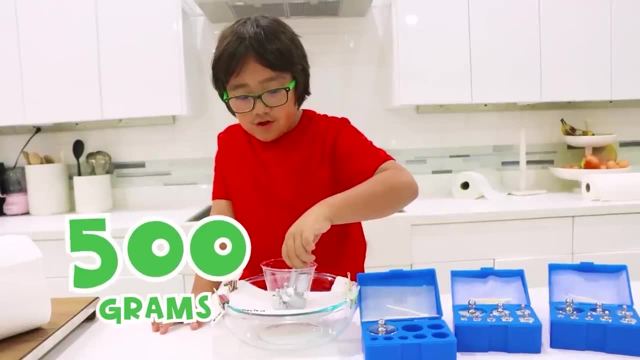 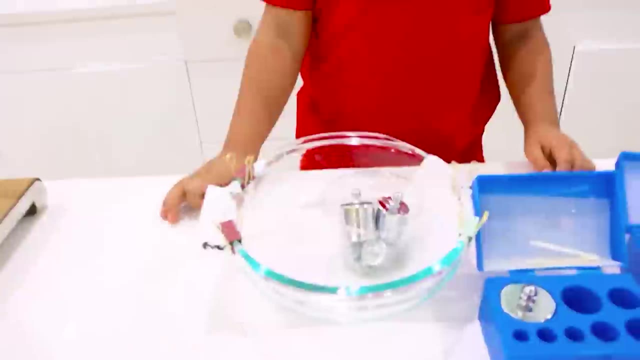 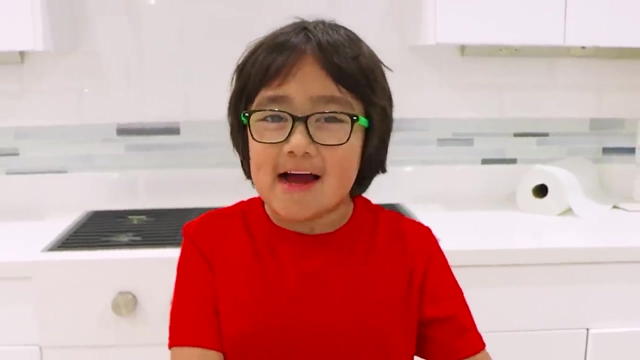 Okay, 50.. 100. Another 100. 200.. Whoa, Let's put another 200.. Whoa, it broke The recycle. one broke at 700 grams. Now let's do the next one. This one is the target up and up. 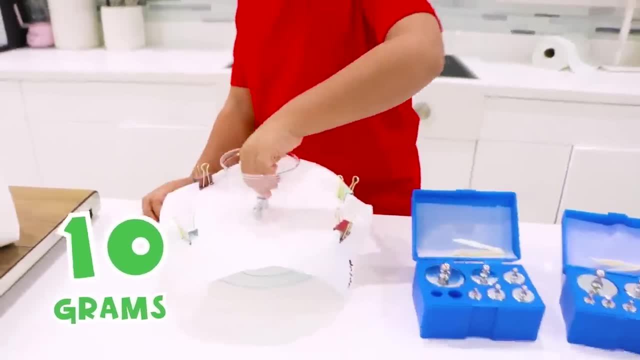 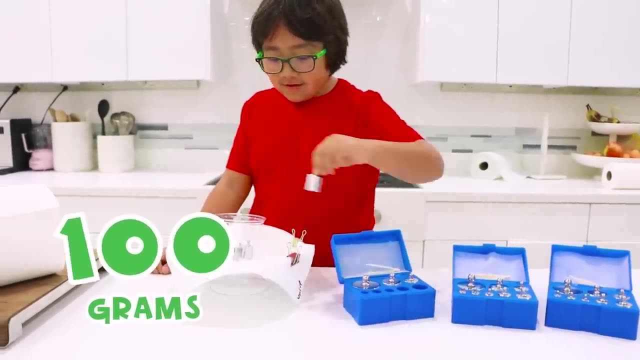 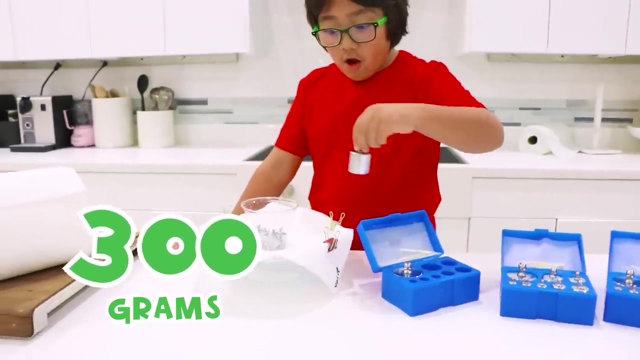 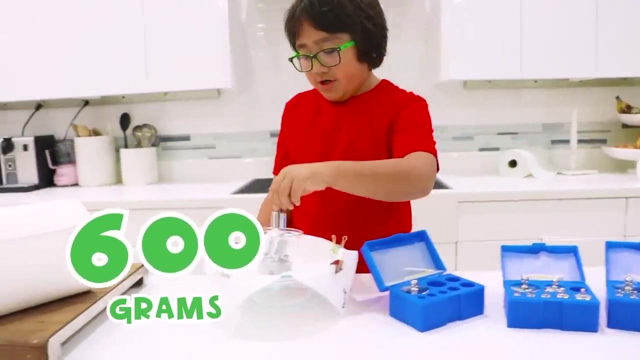 Now let's put the weight: 10. 20. Another 20. 50. 100. Another 100. 200., 200.. Okay, And then let's put another 100.. What about another 100?? 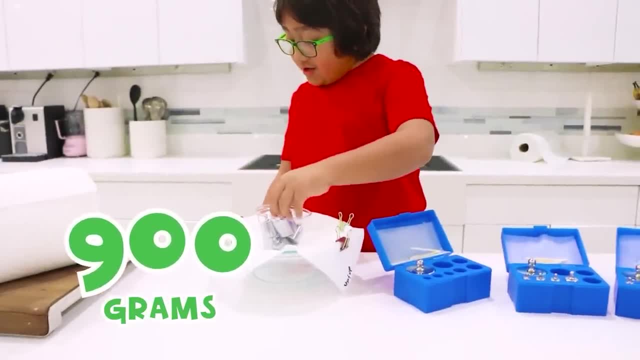 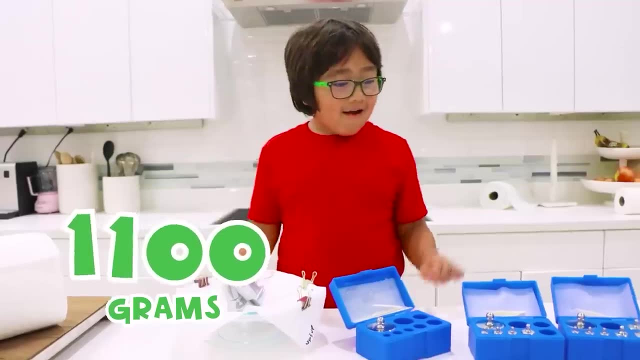 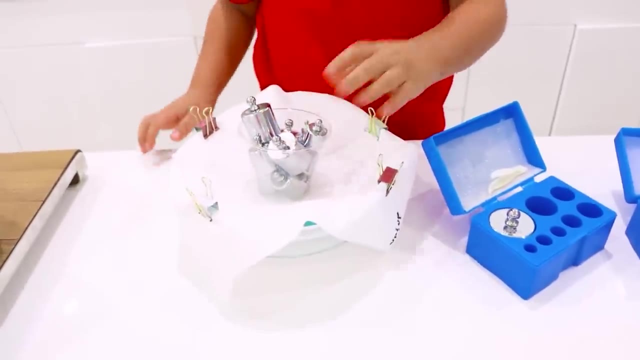 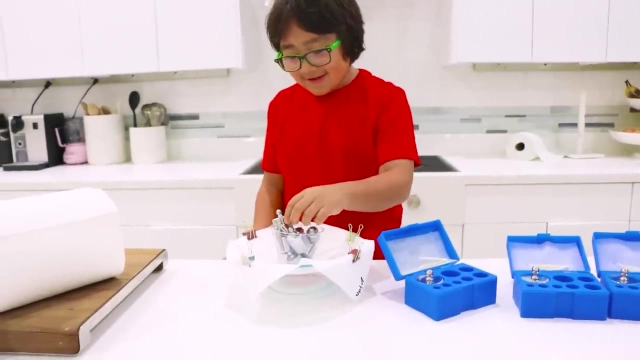 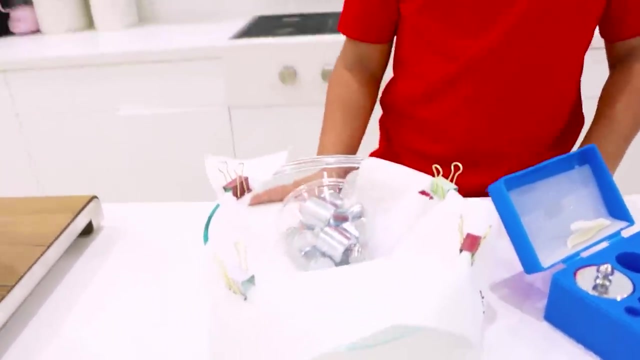 Whoa, this one's strong 200.. Whoa, 200.. What? Okay, I'm just gonna use all of these weights Let's see what it feels like. Let's see what it feels like when it breaks. this is really strong. Wow, target up and up. this is drop all the. 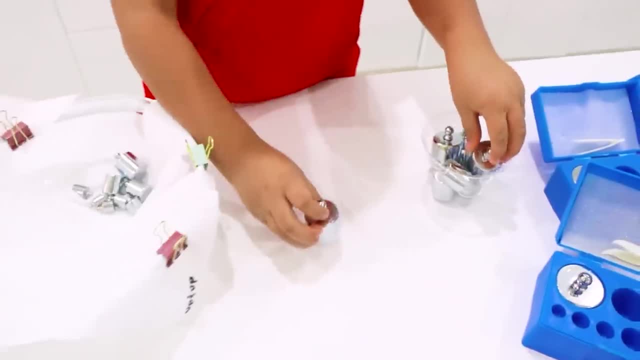 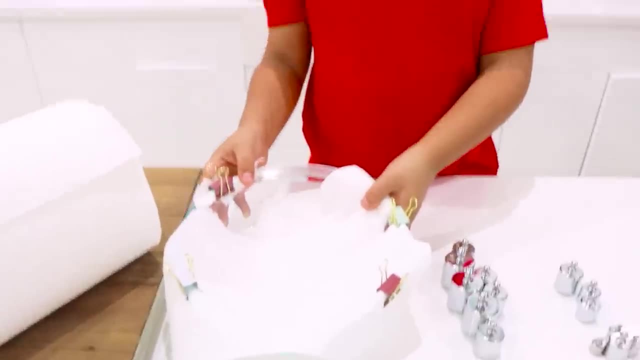 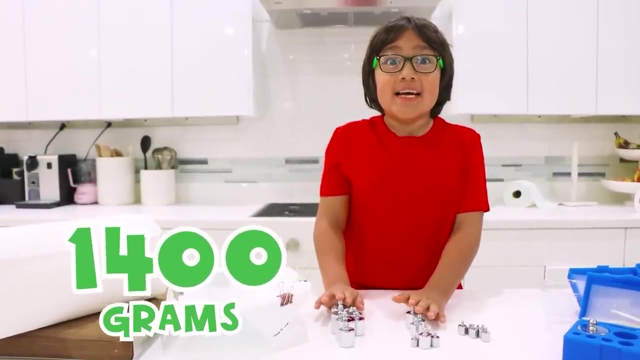 weight. look how much is left. oh, this is a lot of weight. take them out and we're gonna count them. so it's one, bro, but it's the strongest because it has one thousand four hundred grams. it's so strong I didn't know target up and up. 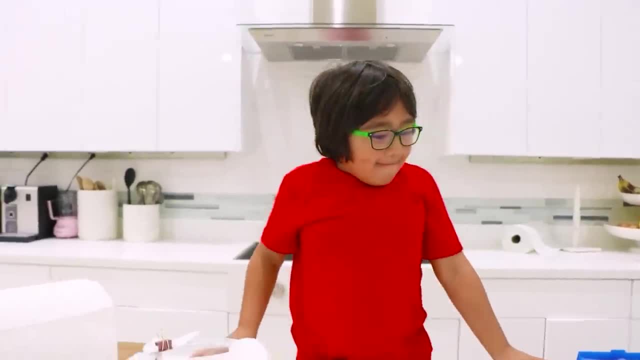 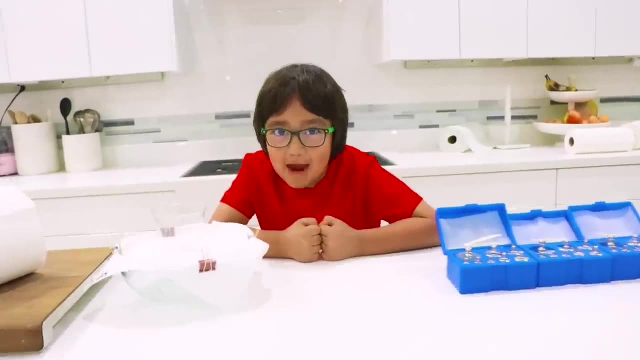 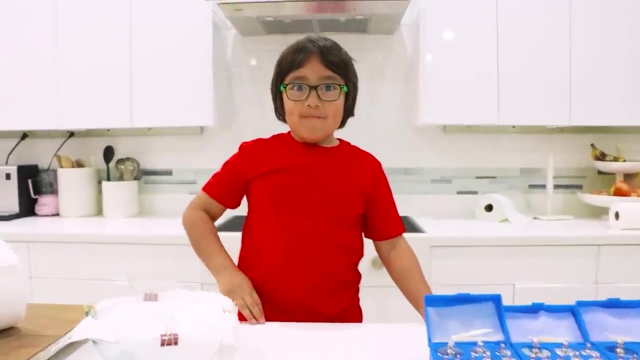 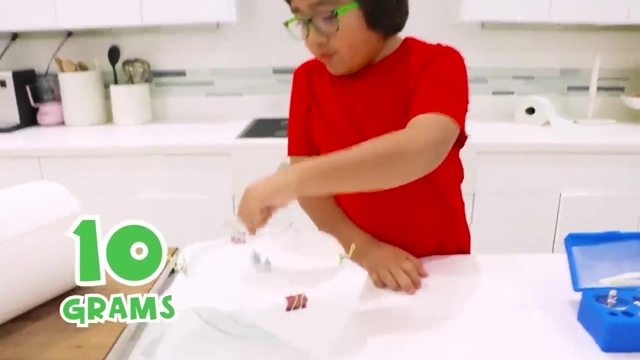 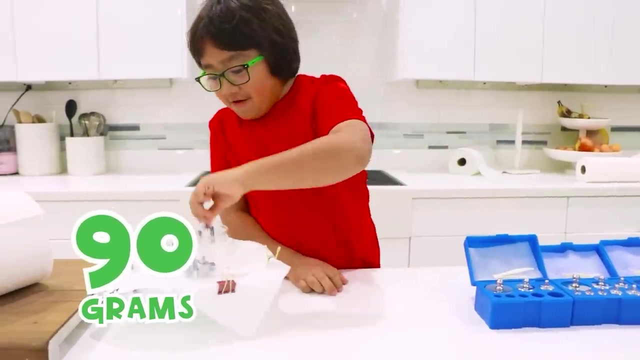 was so strong. okay, guys, we're gonna tackle the last one. let's see how it does. bounty- are you up for it? last one bounty? yeah, earlier we test that the bounty one was the most absorbent, but can it be the most strong? people find out. Kitchener has aiders. no. 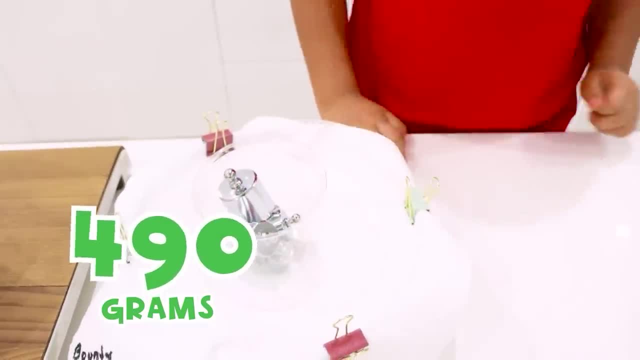 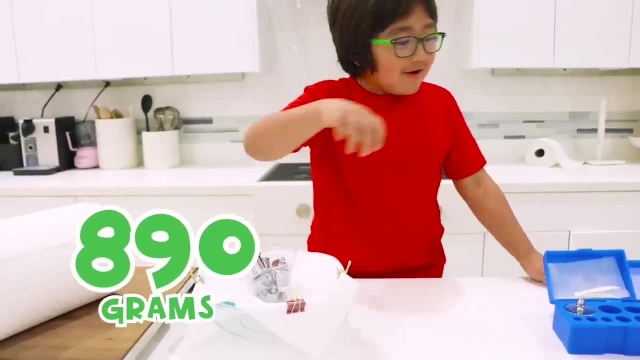 Oh, great bouncy. well, I'm hearing something. do you do you're doing great bounty? you did great bounty. you did great bounty, you did great bounty. do you're doing great? I'm hearing something. do you do your? You're doing great bounty. Wait, I'm hearing something. Do you hear that? 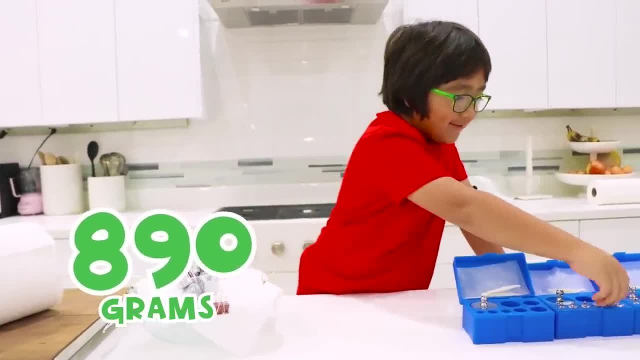 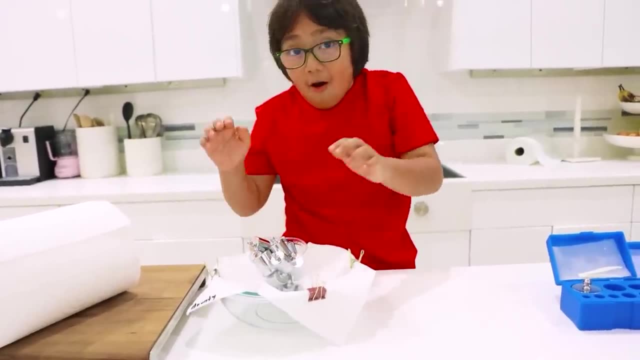 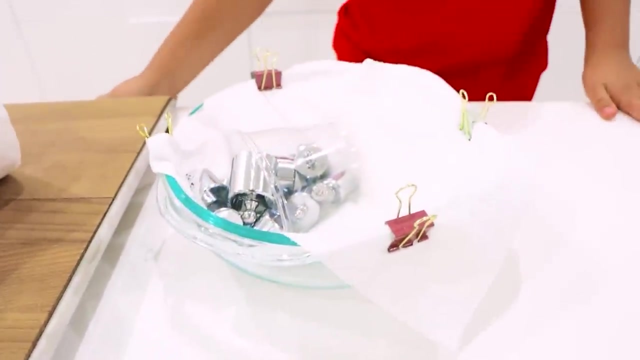 The rip. Yeah, Okay, 100.. 100.. This is more than one pound It broke. Okay, we're going to test to see how much Ryan put in. We're going to take it out and count them, Okay. 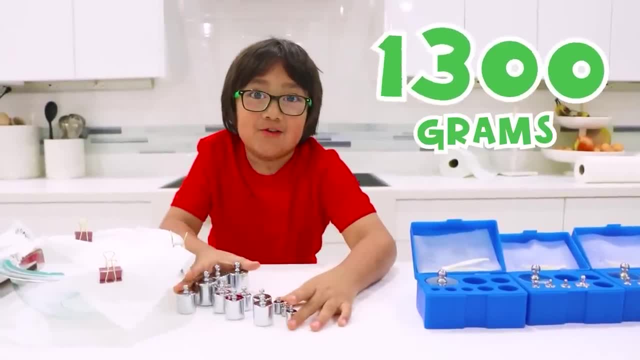 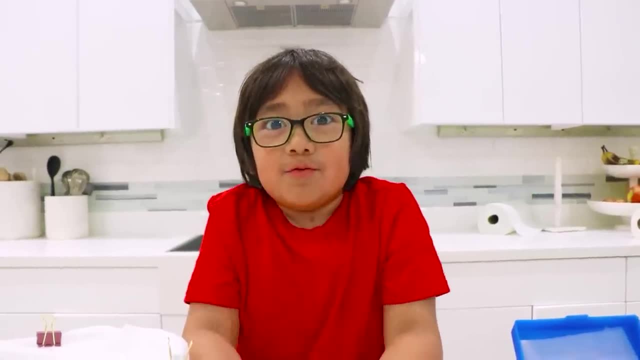 Okay, Ryan's counting right now. This is 1,300.. Wow, that's still pretty strong, Yeah, But it did not beat the Target Up and Up, That's true. Yeah, it's 100 less. My experiment Bounty was the most absorbent. 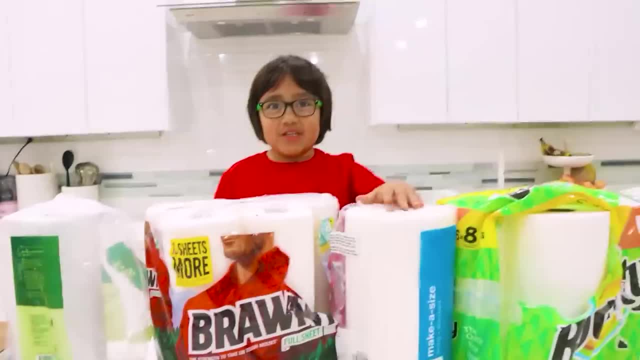 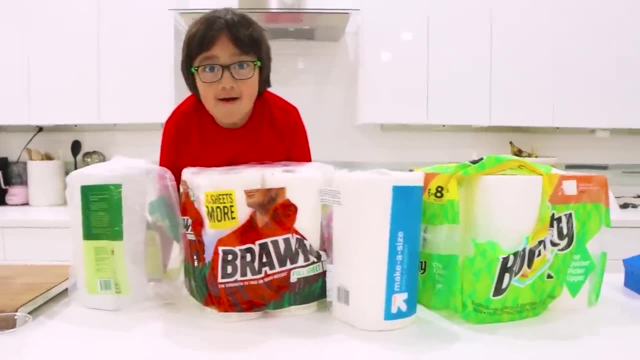 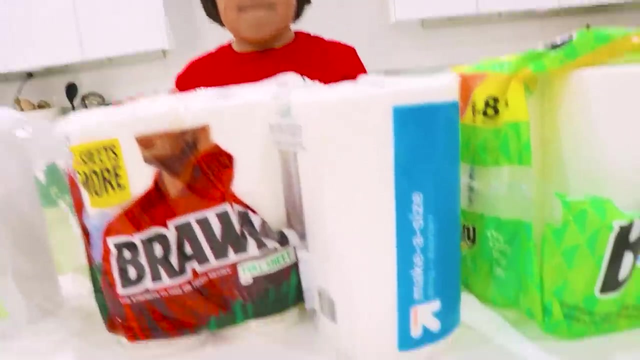 Absorb And the Target Up and Up was the strongest Pow, pow, pow Wow. So it'd be fun if you guys also test out different brands to see if Ryan was right and see if any other brand beats the Bounty or any other brand that is stronger than the Target Up and Up. 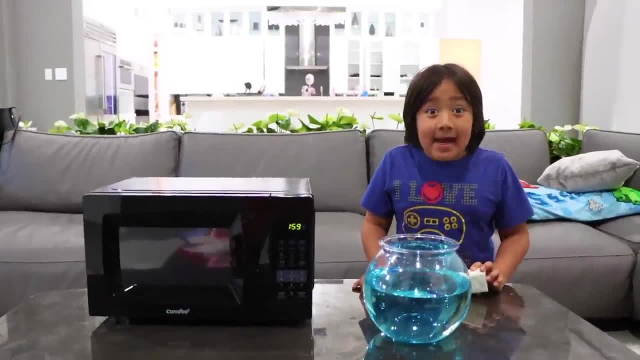 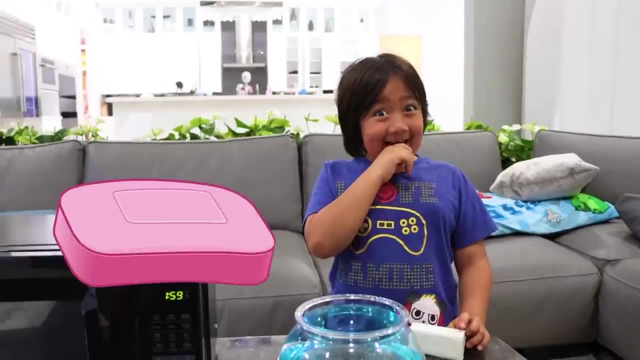 and let us know. Hi guys, Today I'm going to microwave a bar of ivory soap and see what happens. What do you think will happen, Ryan? Do you think it's going to melt? Do you think it's going to become bigger or smaller? 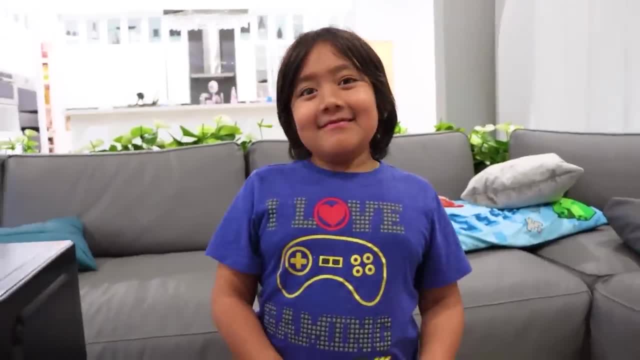 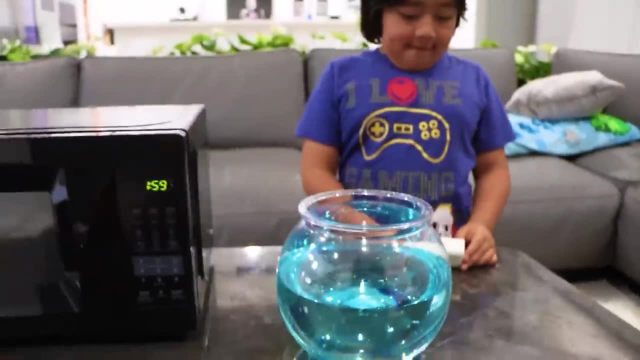 Disappear. What do you think? Disappear, Disappear. I guess we'll find out. So what I want you to do first is: I have water here and I want you to put the ivory soap into water, And first we're going to see if it's going to sink or float. okay, 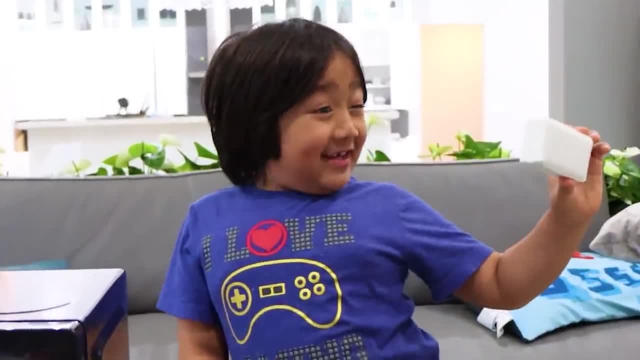 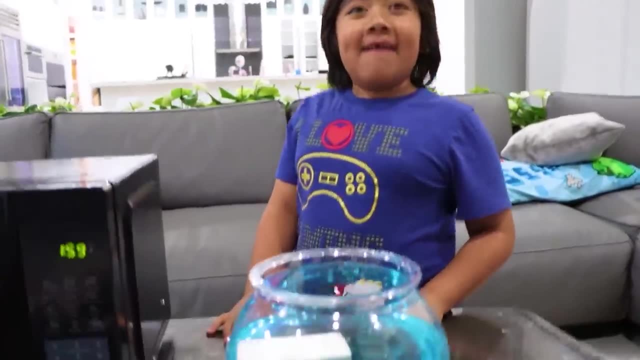 Okay, Do you think it's going to sink or float? Maybe, Maybe float. Okay, let's try it. It's floating. Yes, there it is. It actually floats in water. We don't have other bars of soap, but if you have a different brand, 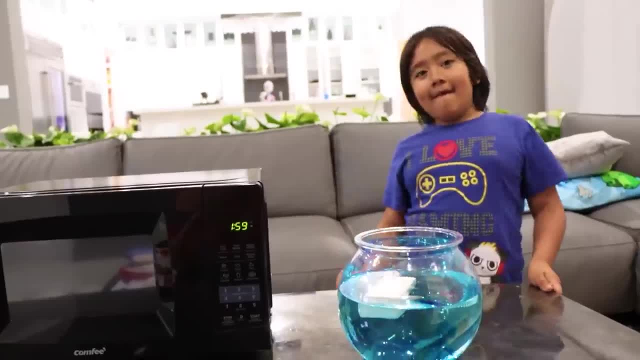 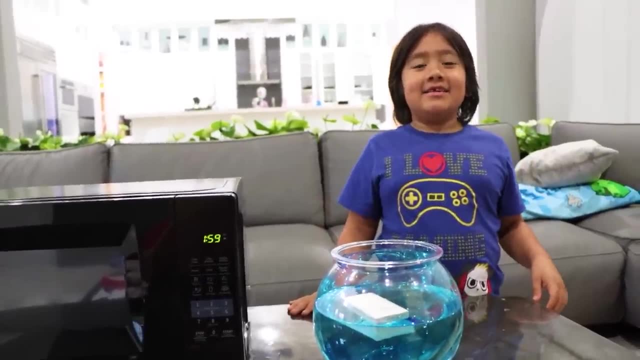 you can see if it also sinks or floats. These are ivory brands. So what does it mean when it floats on water More dense or less dense than water, Less dense? Good job, The bar of ivory soap floated because it's less dense than water. 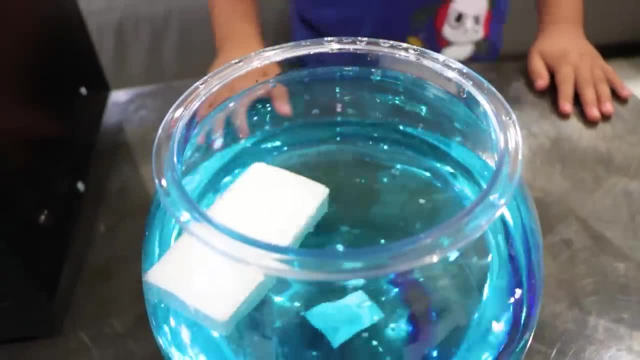 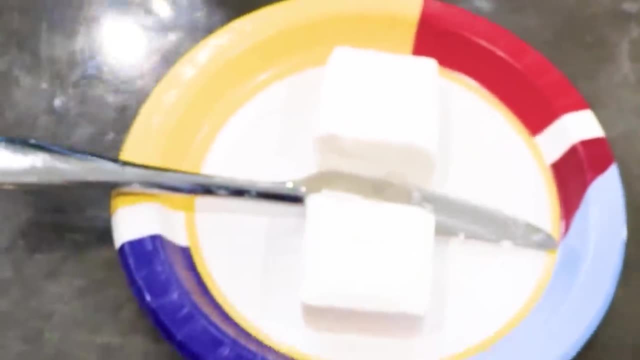 probably because there's lots of air holes. There's lots of air holes inside, okay, Yes, So we're actually going to cut it open and see: Okay, I'm going to cut the bar of soap in half. Okay, All right, so I cut it more. 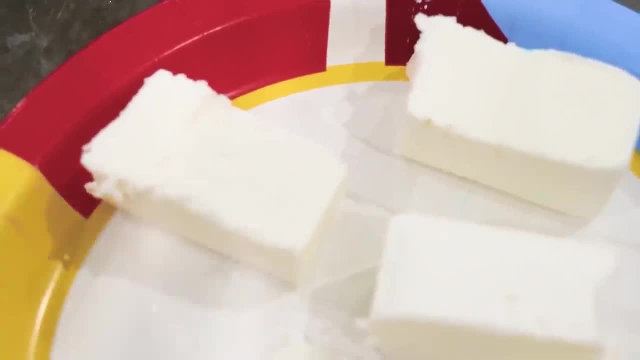 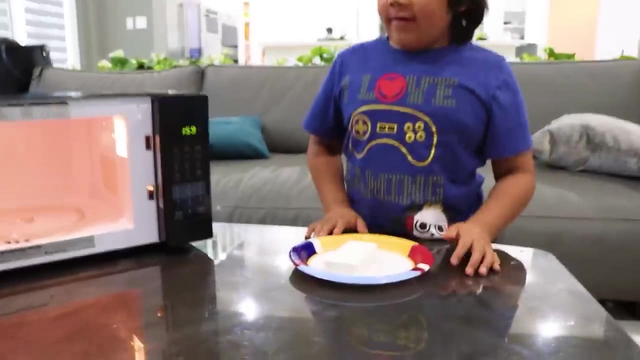 If you examine it very closely, it has like little holes of emptiness. I guess it's where all the air is. Are you ready to microwave it? Yeah, All right, we got our new ivory bar of soap here. Put it in the microwave, closing it. 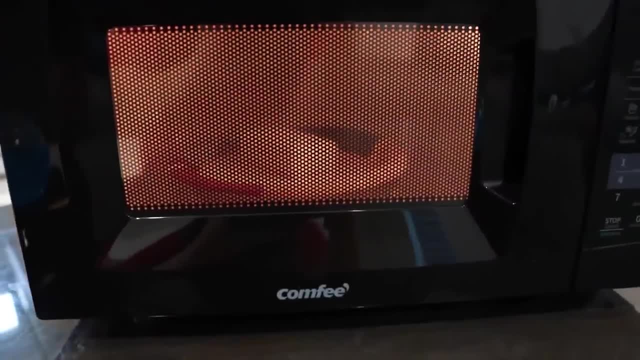 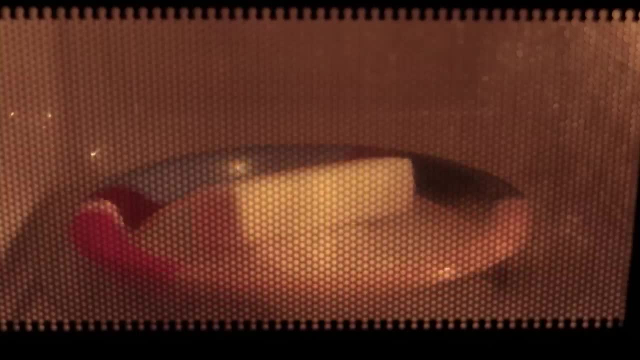 Start, Here we go, All right. So we're keeping our eyes on the bar of soap. Make sure you use a microwavable safe plate. Okay, let's see There's like stuff coming out of it. It's hard to see because of 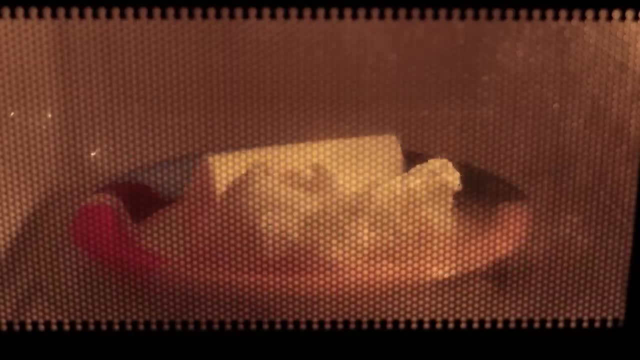 Do you see like the stuff? Oh, I do see. You guys see Whoa? Keep your eyes on it. Look guys, It's a little bit hard to see, but look, it's expanding. Yeah, it's expanding by a lot. 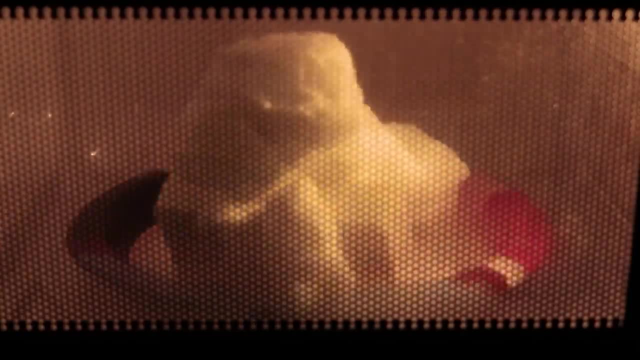 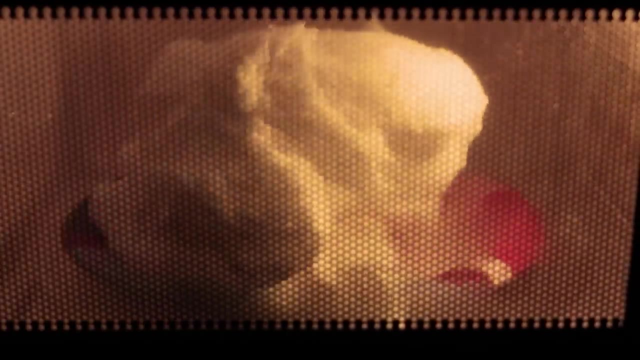 Whoa, I think it's melting the soap or something. Whoa guys, look That's big. Should we stop it? It's going to go all over the microwave. Whoa Guys, look at this. Whoa. 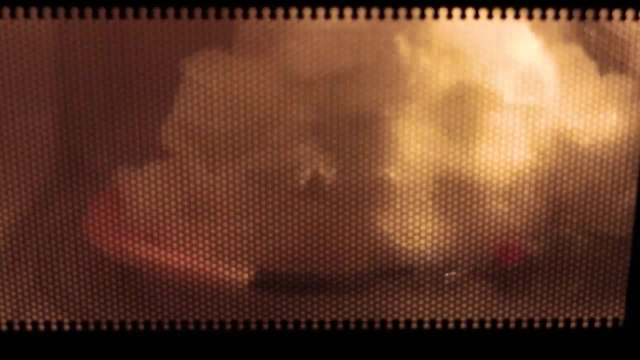 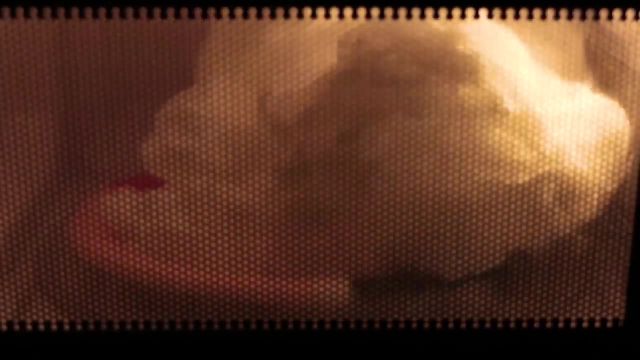 Whoa, it's filling up the whole microwave. Oh, Do you smell anything? A little bit Smells like soap. Yeah, Whoa, It looks fluffy like marshmallows. Okay, go on. Okay, Okay, Okay. 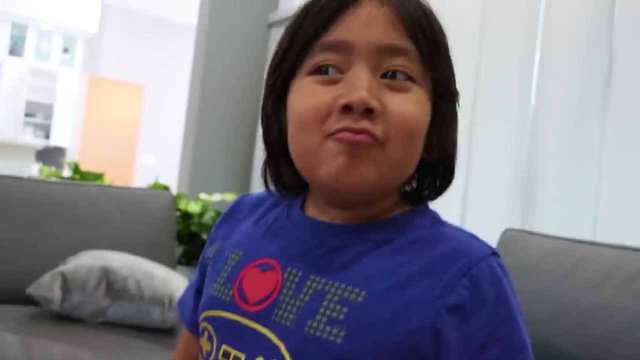 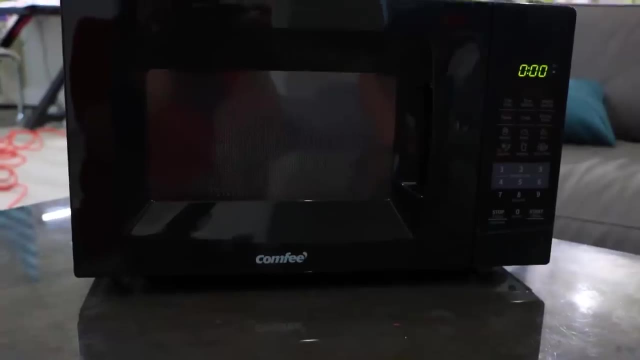 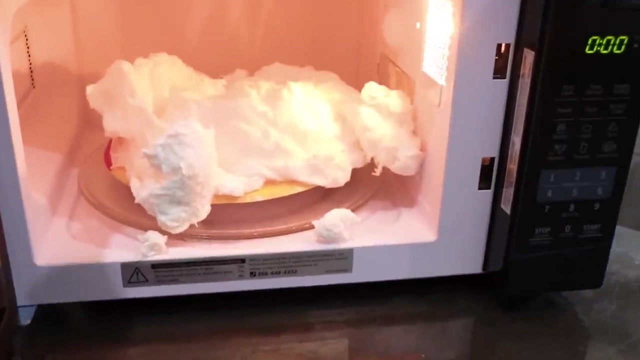 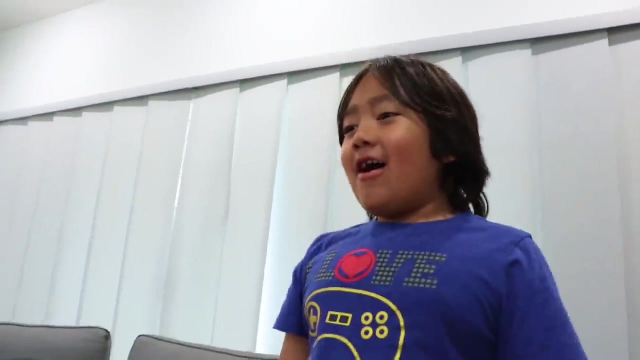 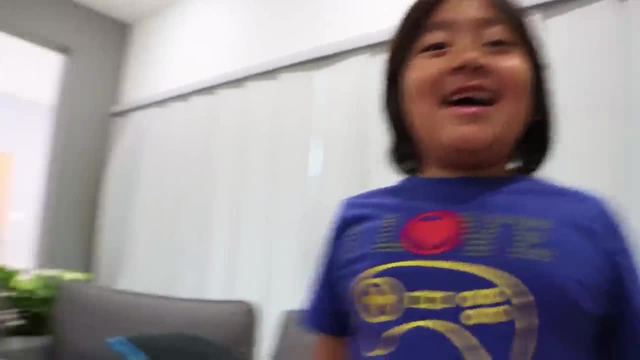 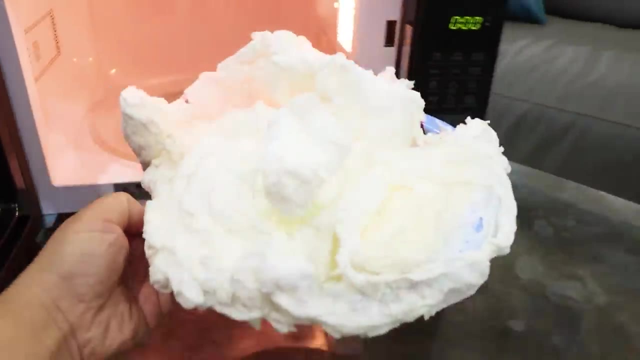 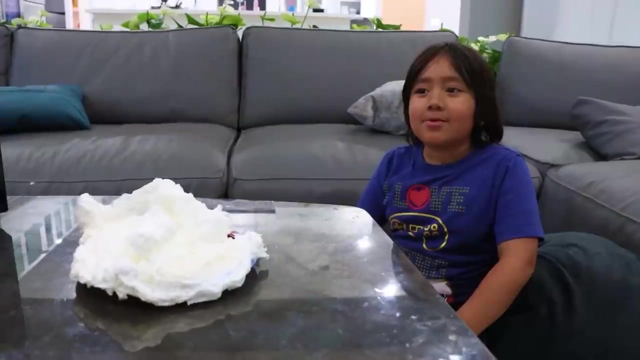 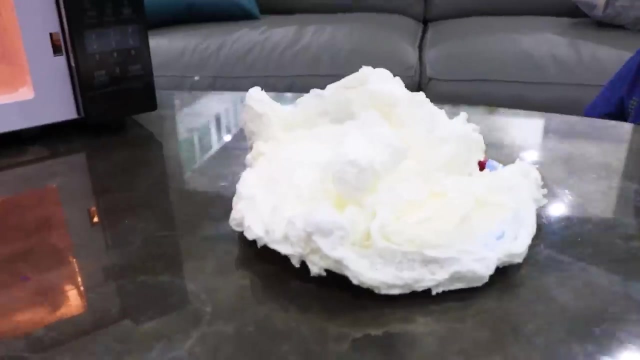 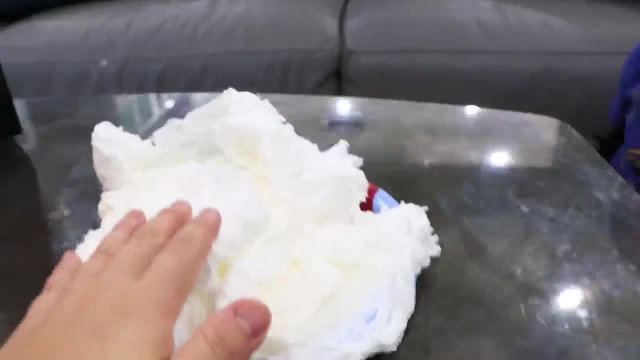 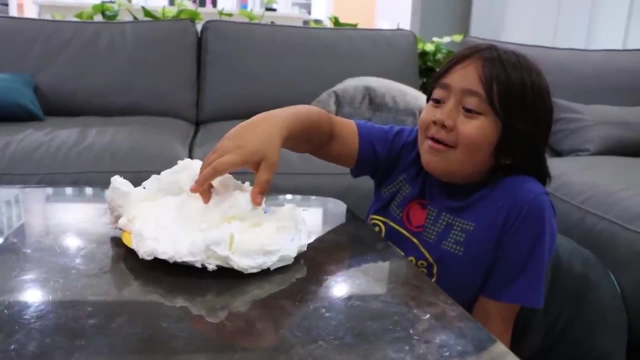 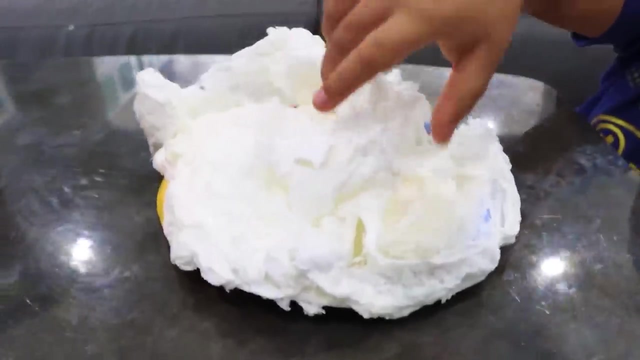 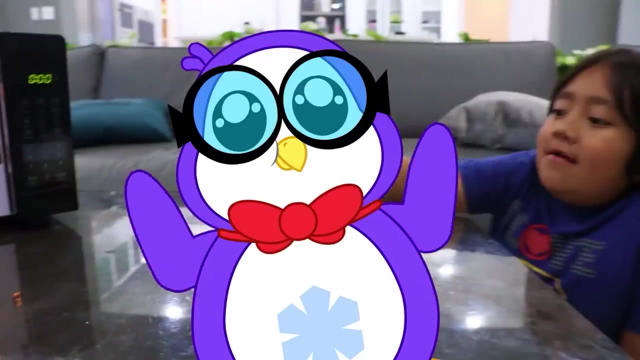 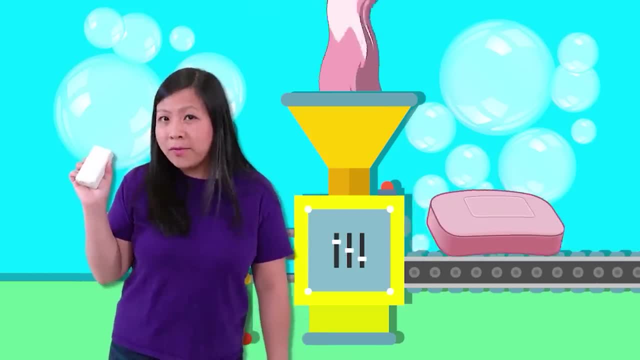 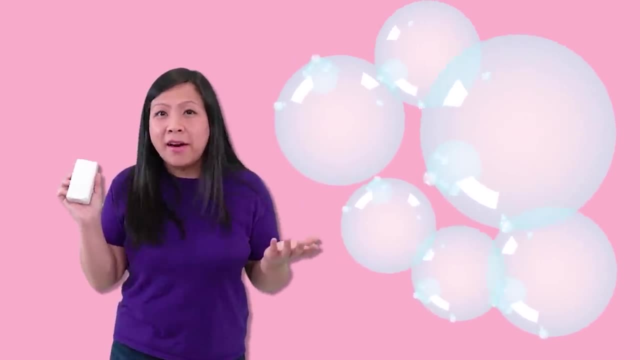 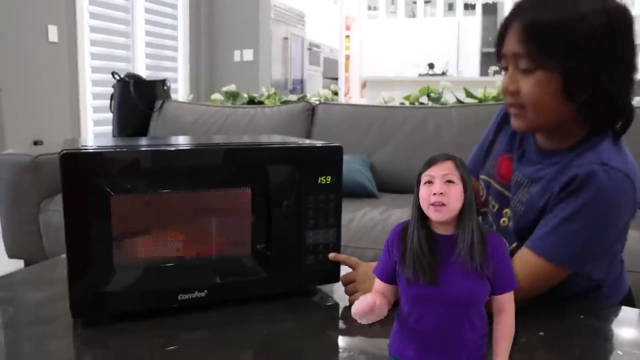 So why did the ivory soap expand in the microwave when it was made there? air that is trapped inside the mixture and because of the air that's why it floats in water. so when you put the soap in the microwave, the air and the water molecules that was in the soap starts to heat up. 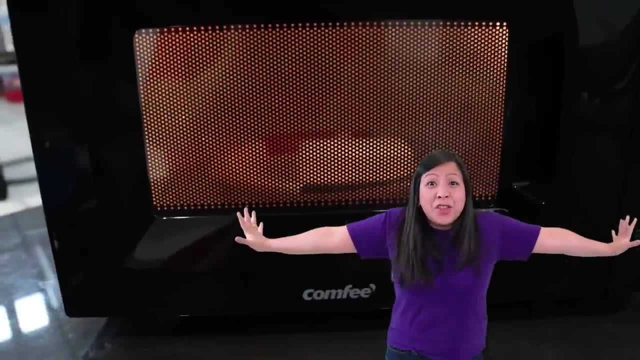 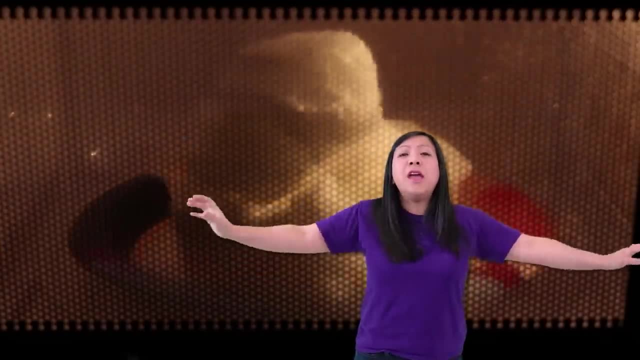 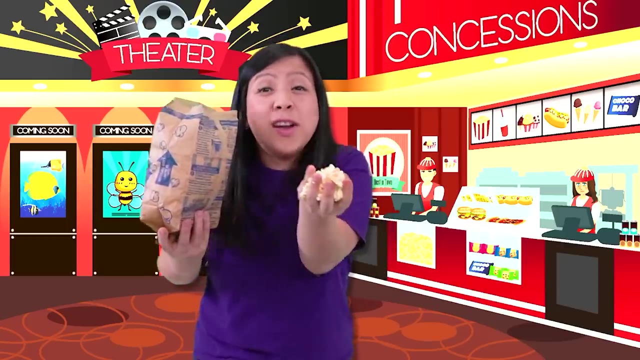 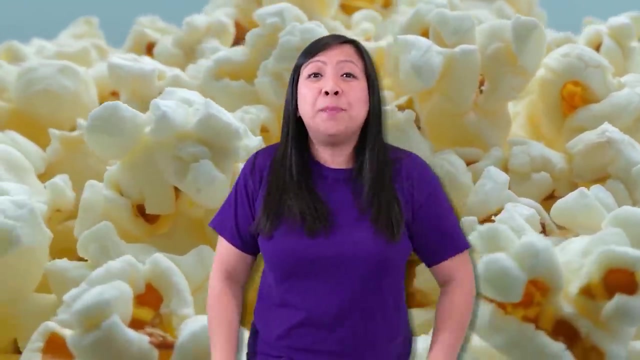 Vibrate and expand and spread farther apart. They push us against the rest of the soap molecules, expanding the bar into a fluffy cloud blob. Do you guys like popcorn? It works the same way. Water inside the kernel expands and pushes on the walls as it's being heated inside the microwave. 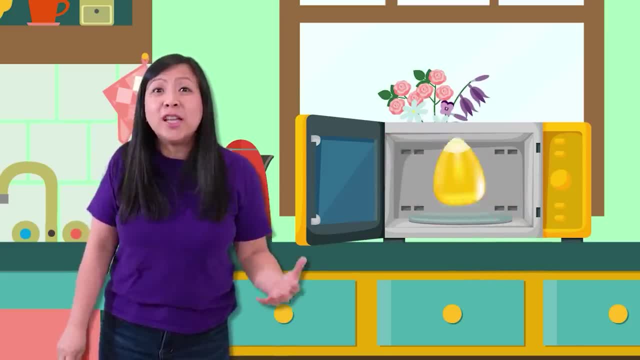 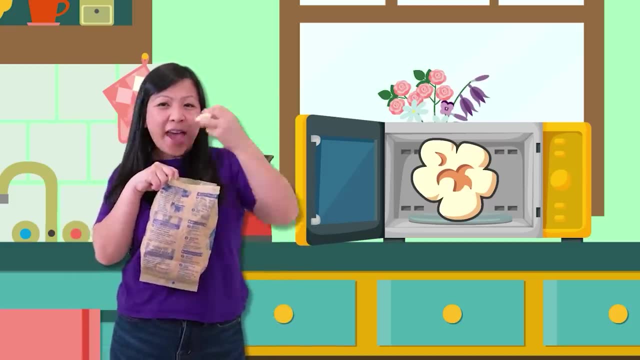 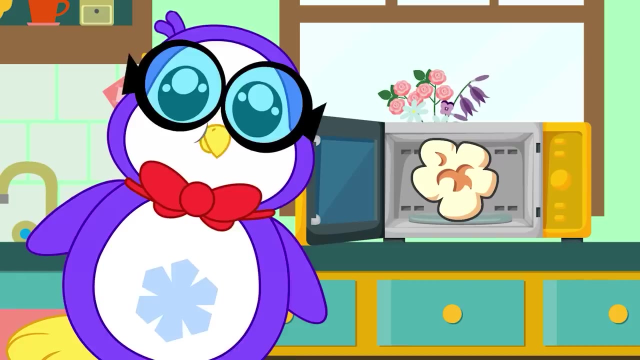 The water will turn into steam and expand and push on the walls. It pushes along the wall of the kernel until the kernel explodes And we have a yummy piece of popcorn. That was so cool. Let's get back to Ryan. Now Emma wants to touch it. 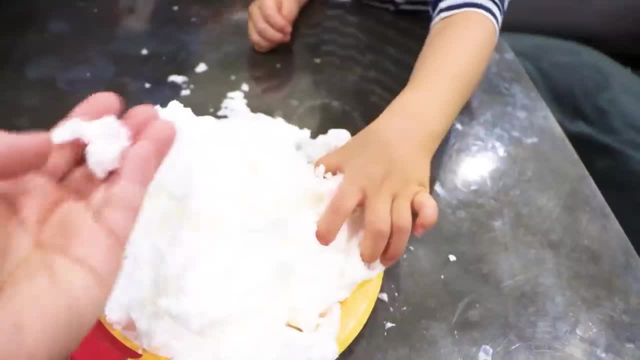 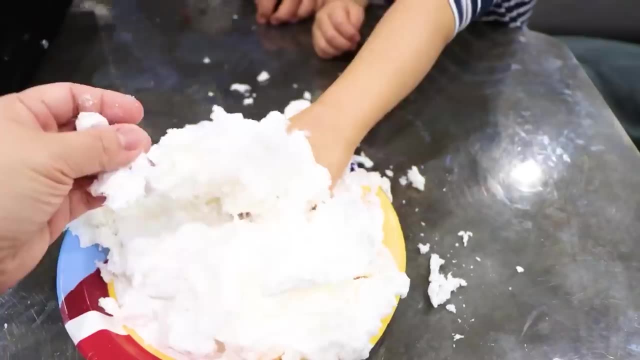 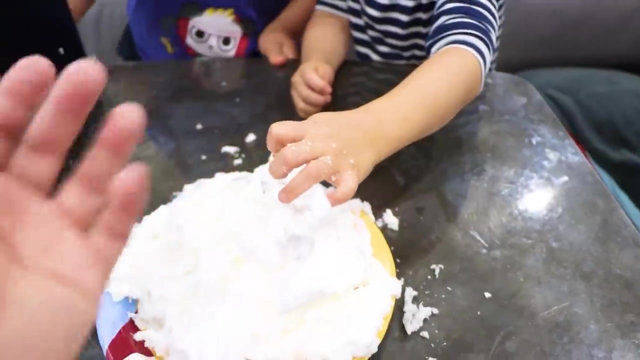 Yeah. so, Emma, this is soap. Apparently, It's like coming apart. Why do you microwave it? Well, because I wanted to show Ryan how soap expands. Yes, microwave it. look see, but it's all mushy. yeah, but it's okay, it's just soap. we can go wash your hands. 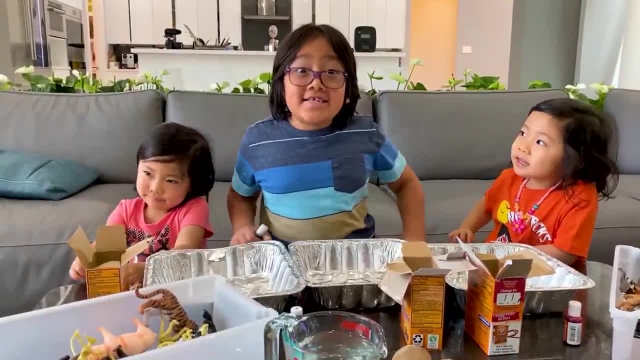 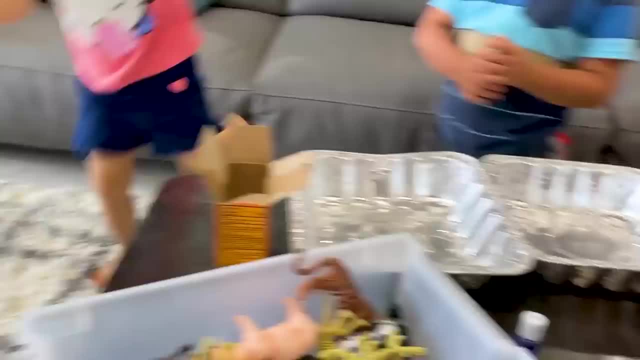 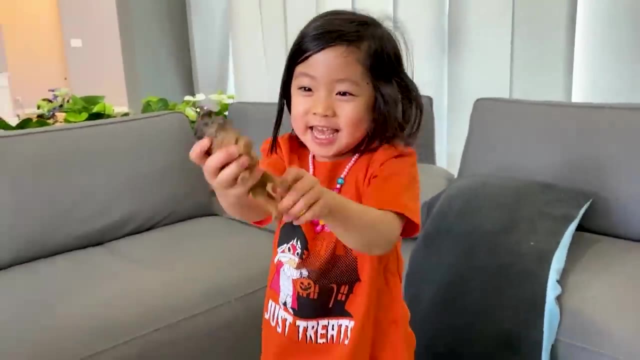 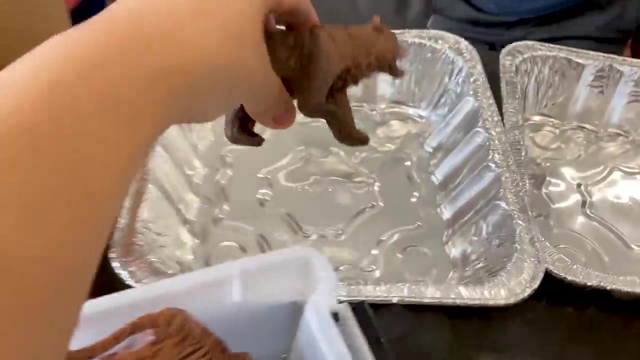 okay, isn't it cool? yeah, today we're doing a science experiment where we hide surprise toys. yeah, so we have all the leftover toys here, scary where we're going. yeah, so we have all these surprise toys here we're gonna hide. first we're gonna put in baking. 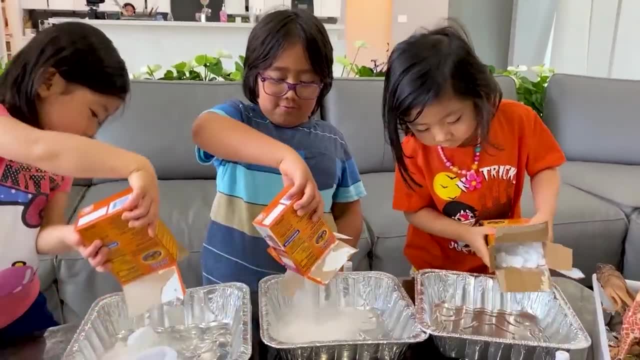 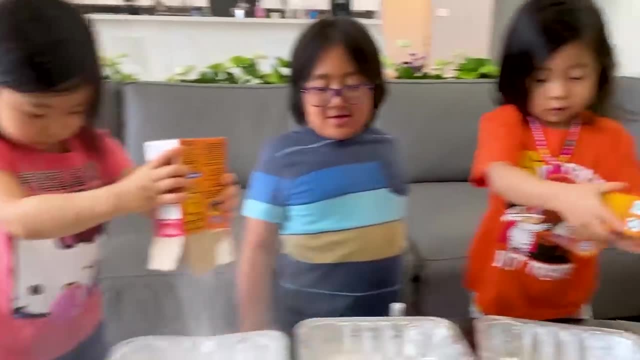 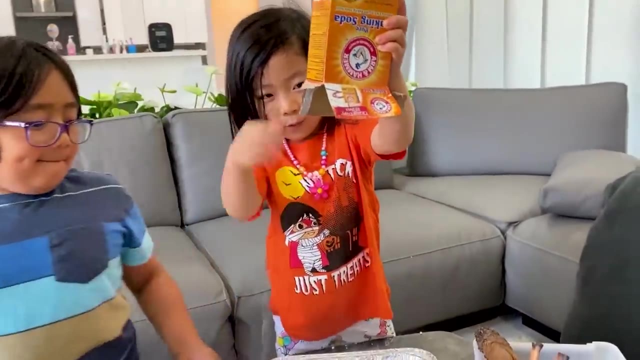 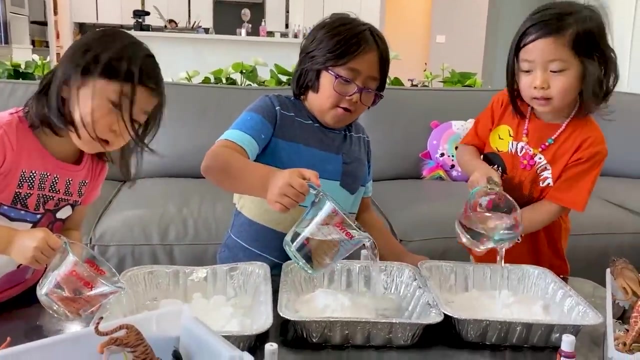 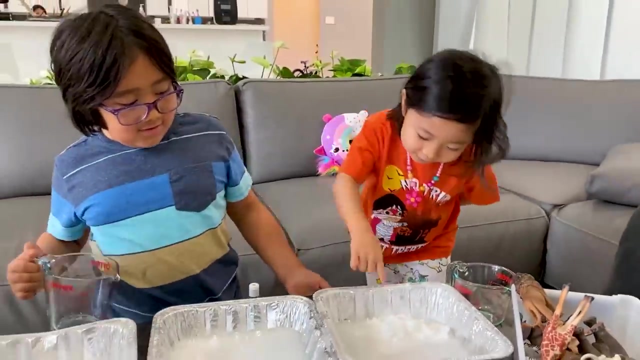 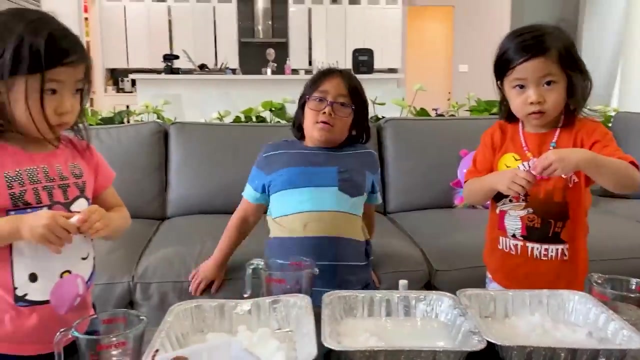 soda, all of them, all, the whole thing, the whole thing. yeah, yes, emma, looks like snow. next, let's add in water. now we're gonna be doing all of it, all of it. yeah, look like a bell. look like a bell. can i add the color? yeah, that's right. okay, so now we're gonna add color. but don't forget, this is a science experiment. you guys cannot eat it, right? 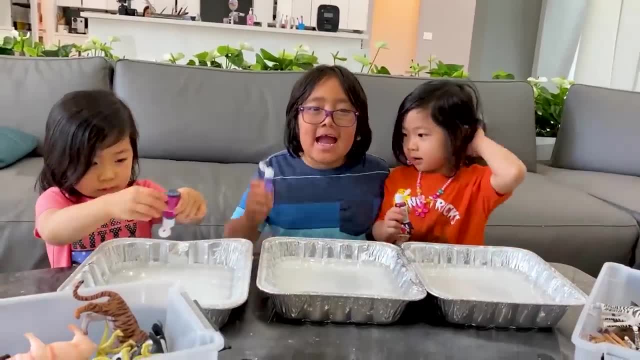 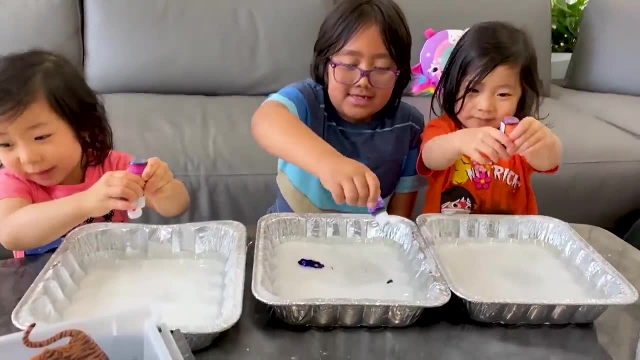 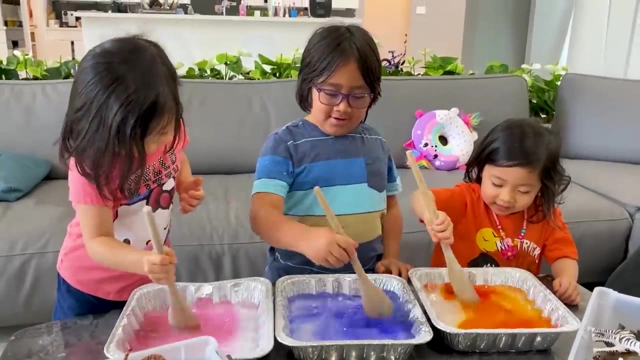 yeah, next, add food coloring, and i'm gonna use purple, i'm gonna use pink, i'm gonna use pink. do you like it pink? i add one. drop next up, let's add the pink. add the pink. mine looks like a piggy, mine looks very purpley. 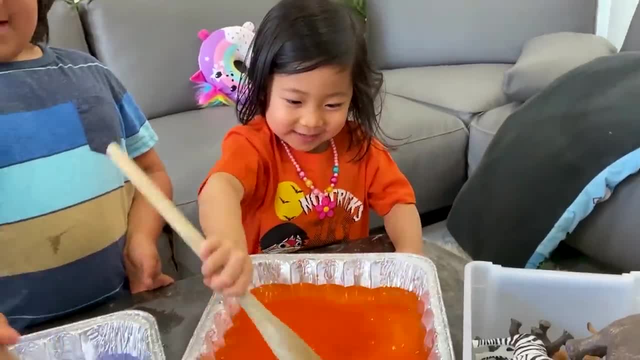 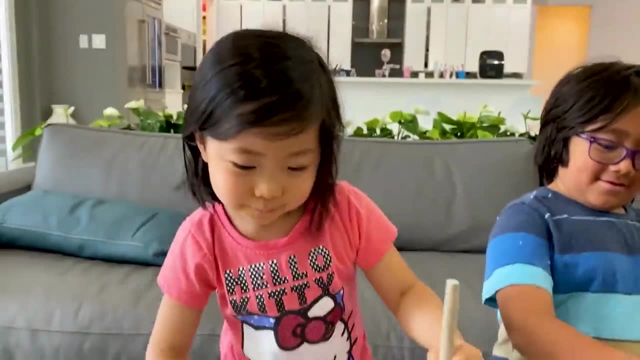 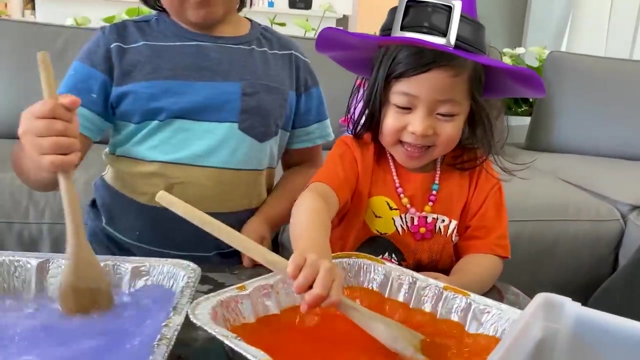 mine looks bubbly, mine looks purpley. mine looks bubbly, mine looks purpley. it's like a piggy. mine looks bubbly, bubbly, bubbly. mine looks bubbly, purpley, bubbly. whoa, emma the witch, i like your laugh that much, hahaha. 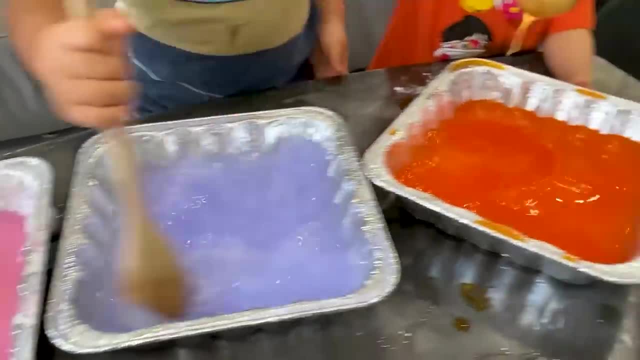 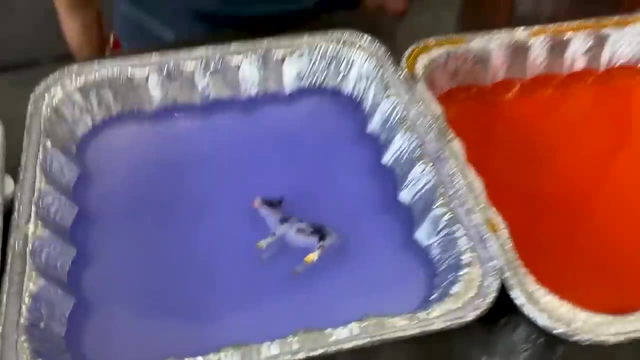 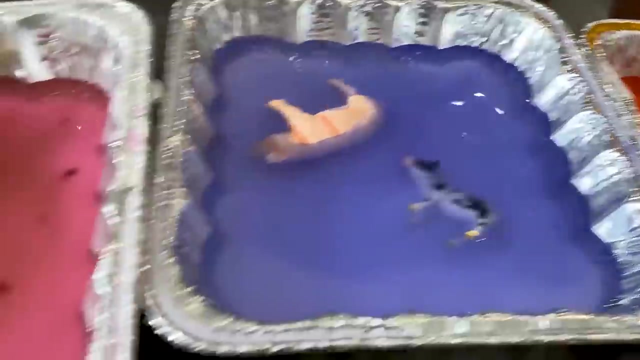 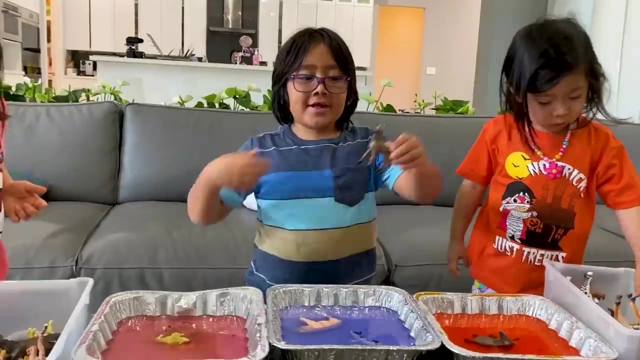 haha, there you go. now let's put some poison. yeah, anything you want, ryan, pick a cow, baby elephant, baby elephant, and and, oh, and a dinosaur. no, it's fine, you can put it. try, sarah top, i'm putting in a horse. no, okay, so just add. 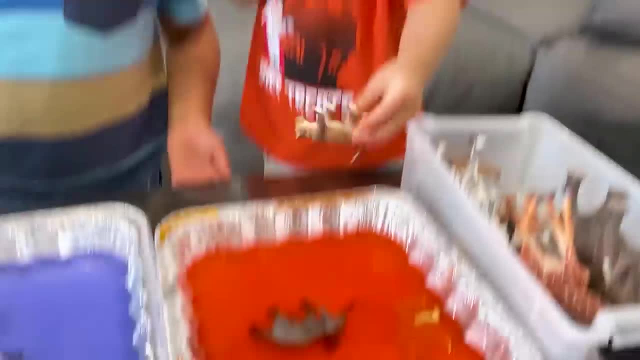 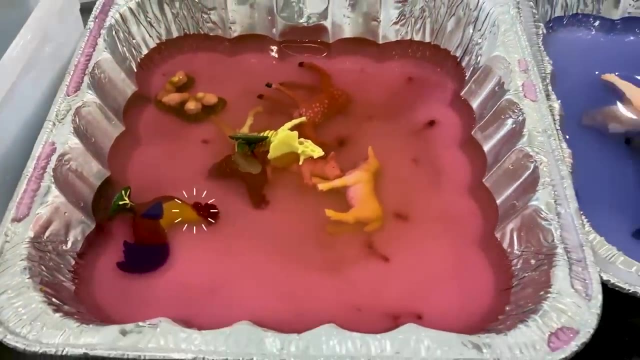 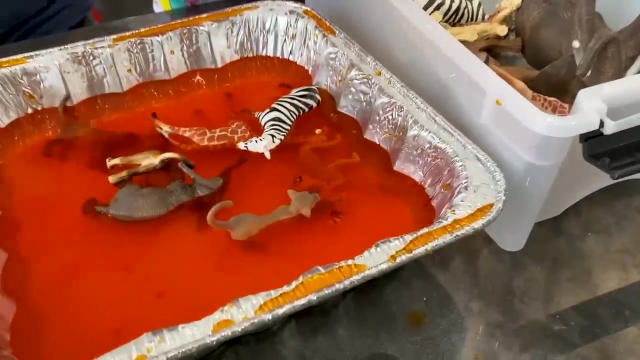 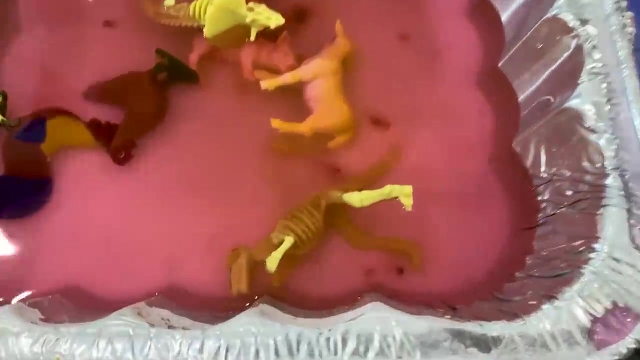 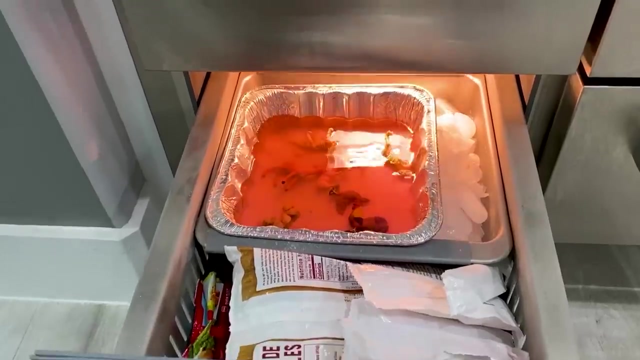 in a couple. oh, what about this one? sure, okay, whoa chicken, are you guys done? yeah, one more. okay, emma, one more. okay, another dinosaur, another dinosaur. now let's put it in the freezer, all right, so mommy's gonna do that one more time. okay, we're gonna freeze it. 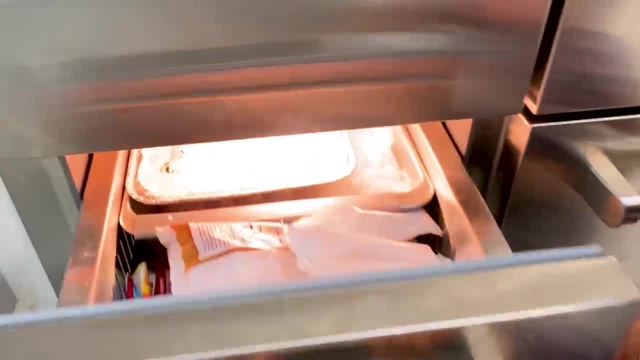 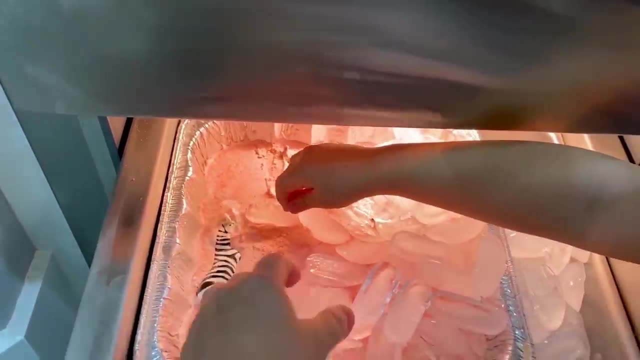 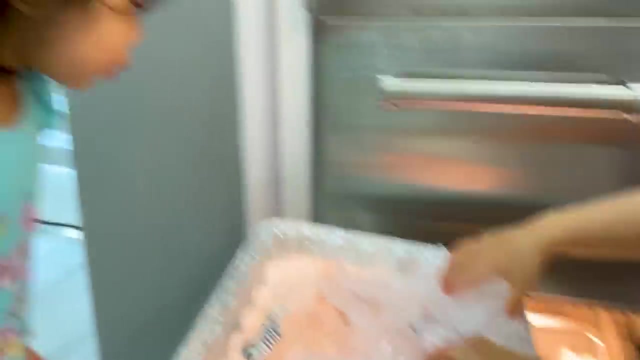 all right, i think it's ready. okay, let's see. whoa, wow, what is this one? oh, this one has ice on it, because i accidentally put it in the ice tray. is it cake or horse? i don't remember. all right, let's take it out, guys. 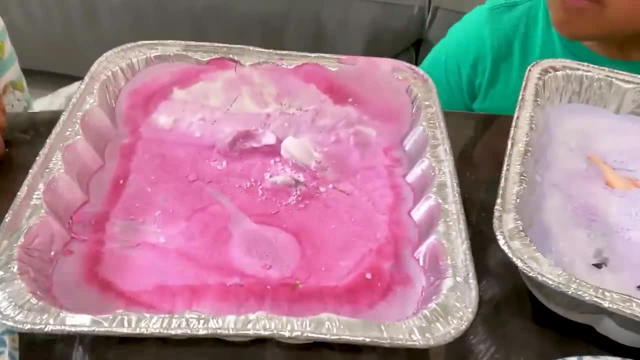 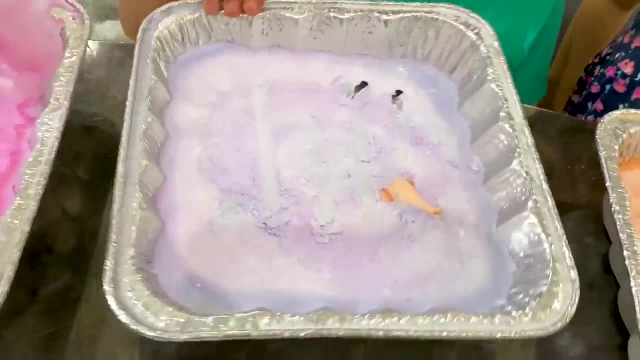 okay, guys. so now that we got it out of the freezer, that's what it looks like. some of them have ice in it, but it's okay. oh oh, ryan did right with his hand there. so now these are vinegar. so what you're gonna do is you're gonna put vinegar into. 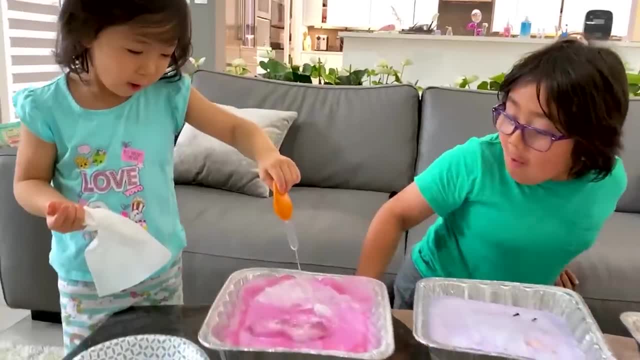 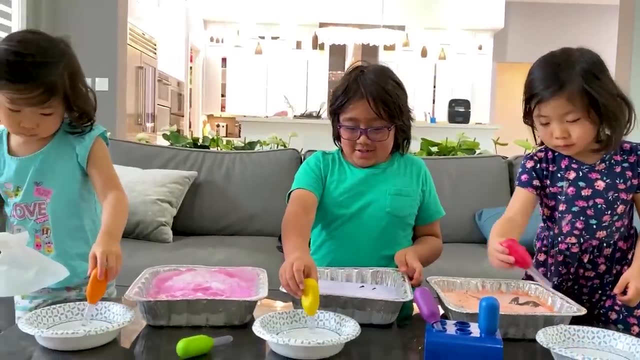 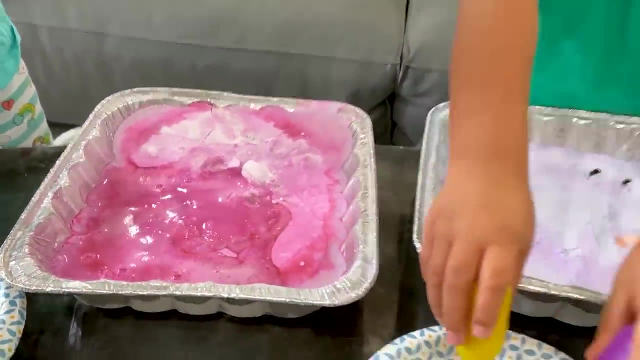 your baking soda, oh yeah. so what we're trying to do is rescue the animals that we put in there. rescue the animals. yes, that's the goal: rescue the animals. so why do we put the animals there? they're having a fun bath. i'm trying to get this one animal. 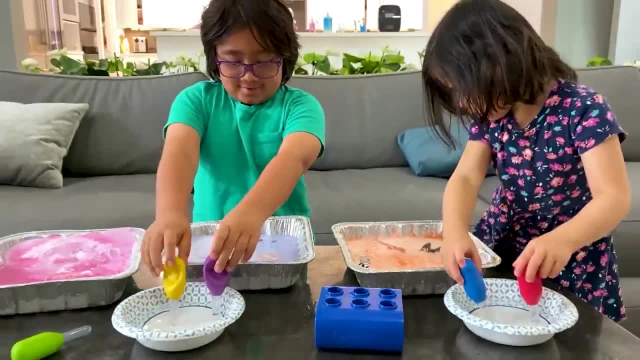 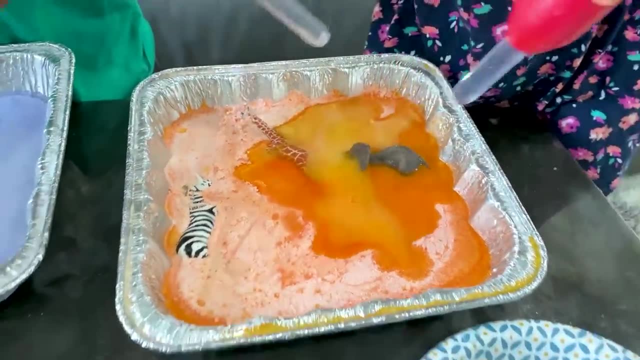 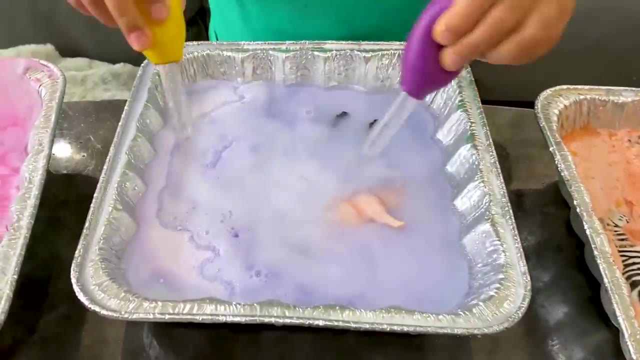 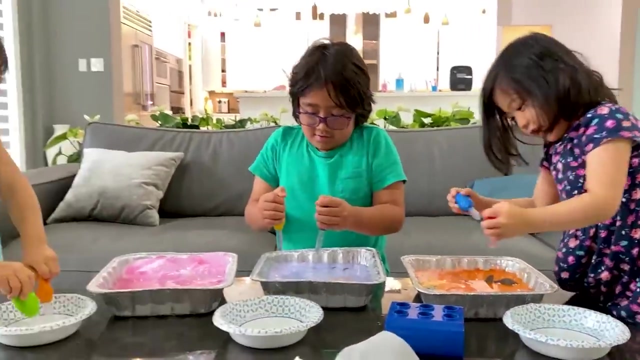 what was that? did y'all see it? i don't know what it is. now it's Kevin. oh, i'm saving both of them. i would say lots. i have a lot, i know. whee. whoa good job, kate. save the animals. they're having a bath. 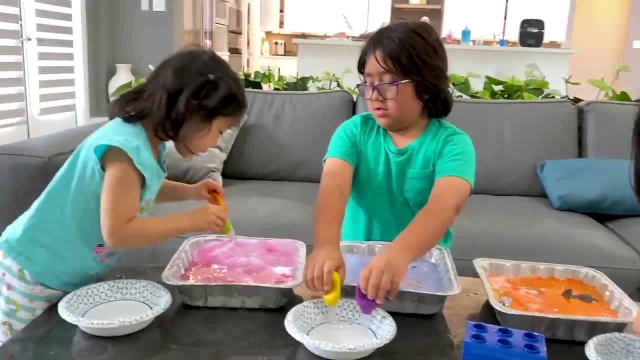 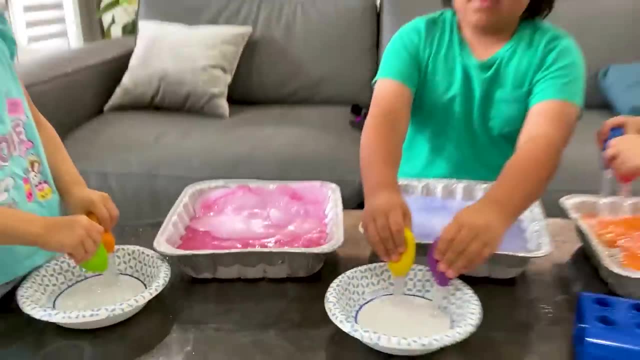 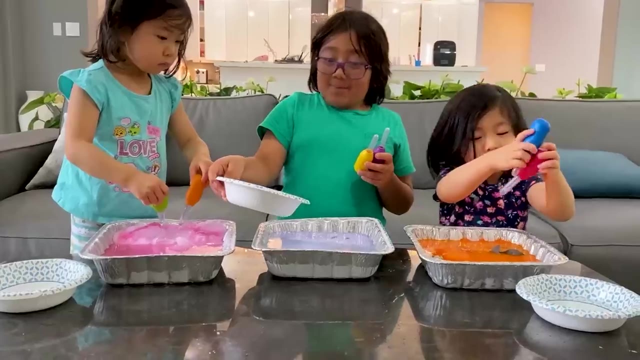 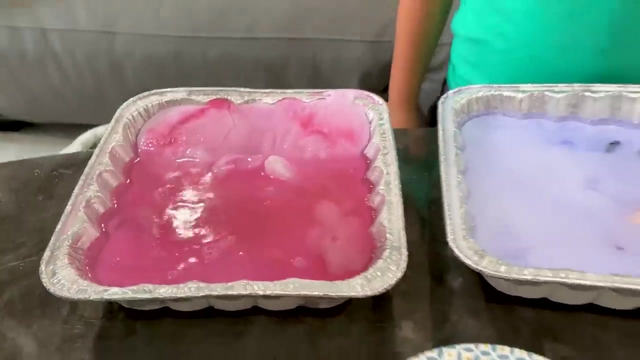 they're having a bath. yeah, why? hehehe, whoa what? everybody helping each other. how nice looks good emma. yeah, i'm gonna put the whole thing because it's not going that fast. me too. whoa, you wanna do that too? not yet. we need way more. 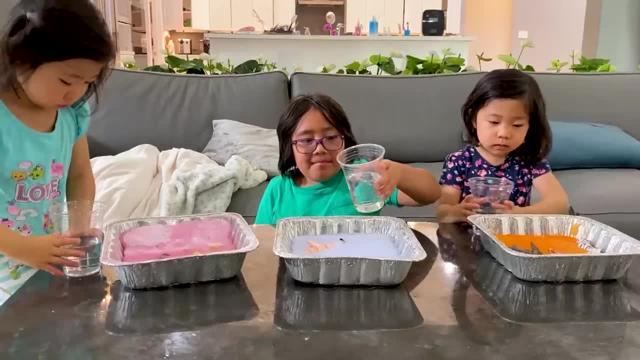 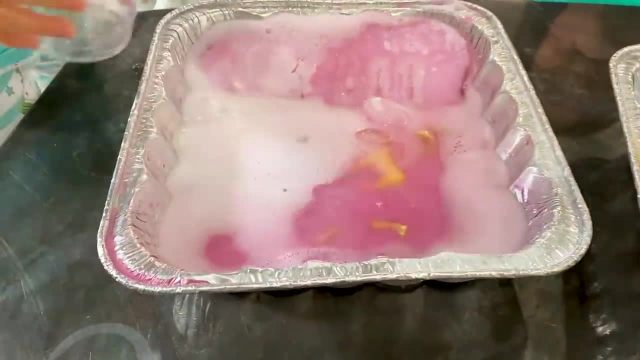 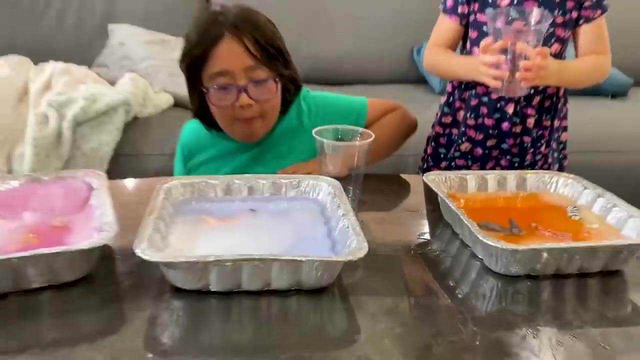 yeah, emma, all right. so now i'm just gonna give them a cup of vinegar. oh, look at the bubbles. look at it bubbling. look at it, bubbling, it's bubbling. yeah, can we save the animals? yeah, can we save the animals? i want that animal. 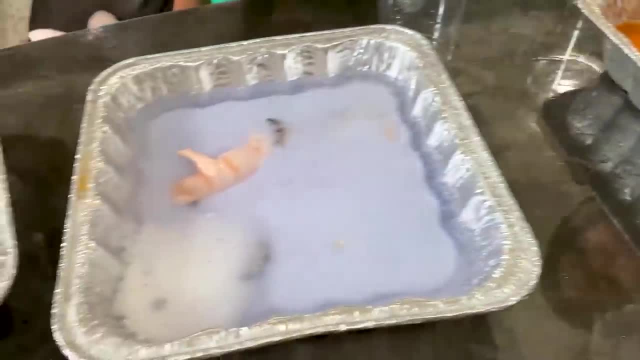 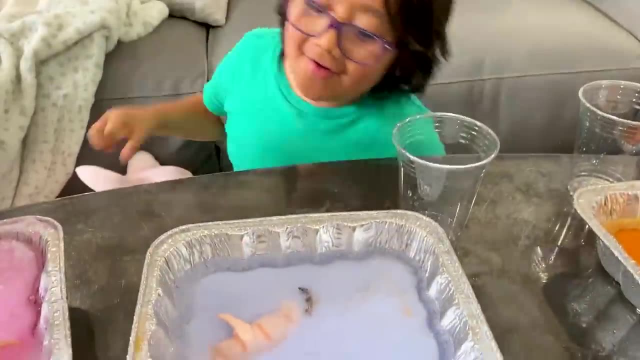 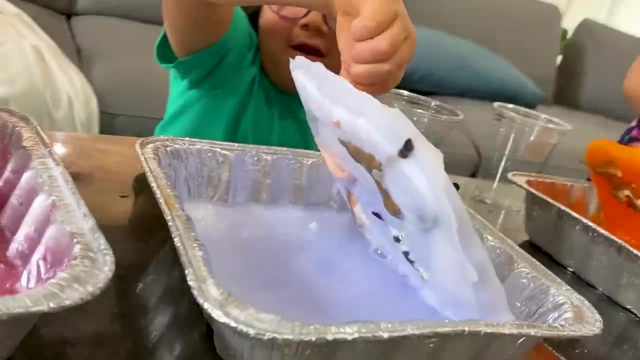 oh, oh, almost. can emma take it out? let's see if emma can take it out. almost i cannot, ryan, not yet. hehehe, whoa, so close. oh, look the animals on the other side. okay, guys, we are so close. we're gonna try one more time. 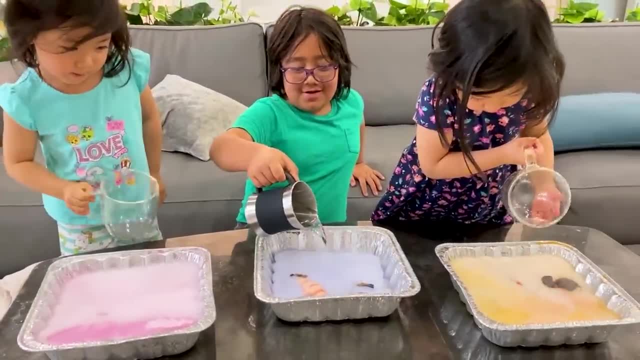 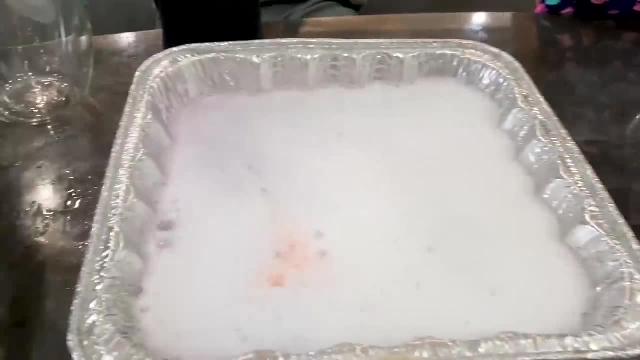 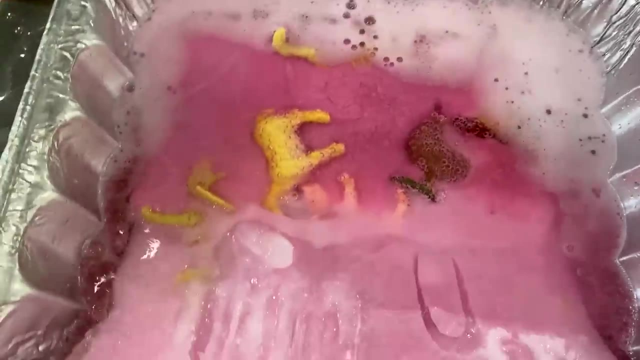 can we rescue the animals? oh, that water probably works a lot more. yes, we actually warmed up a water. this is a fun video because the kids can help each other figure out how to rescue the animals. mommy, yeah, almost so close. you can see the animals here, so close. 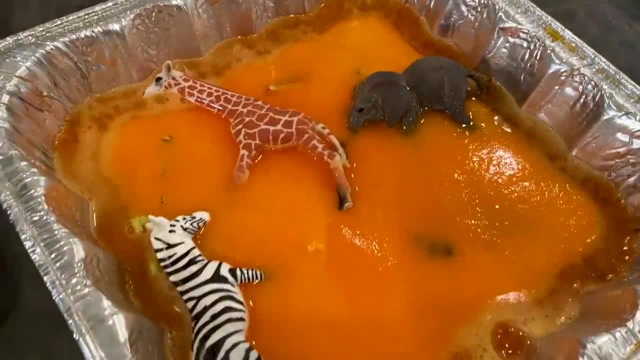 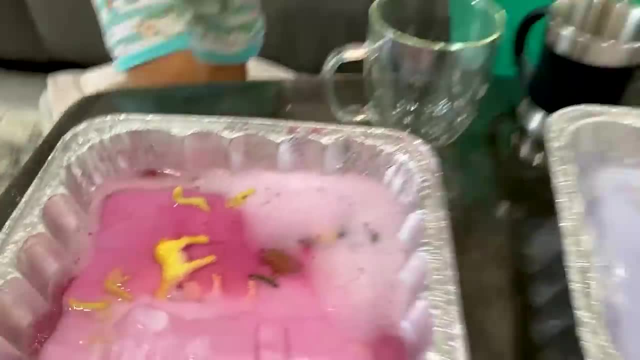 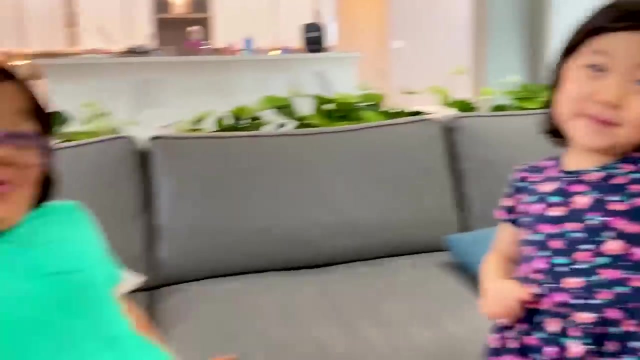 ryan's so close. look, it's moving, i'm gonna get mine out. look, i'm gonna get mine out. i know that's the point. we gotta figure out how can we rescue the animals. how about we do hammer? good idea, all right, not strong hammers for us. 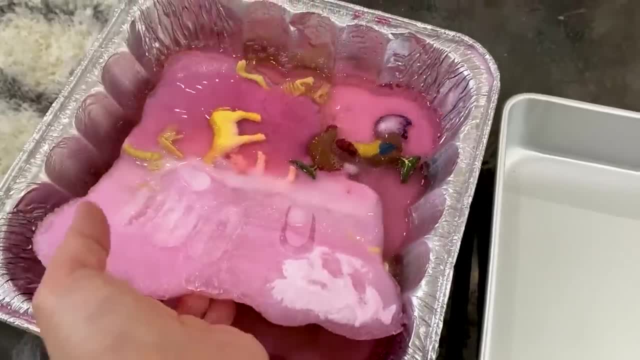 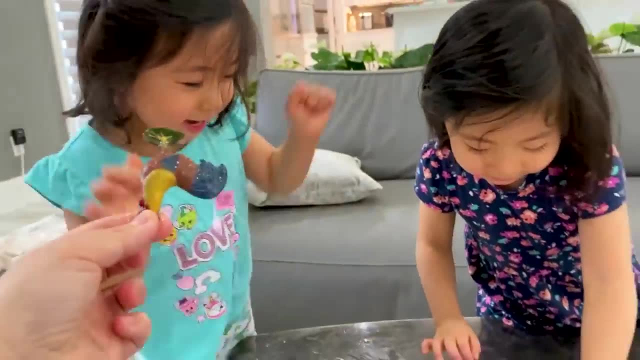 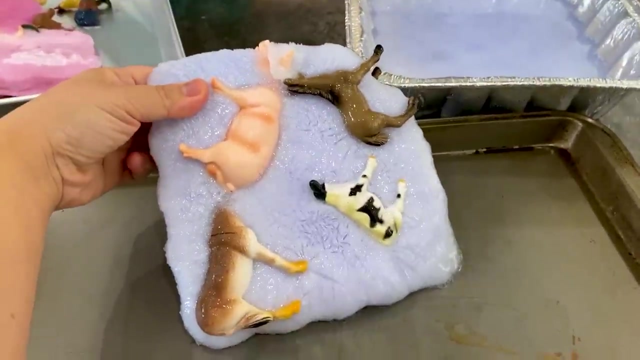 not strong. yeah, good idea, ryan. first mommy's gonna help put it into a tray so you guys can break it up. look, we got one. yay, good job. okay, this is ryan's. i'll take it out for him and it's almost done. look, look at the back side. 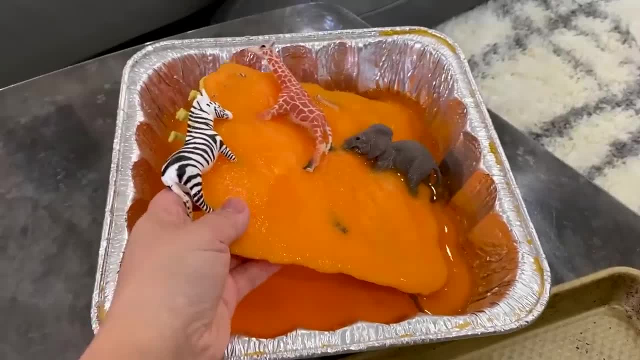 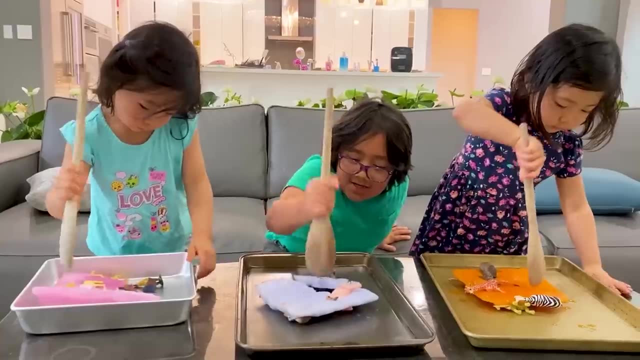 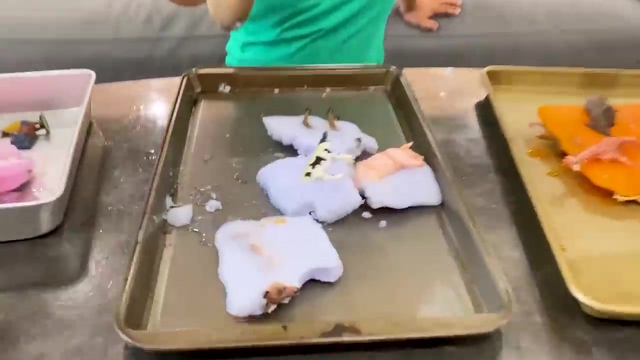 you guys can see what animals he picked out. hehehe, and this is emma, really, really close. she also puts a dinosaur. we actually don't have a hammer, so i'm giving him a spoon. well, ryan, good job. whoa, whoa, where am i gonna get? 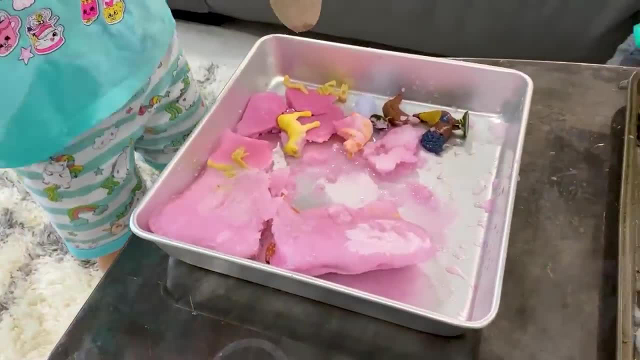 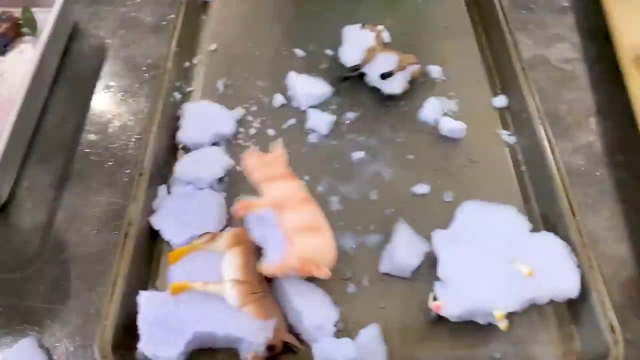 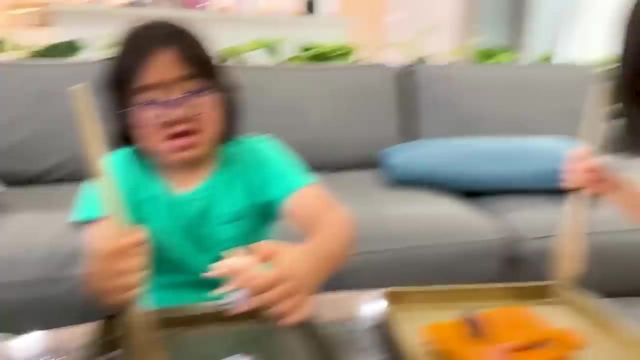 oh okay, this is a very messy experiment. where am i going now? i think i'm dead. you rescued the zebra, i'mma rescue the pig. is this really a rescue leg? hahaha, what about you, kay? did you? i rescued a dinosaur? you did. did you rescue anybody? 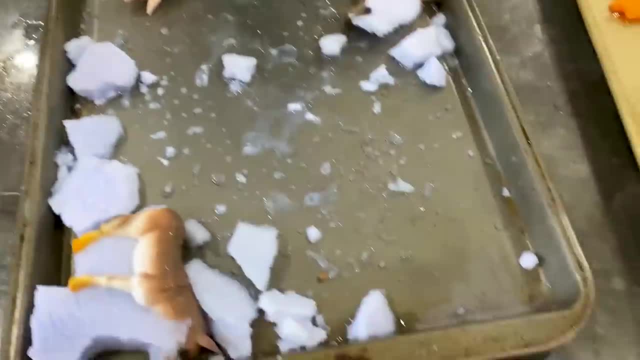 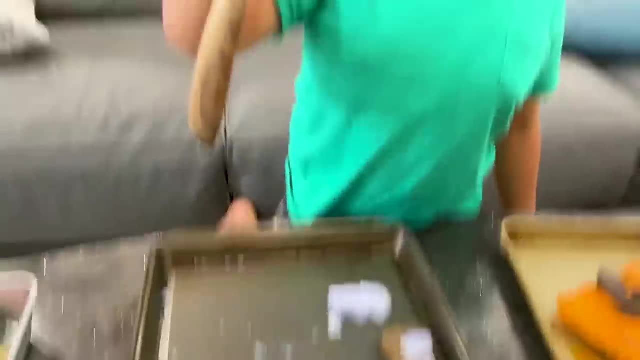 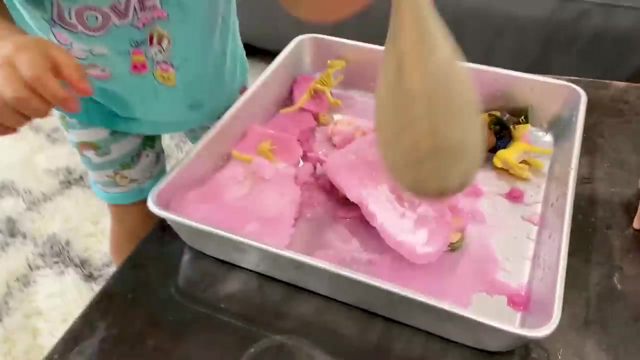 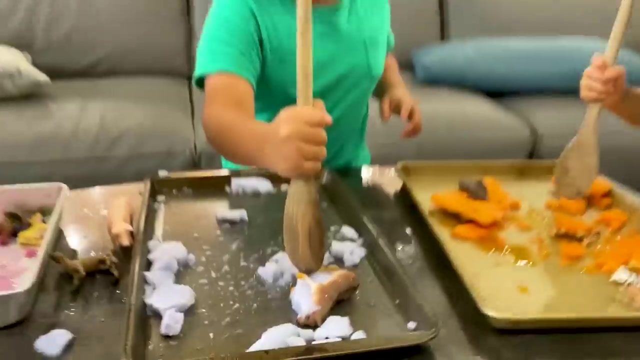 wow, almost done. whoa baby giraffe. good job, mommy. look, i got the pig, you did ryan. nice, just one more. the horse. i got the baby blue, i got the horse. oh, one more. what is that? is that a donkey? i forgot, it's a hyena. 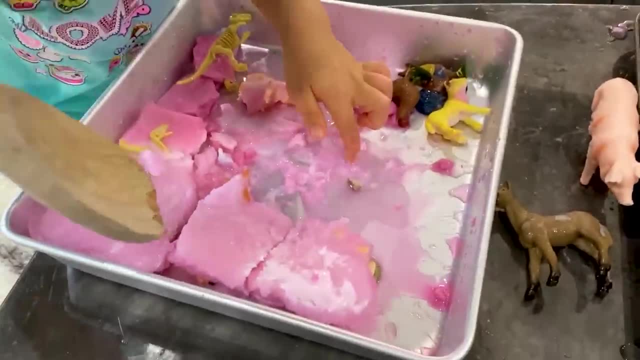 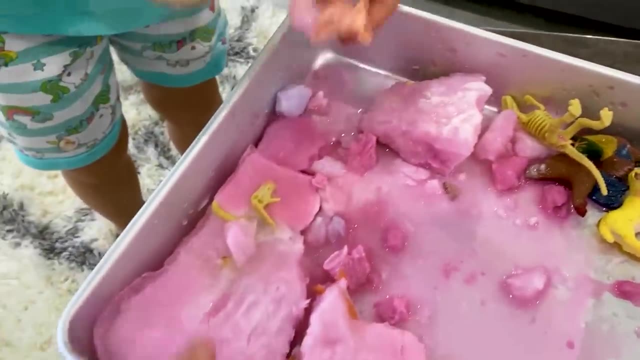 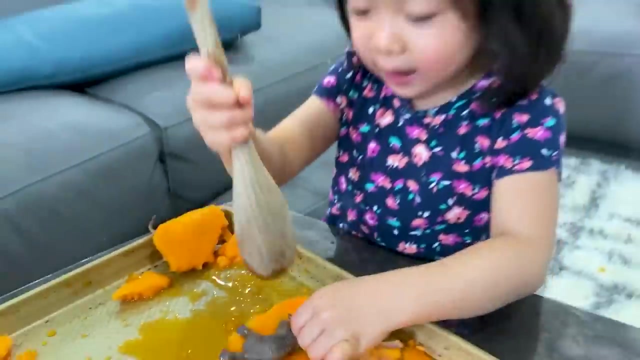 oh, hyena, i think this is a baby tiger. you got a baby tiger, yeah, wow, kay's almost done. look, she just needed to rescue the piggy, and then there's one giant dinosaur. huh, what is that elephant? i think it's a mommy elephant for the baby. 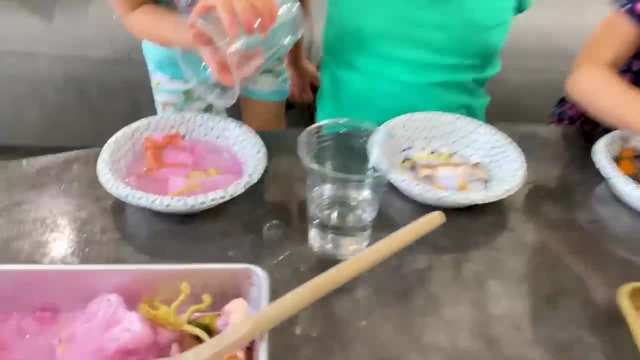 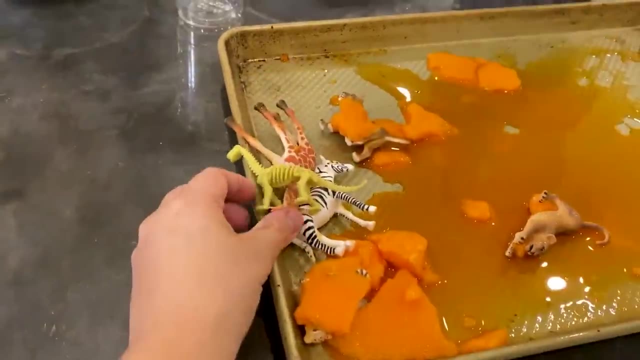 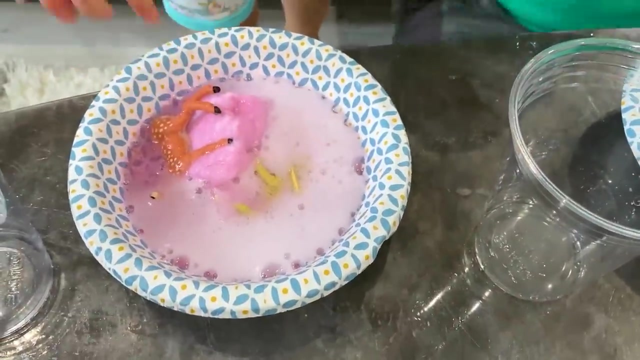 whoa, almost done. okay, so we just have a few more animals here to rescue, okay, yeah, they rescued pretty much all the animals already, except for these. oh, look, it's going. you see the bubbles? look, we rescued all the rest of the animals. yeah, look, it's out. 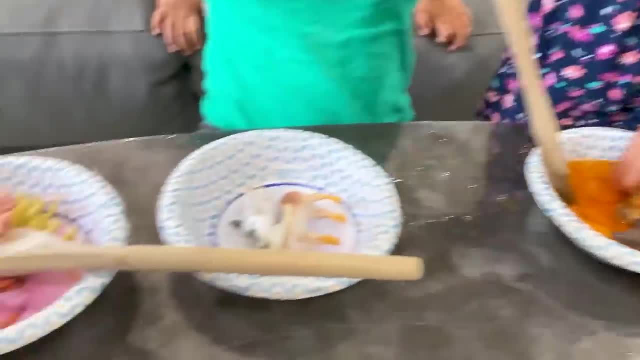 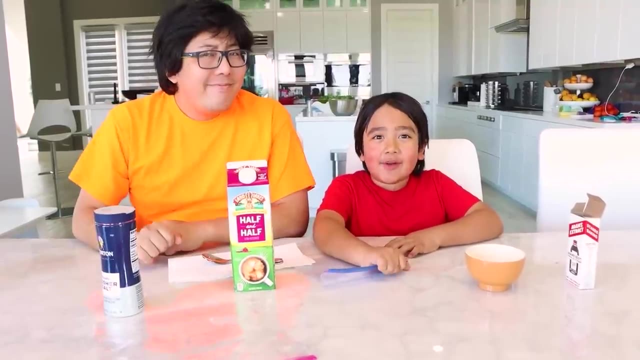 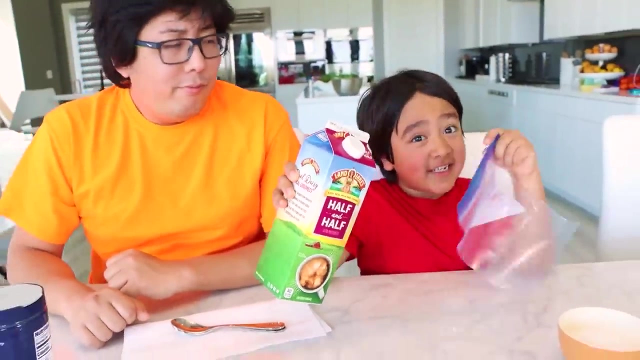 so emma's almost done with hers. yeah, good job. looks like soup, looks like soup, hahaha. hi guys, today we're going to make ice cream in a bag, so we're going to put half and half, and you can put as much as you want, because that's how much ice cream we're going to make. 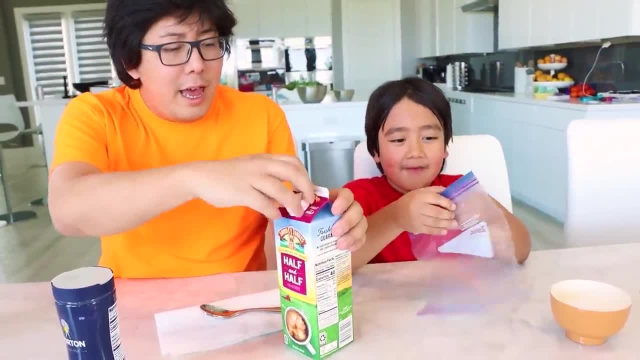 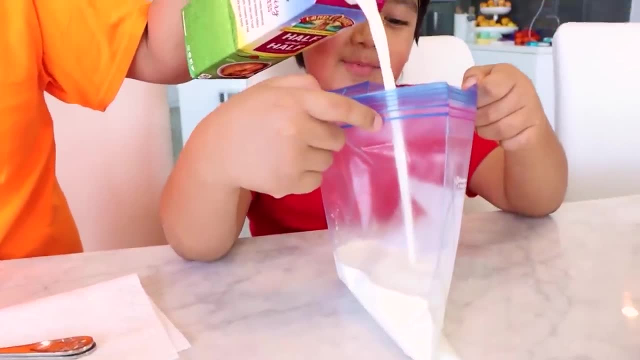 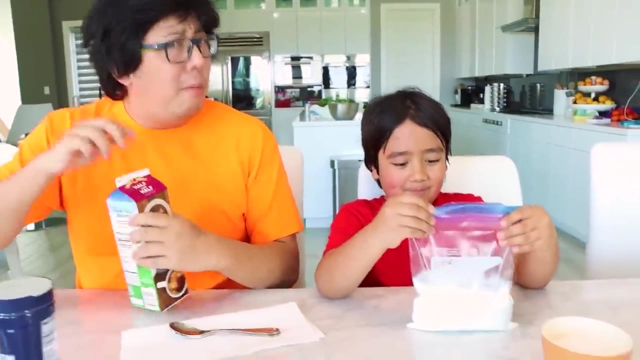 that's right. alright, let's open this half and a half. ryan, why don't you tell me when to stop? okay, okay and keep going, keep going, keep going and stop. alright, that's plenty of ice cream for both of us. yeah, if you want some sweet ice cream, 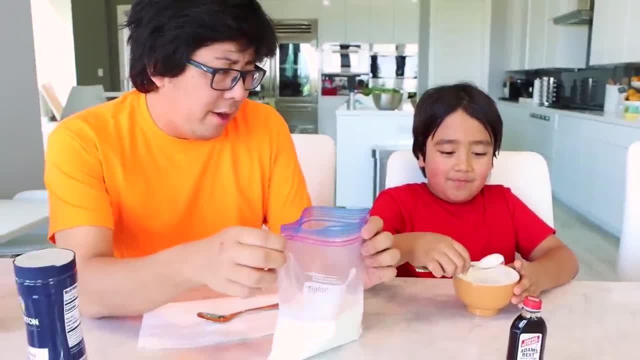 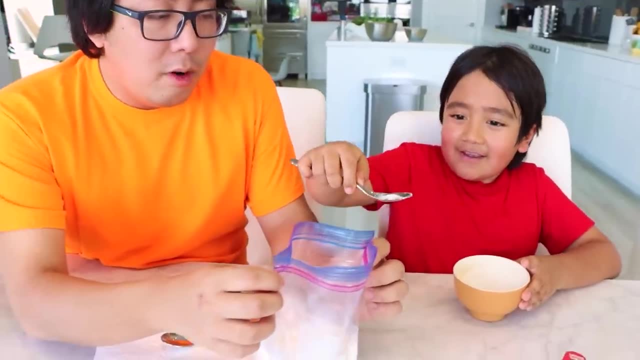 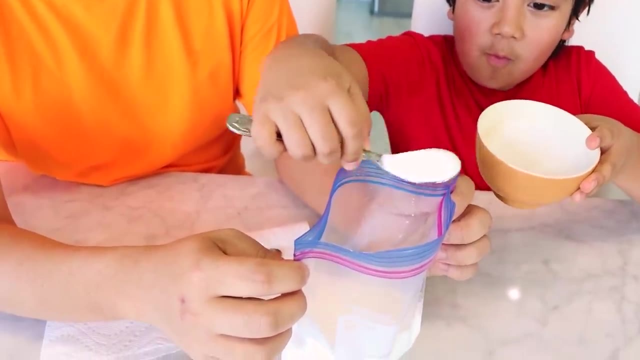 then add a bunch of sugar. yeah, so this is for just the flavoring. you need the sugar and also vanilla extract. okay, you think this is enough. yeah, a little more, probably. it's okay, you can do two scoops if you want to, alright, alright, sprinkle, sprinkle. 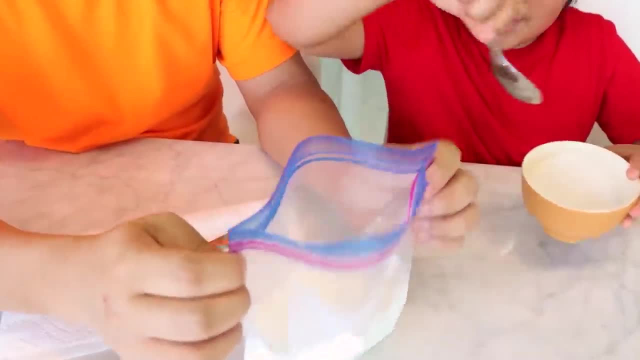 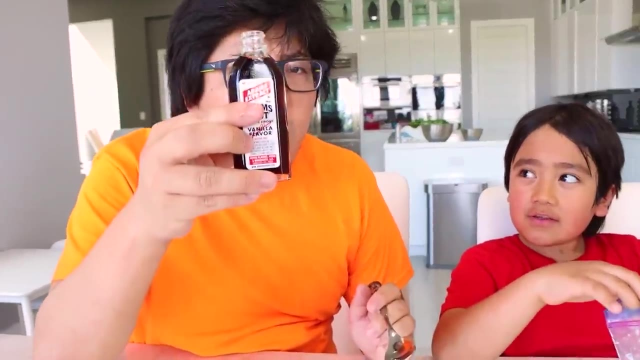 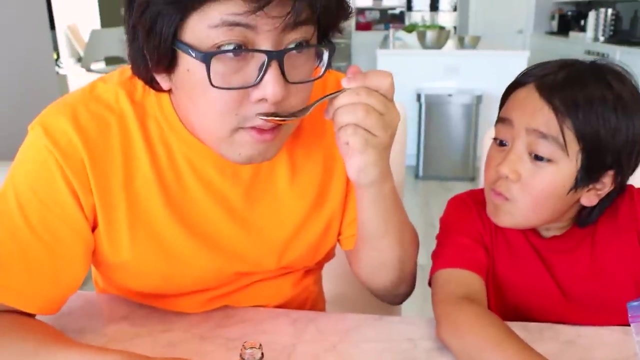 maybe just one more scoop, I think: alright, okay, alright, I almost spilled it. so we're making vanilla ice cream, so we're going to use vanilla extract, add the flavor of vanilla and it will smell like vanilla ice cream too. oh, yeah, yeah, yeah. do you smell it? 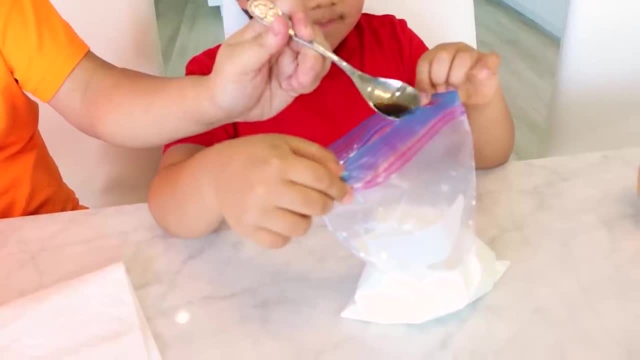 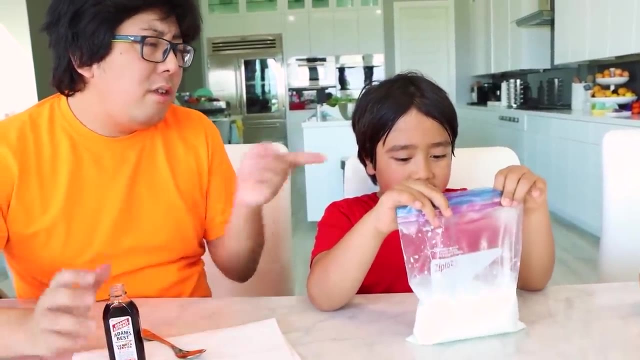 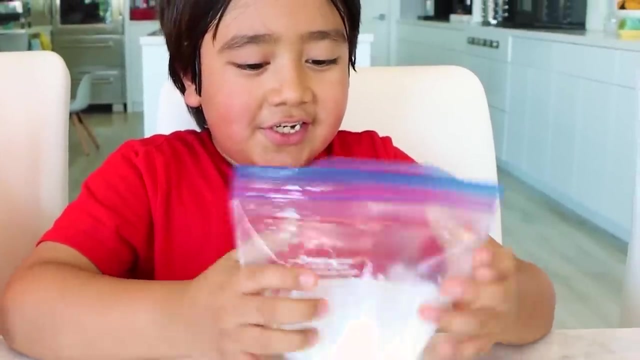 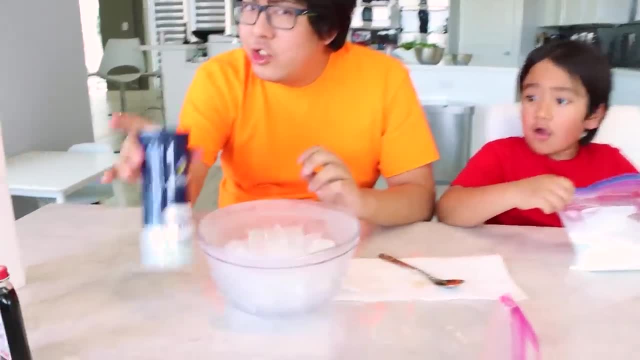 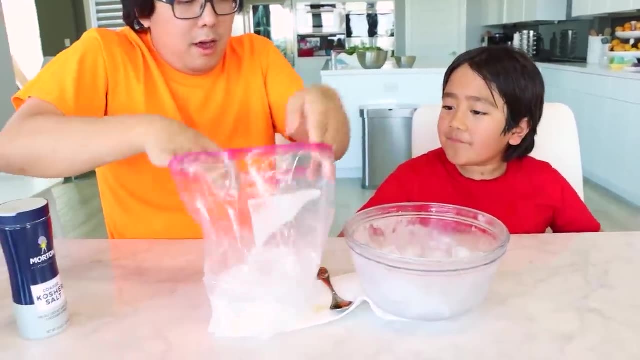 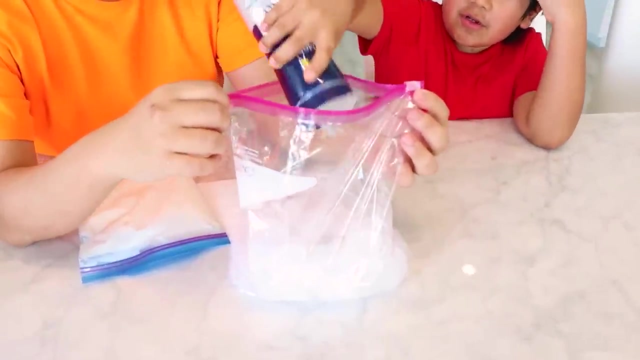 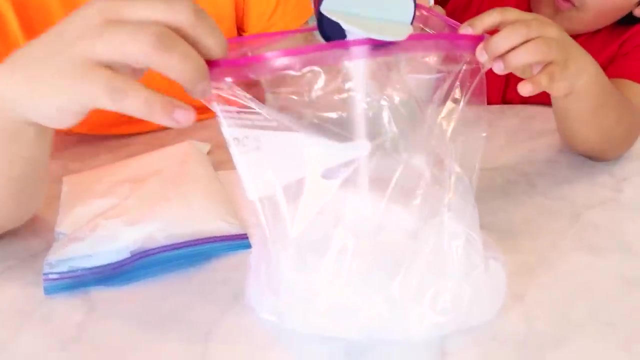 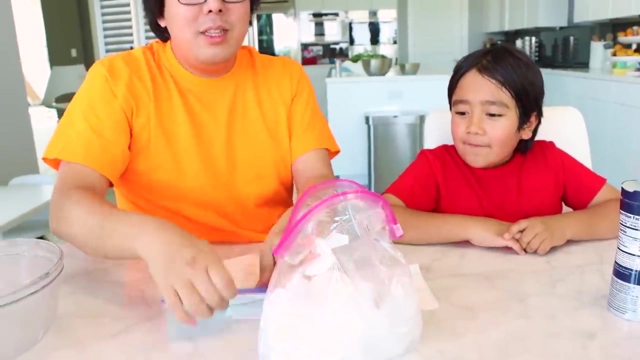 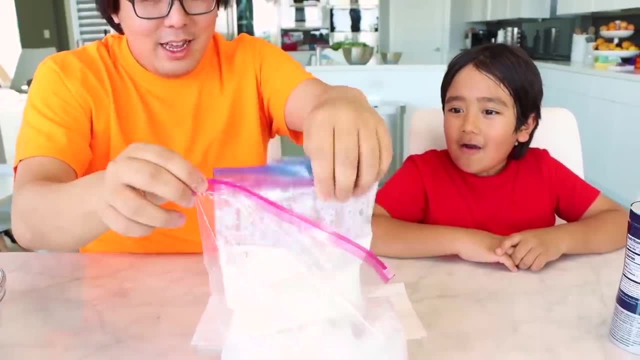 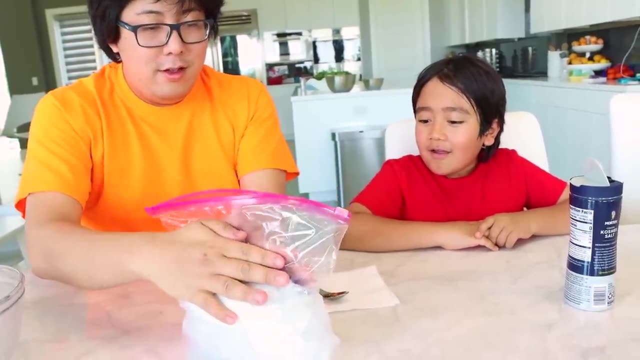 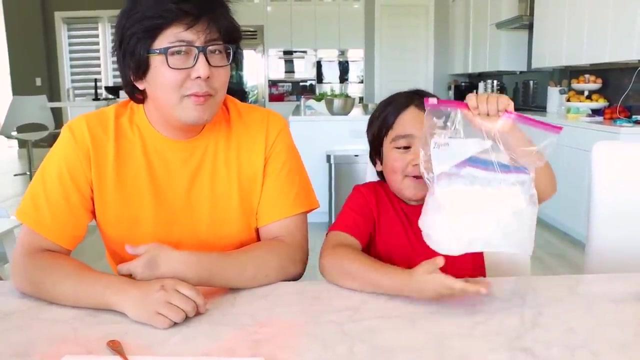 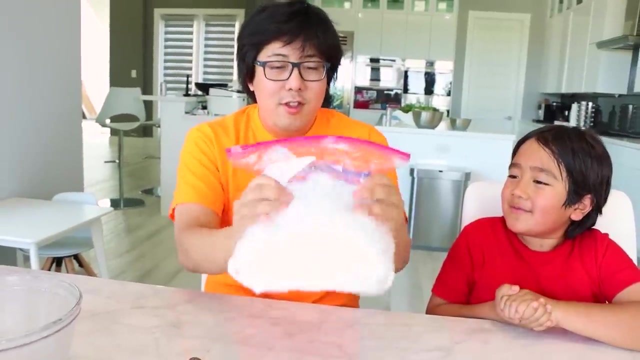 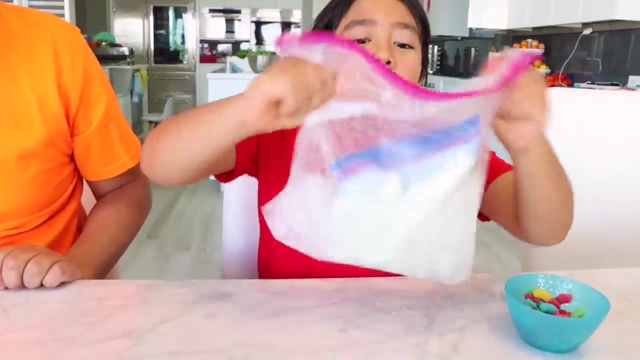 inside. what do you want to do after that? so next we have to shake the bag for at least 5 to 10 minutes. then we get ice cream. yeah, that's a long time, so we recommend you guys take turns. so once it completely, it's almost ready. 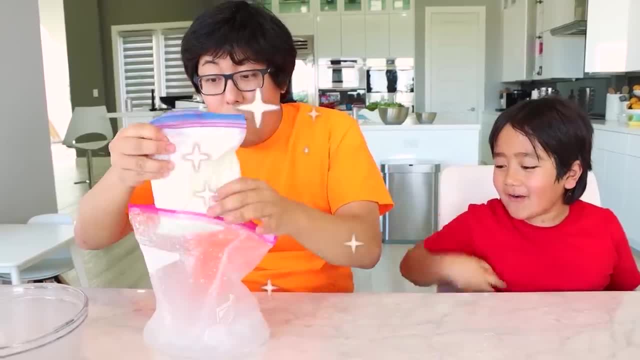 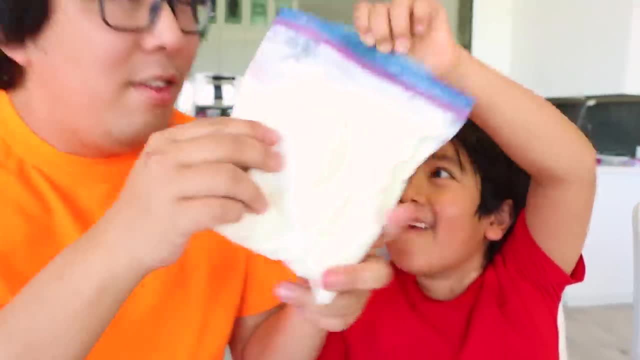 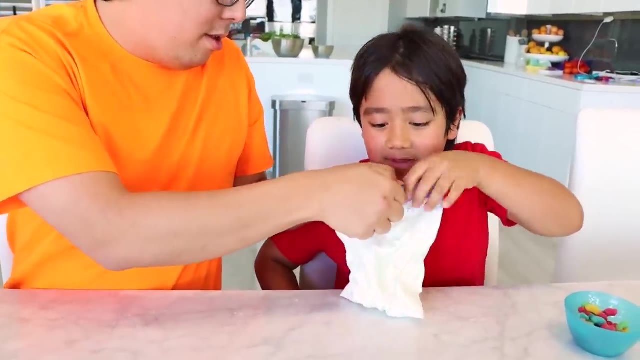 ok, it's done. labread- ok, it's done. look at all that water, Phil it. what smell it? I don't like. I can smell it through the bag. you can smell it, I smell it. I smell it a little messy. Does it smell like vanilla ice cream? 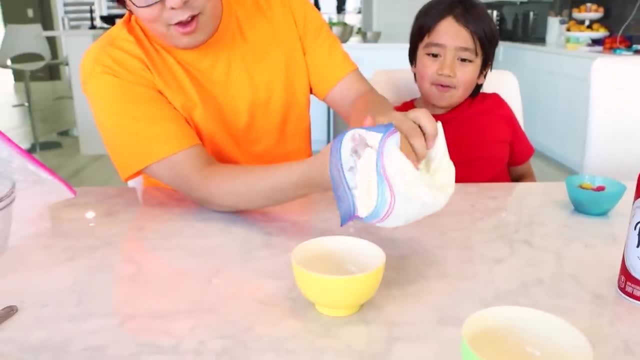 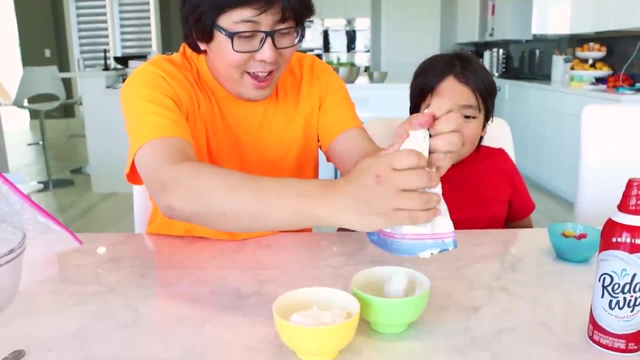 It does, It does. Let's take it out. Ooh, look at that. Whoa, Whoa Homemade ice cream. Oh, yeah, yeah, yeah, yeah, yeah, And it's super cold, Too cold. Look at that. 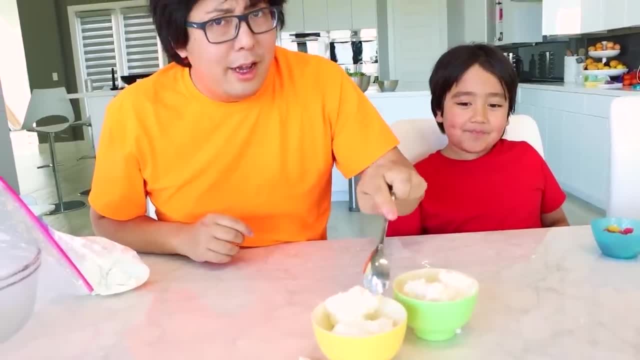 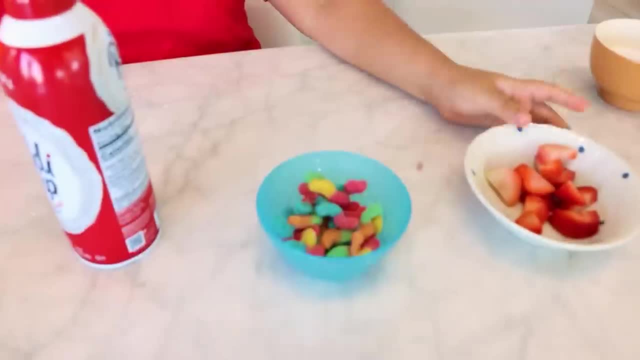 I think we made a little too much, But this is we're not done yet, guys, because you know you could eat this ice cream as is, but you can add toppings right, Like whipped cream, gummy bears, strawberry. 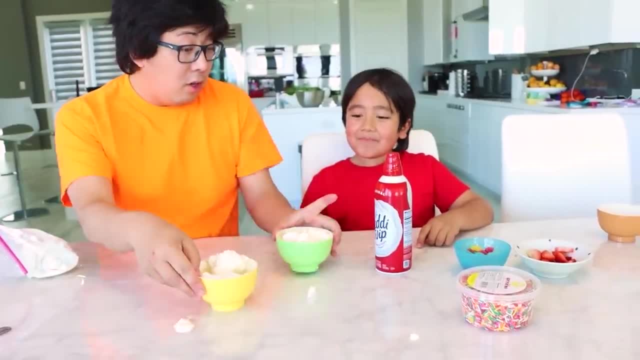 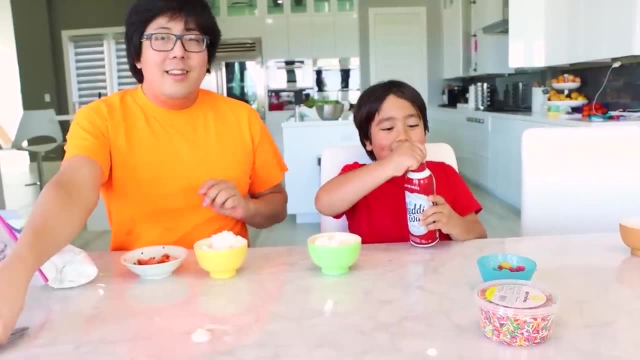 and sprinkles, of course, Okay. so this is yours, Ryan, and this is Daddy's, Okay, Okay, all right, let's add toppings. Obviously gonna add this, Of course. Ryan always loves adding the whipped cream. I like adding strawberries. 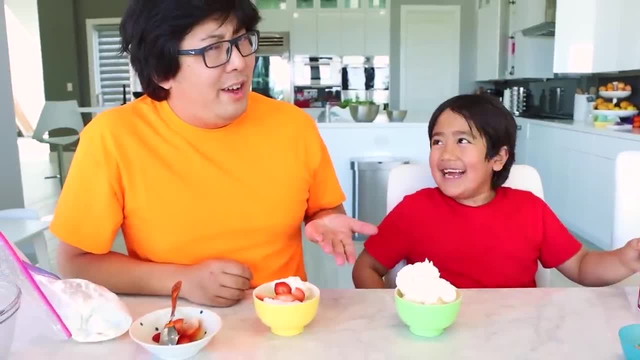 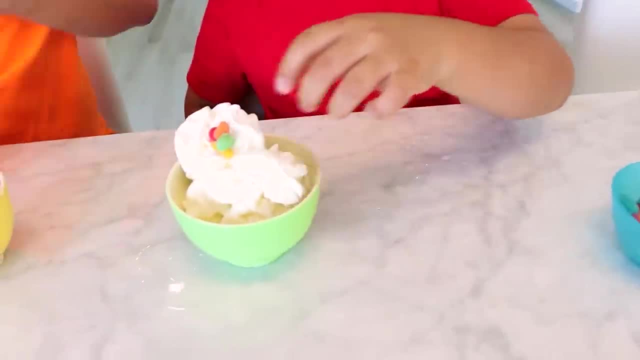 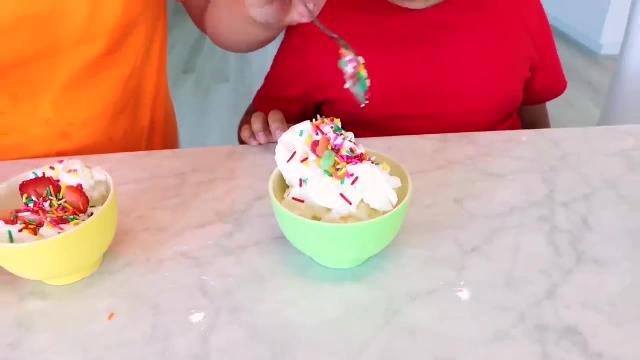 Oh my gosh, Are we eating whipped cream or ice cream? Mm, You make one baby. Add some sprinkles for mine And some of these, Mm colorful Welcome sprinkles. Ooh, Nice, Nice. 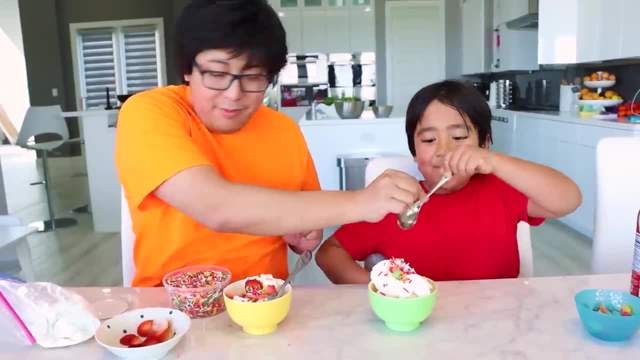 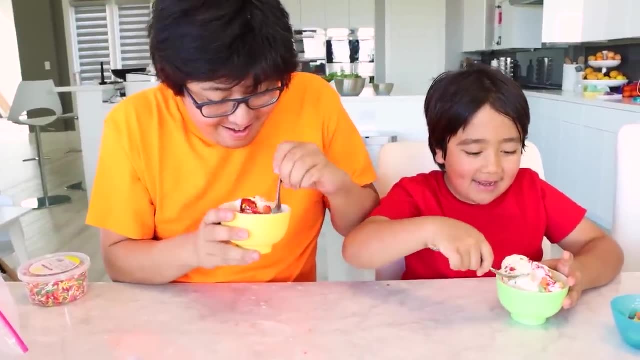 Nice, Nice, All right, here we go. Yay, we made our own ice cream in a bag, Woo-hoo. Now it's the fun part: we eat it. Yeah, I don't even know if I'm eating the ice cream. 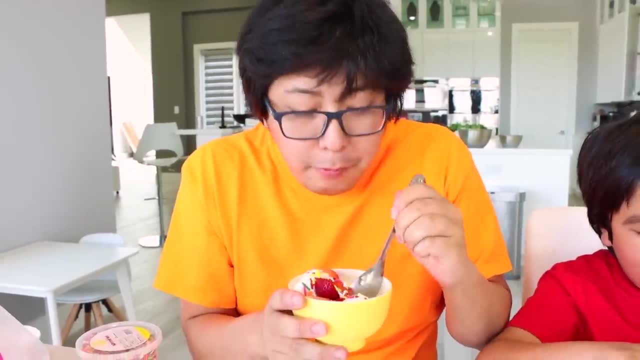 I don't even know if I'm eating the ice cream. I don't even know if I'm eating the ice cream. Mm, It's good, I'm trying to get the thingy. Oh, oh, oh, Oh, oh, oh. 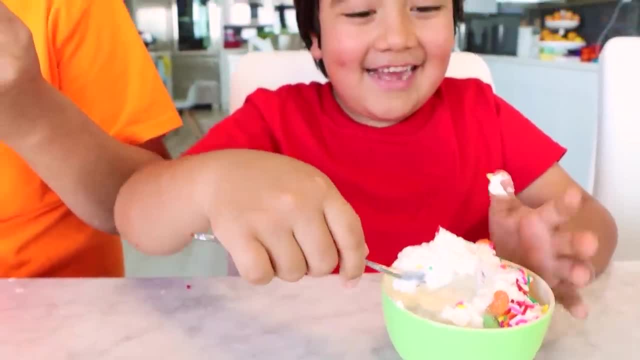 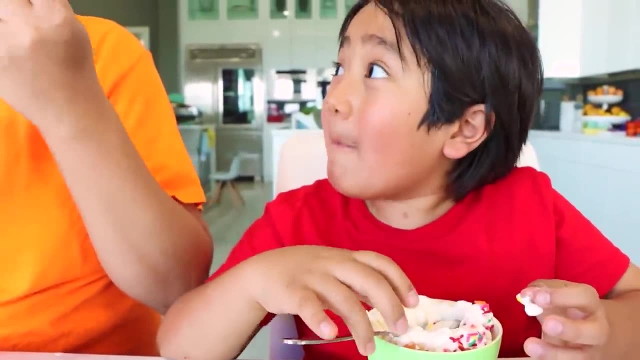 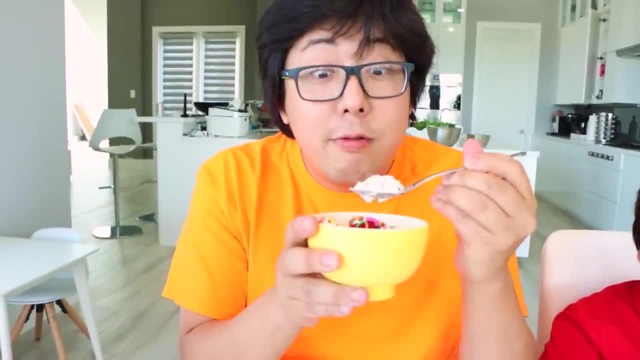 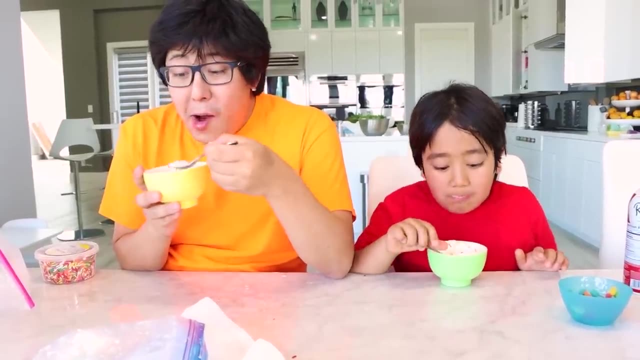 I think we didn't add too much sugar, so it's not that sweet, which is good, right, Good. A lot of times, ice cream is too sweet, Mm. But how does this work, Mommy? Good question, Ryan and Daddy. 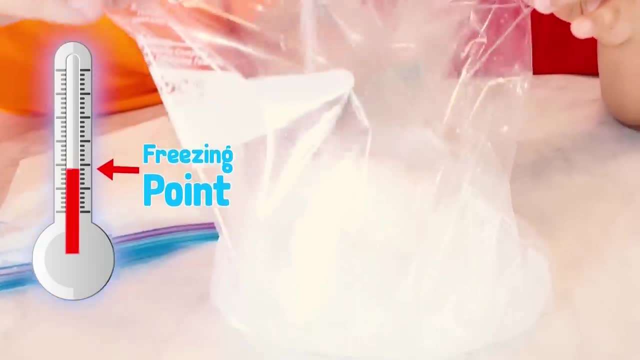 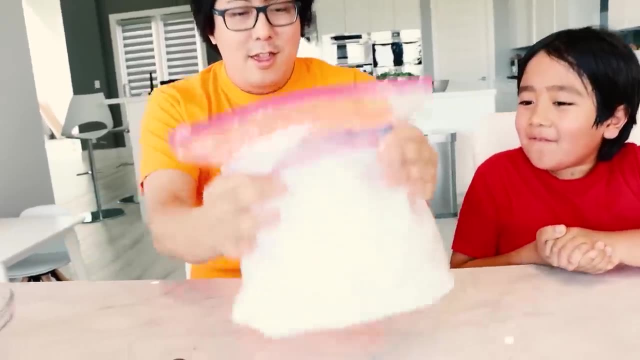 So when you add salt into ice, it lowers the freezing point of ice. okay, So if the freezing point of ice lowers, it has to melt, right? Well, in order to melt, you gotta get energy from somewhere. Where do you think the ice got its energy from? 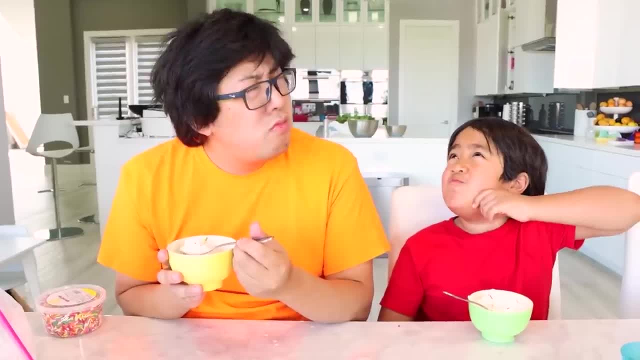 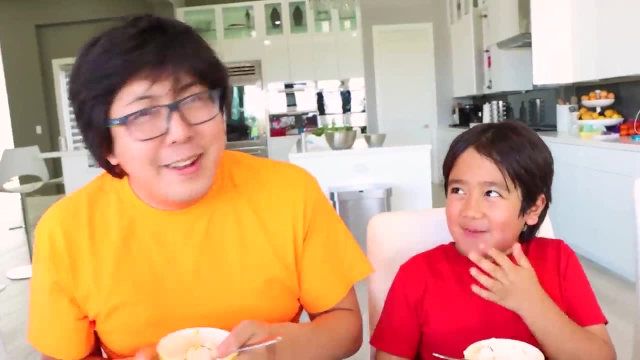 Hmm, Hmm, Hmm, Hmm, Any guesses, Hmm, Hmm, From the cream in the bag. Ah, I was going to say that, Yeah, Yeah, me too. In order for the ice to melt from the salt, the ice has to get energy from somewhere. 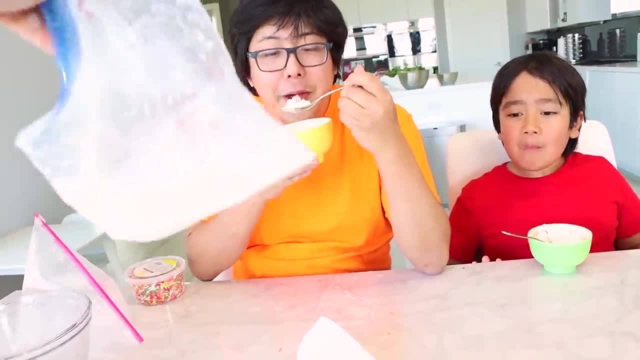 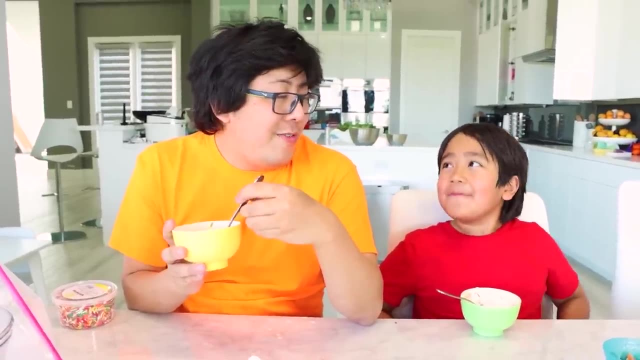 It takes this from the cream in the bag. So if you take energy away from this cream in the bag, it will freeze into ice cream. What do you guys think It's so cool? Yeah, Injabi, That's exactly why you know, during wintertime. 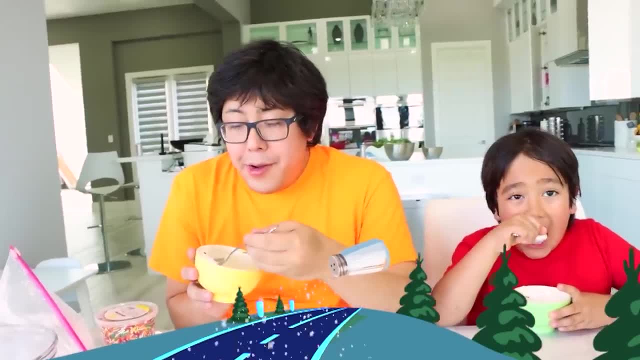 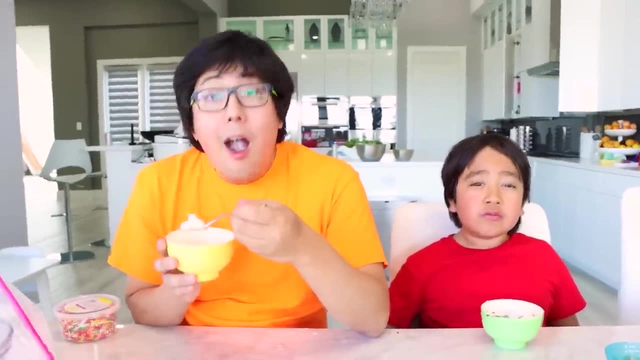 a lot of people would add salt to their paveway or, you know, in the ice outside their yard, You know, so they can drive. So it lowers down the freezing point of ice and the ice will melt, Mm-hmm. 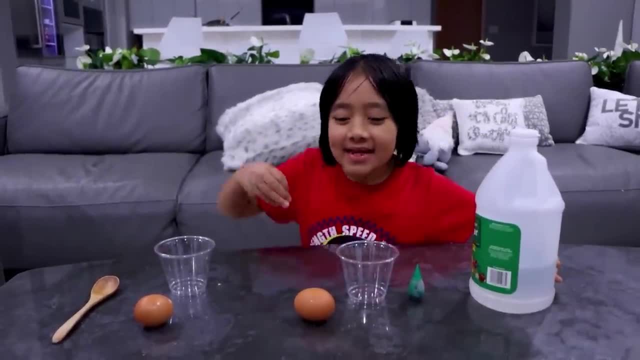 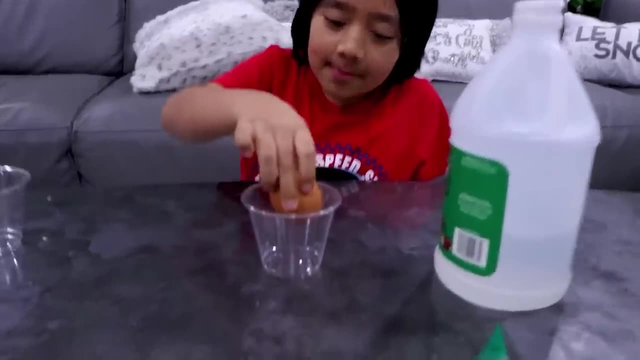 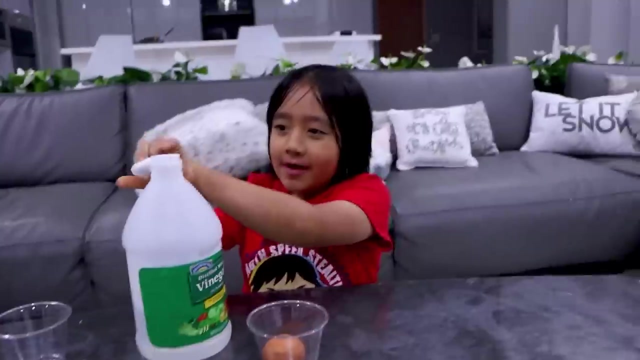 Yeah, Yeah, Hey guys. Today we're going to make bouncy eggs. All you need is an egg and some vinegar. First step: add an egg into the cup carefully. Next, add vinegar. Don't forget to ask a grownup for help. 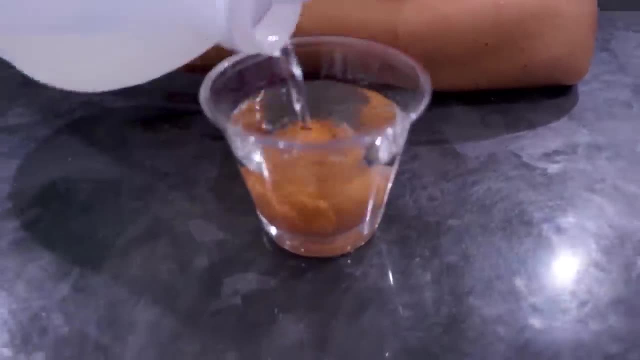 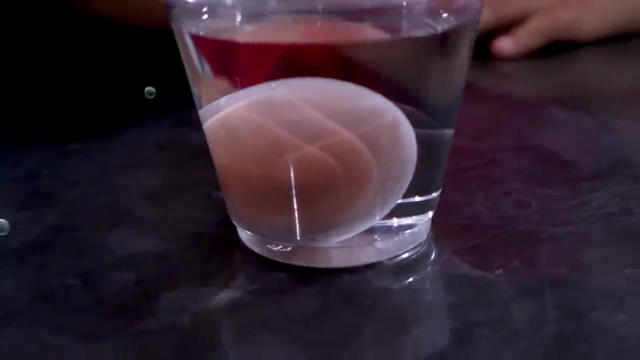 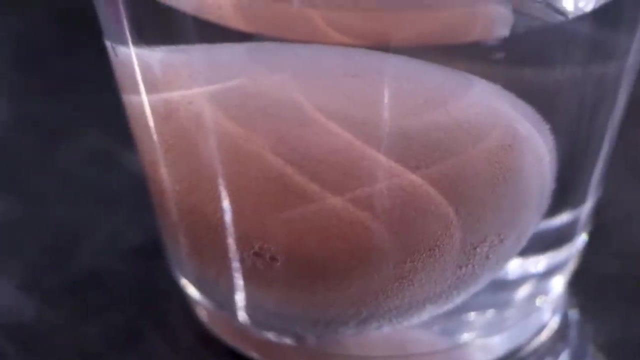 I'm here. Yeah, Guys, I already see bubbles, Oh, Oh. So the vinegar is trying to dissolve the eggshell And I see that happening in some spots. While that's happening, I'm going to do the same thing. 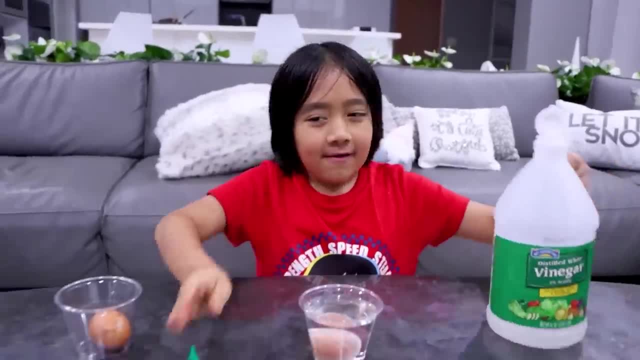 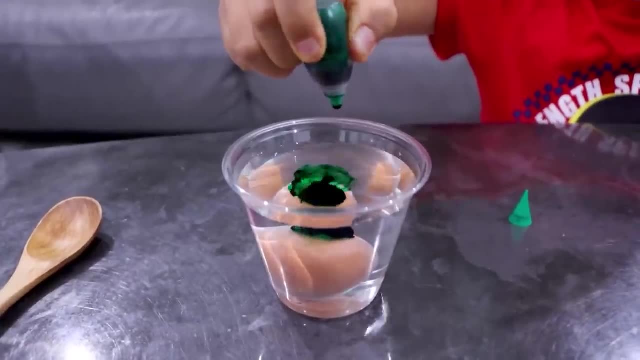 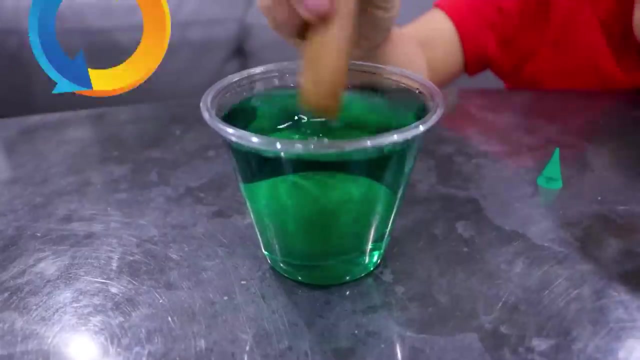 But I'm going to add food coloring to the vinegar There. Now I'm going to agitate the green food coloring. Ooh, Ooh, The egg looks green from the outside. I'm going to test to see if the green color is. 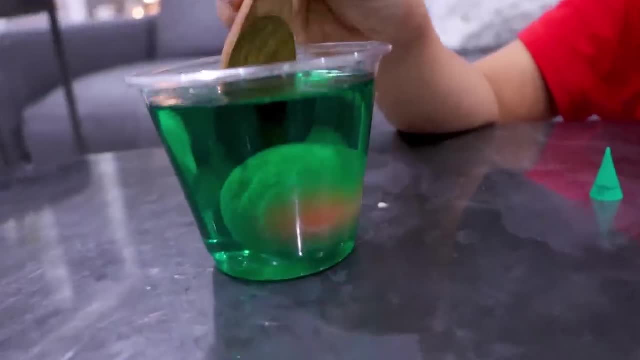 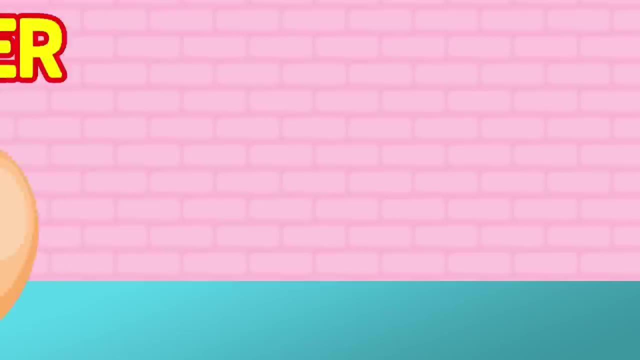 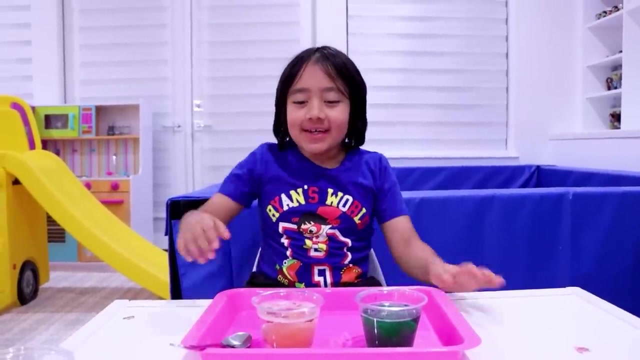 going to go into the egg, But if you put the egg super close, you can see that it's not green yet. Now we're going to wait for 24 hours, 24 hours later. OK guys, It's been 24 hours. 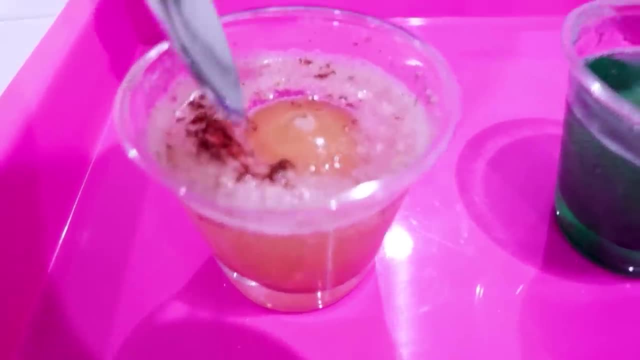 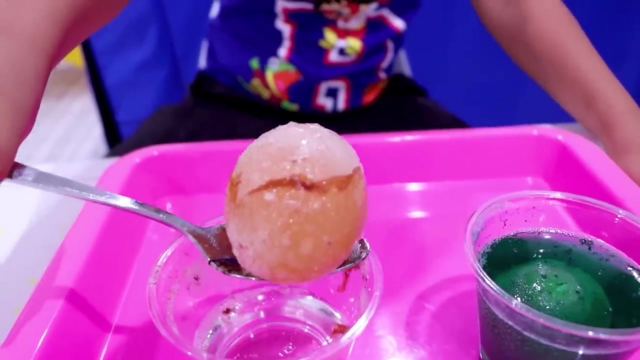 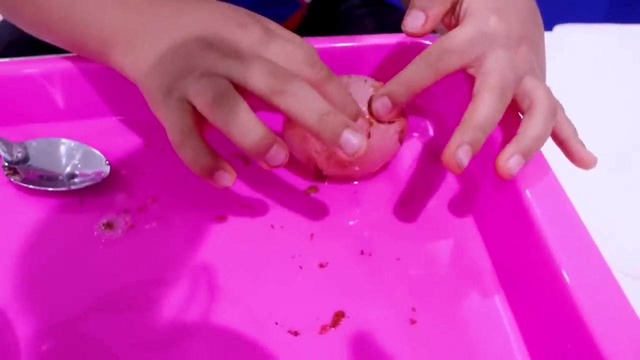 Now let's take it out. And here's all the shell. OK, OK, OK, OK, OK. Whoa, The shell's still here. OK, OK, OK. Or part of the shell, Bam, OK, I'm going to take the shell off. 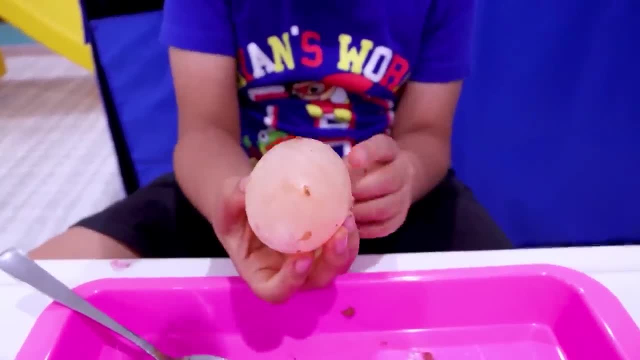 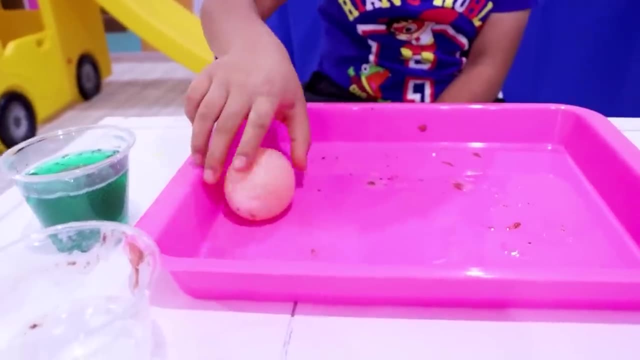 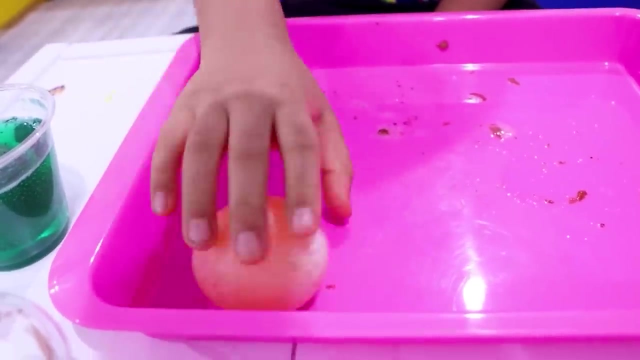 I can't believe it, guys. The vinegar dissolved the shell, Whoa, And it's a little bit bouncy. Look Whee, An egg without being in vinegar would maybe break from this. Now we're going to take out the one in green food coloring. 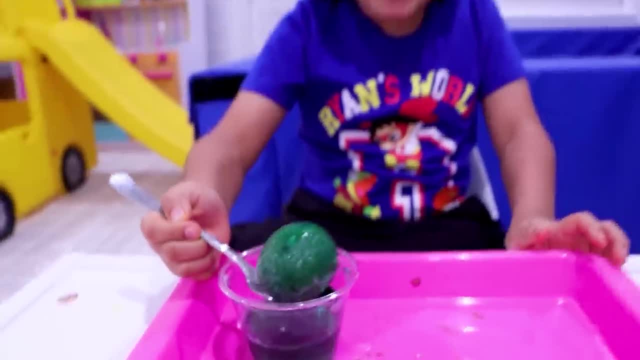 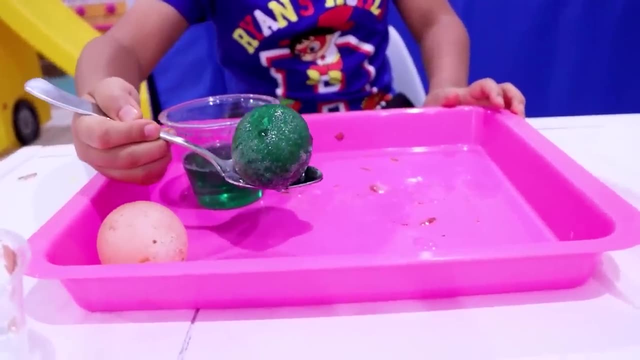 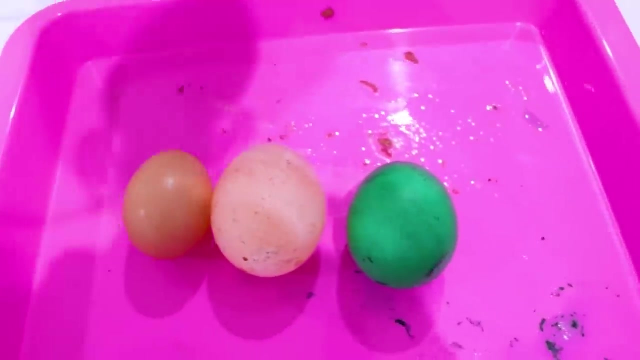 to see if there's a difference. Well, there's the difference: It's green. OK, OK, OK, OK, OK There. Look guys, Here's a normal egg And here's these eggs that were in vinegar. 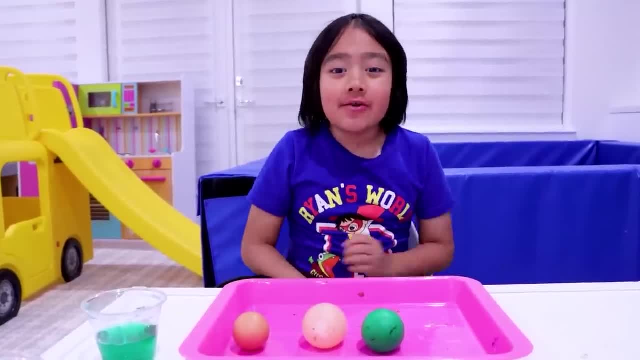 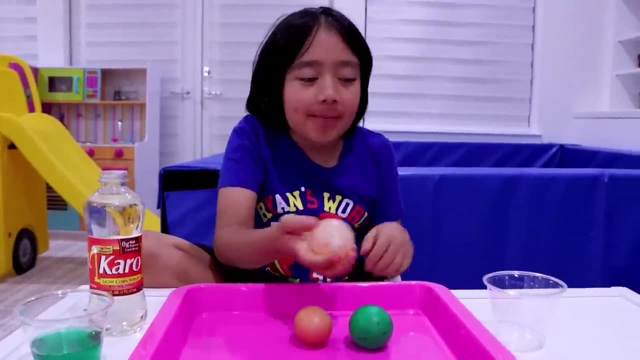 It's way bigger. It's bigger because the vinegar liquid went inside the egg And that's also why it's bouncy. Now we're going to see what happens when we put the bouncy egg into corn syrup. OK, Bounce. 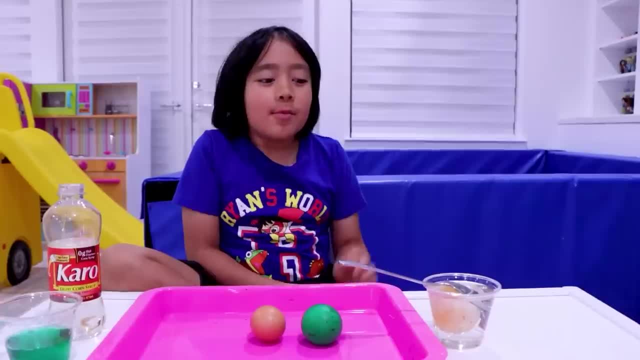 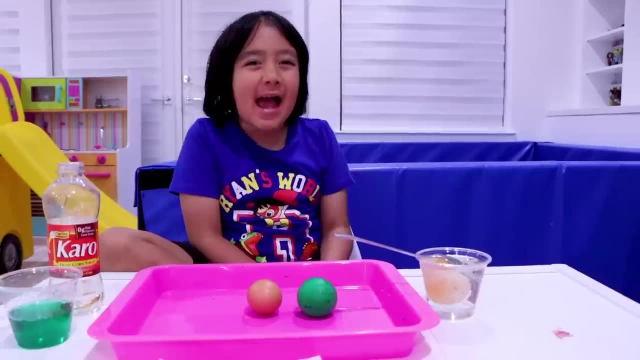 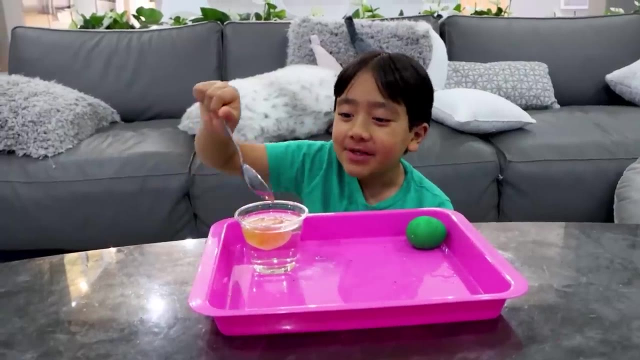 There, We put a spoon on top of it so the egg doesn't float up, And now we wait For 24 hours. That's a long time, 24 hours later. OK guys, It's been two days, So now we're going to take it out. 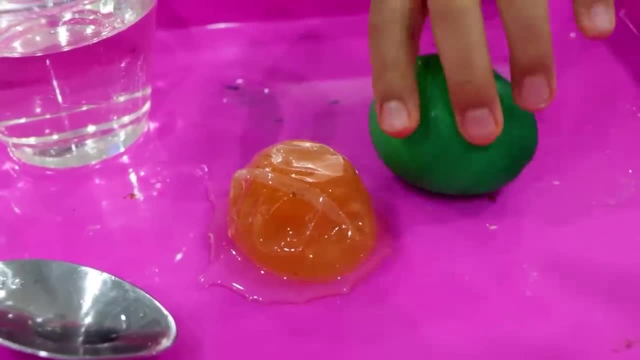 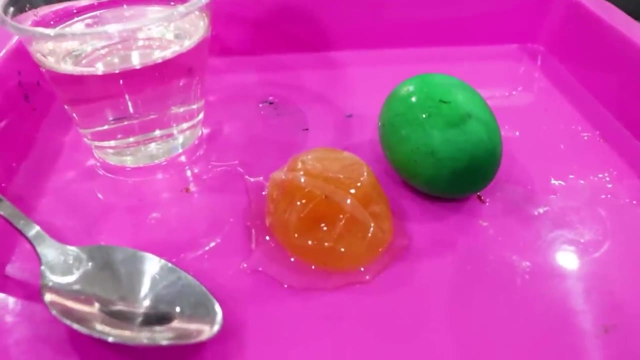 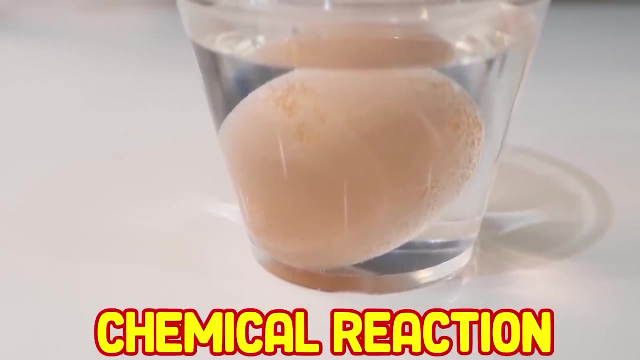 And look guys, Now it's smaller. Not that it's smaller, But it's also deflated because the water went out. Here's how it works: When the egg is placed in the vinegar, a chemical reaction takes place, producing carbon dioxide gas. 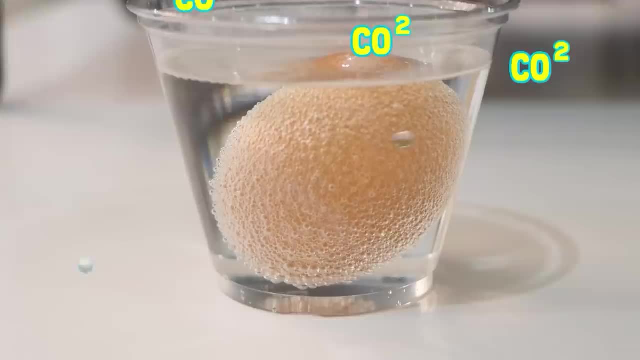 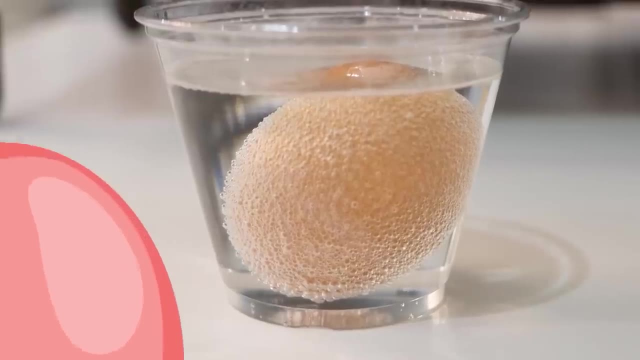 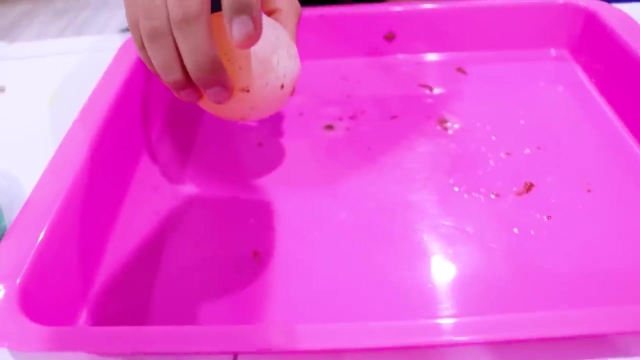 or bubbles. The vinegar, which is an acid, dissolves the egg shell. Once the shell is gone, what's left covering the egg is a thin membrane. The vinegar toughens up the membrane of the egg, making it bouncy Whee. 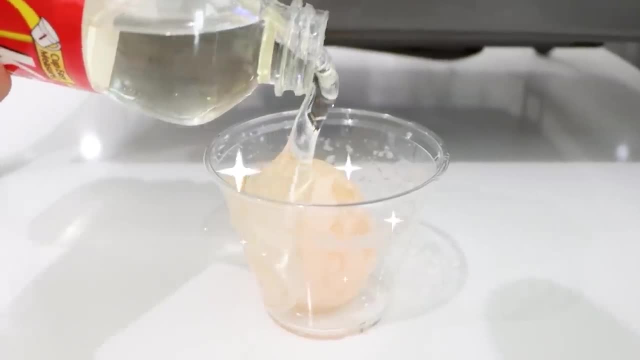 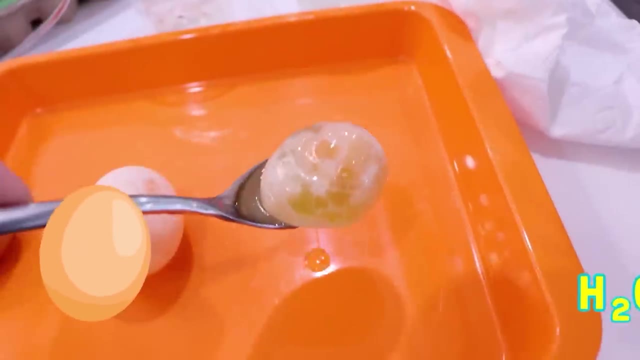 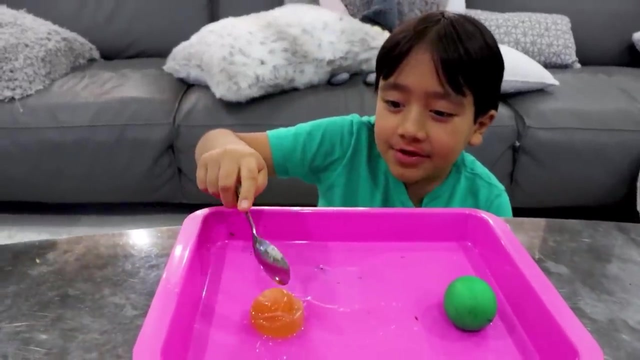 Then, when the bouncy egg is placed in the corn syrup, the water from the egg leaves the egg, So it appears to shrink. OK guys, Now I'm going to see what's inside the egg, But remember to not do this without an adult. 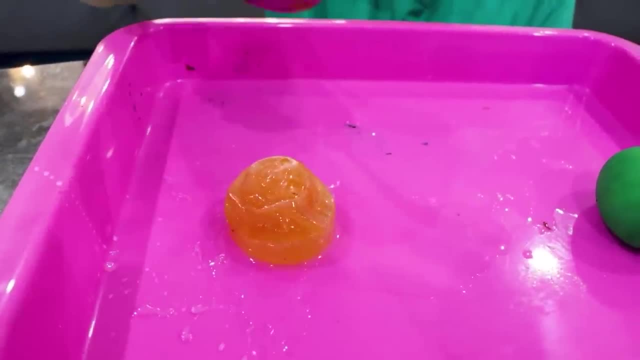 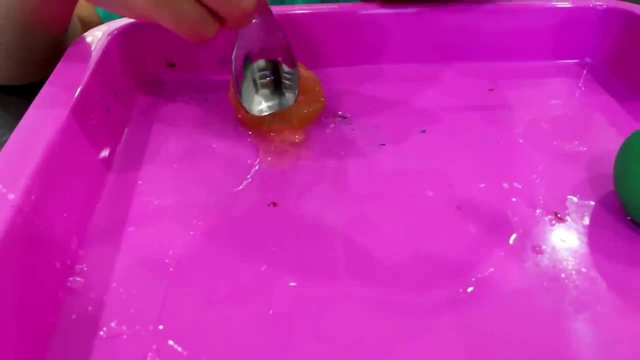 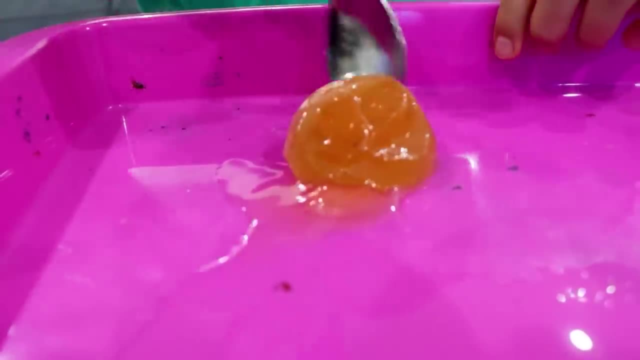 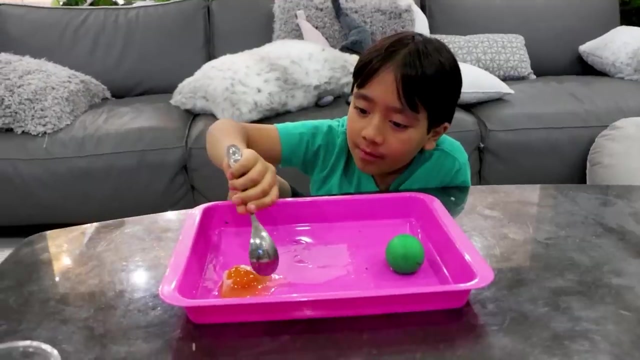 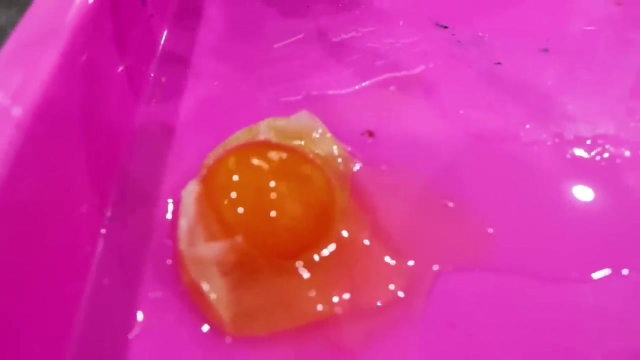 Ooh, ooh, Oh, oh, oh. OK, let me lift it up. If I can lift it up, I will lift it up. OK, there you go, There you go, Oh, OK, Whoa, It's orange. 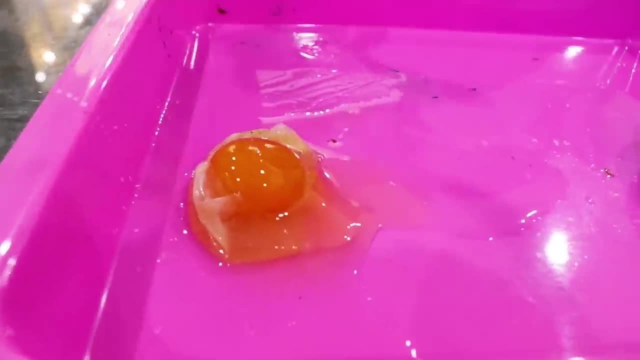 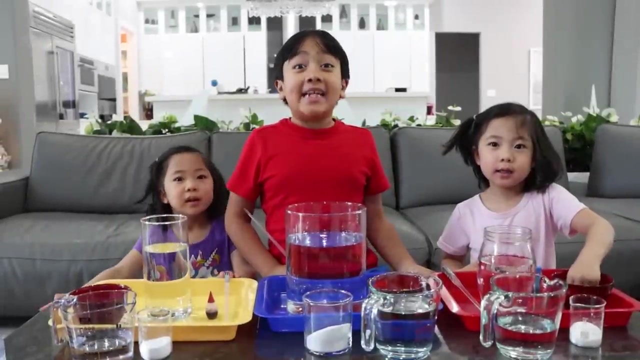 The yolk is still there. Oh, oh, oh, I got it. Hey guys, Today we're going to do the dancing popcorn experience. OK, so first you need a jar of water And then you put the popcorn in the water, like so. 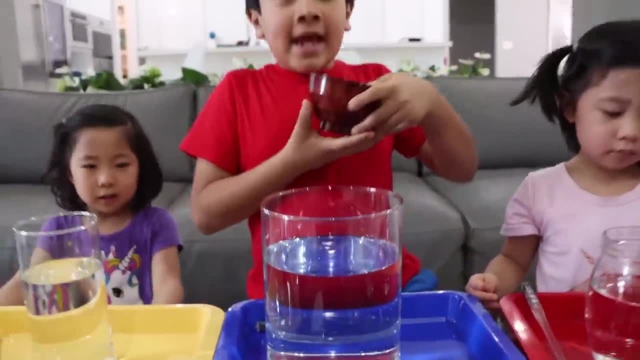 Wow, the kernels sink. Do you know why The kernel sinks to the bottom? because they are more dense than water. OK, do you guys see that the popcorn is dancing already, or not? No, Yeah, popcorn does not dance with just water. 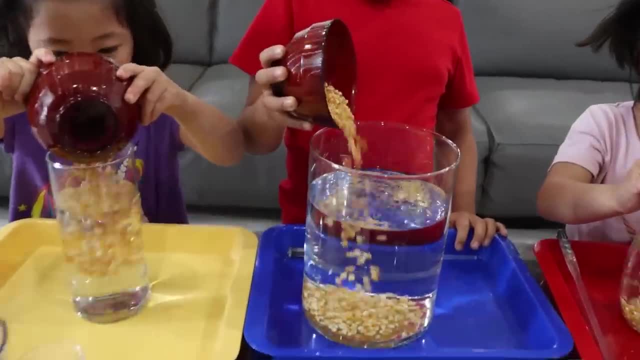 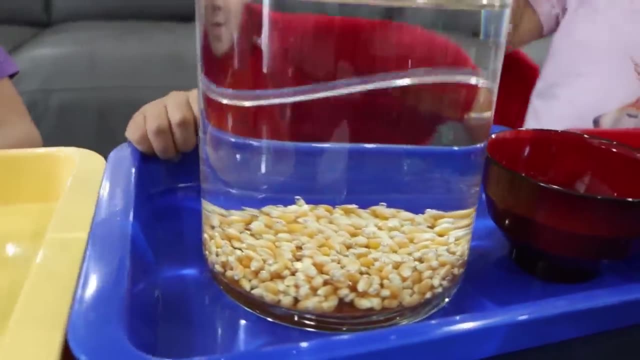 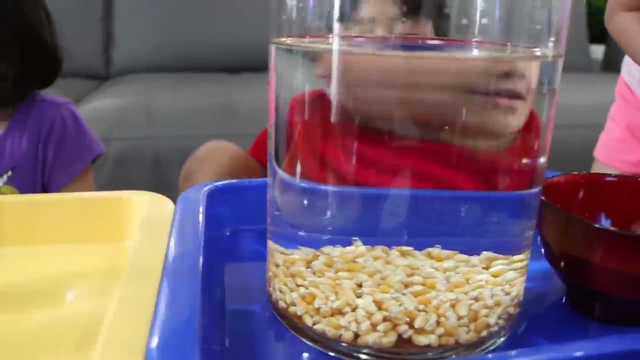 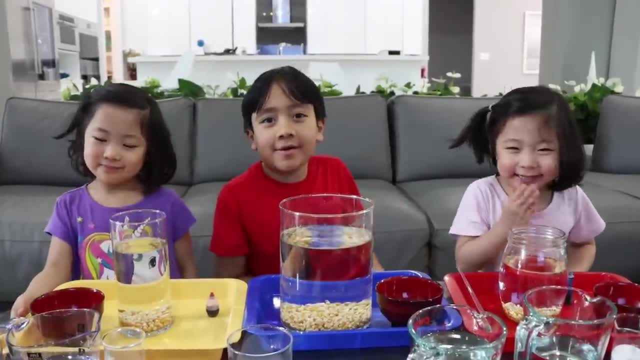 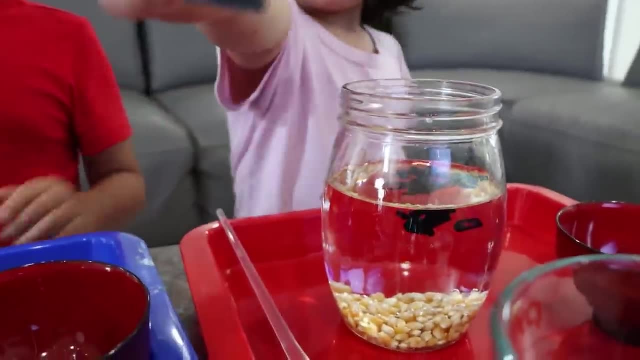 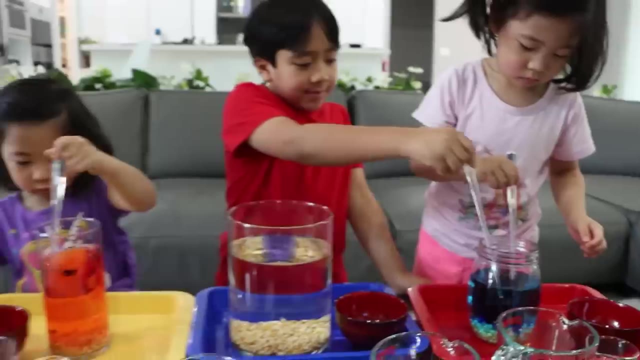 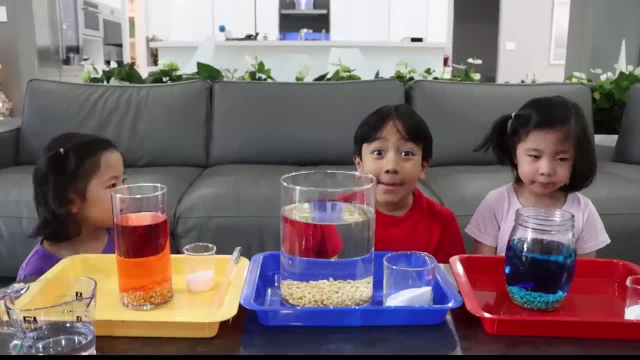 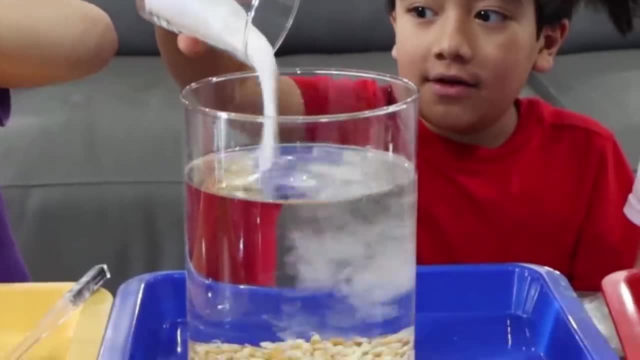 levar. check Darina, because no to me. OK, OK, OK, OK, OK, OK, OK, Right, this Ryan's adding- yeah, Ryan's adding- two cups of baking soda, Emma's adding one, Because mine is bigger. 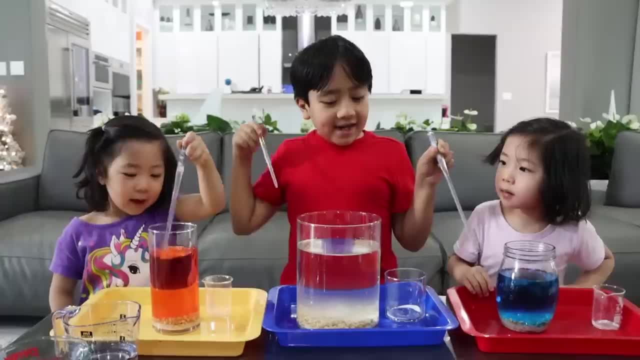 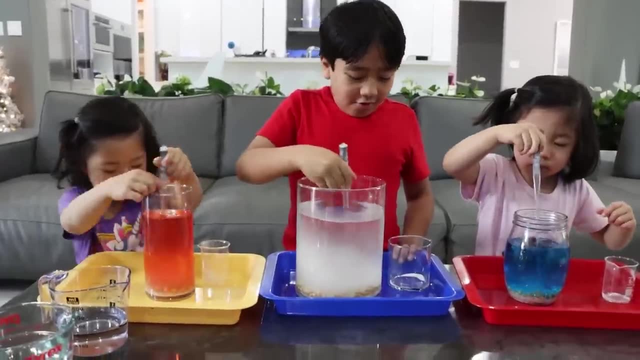 That's right. There you go, It's a buggy. Next, we've got to agitate. That's right. What's another word for agitate? Mix, Mix. That's right. To stir, to mix. Why is it so white? 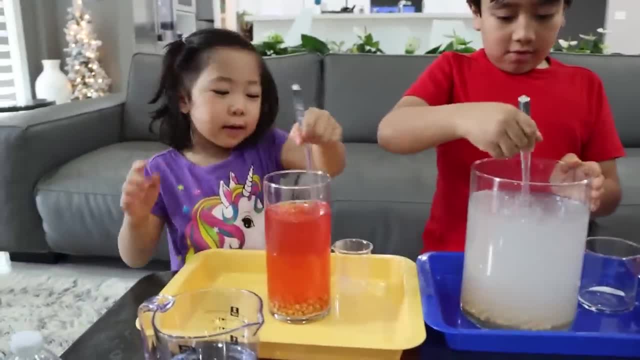 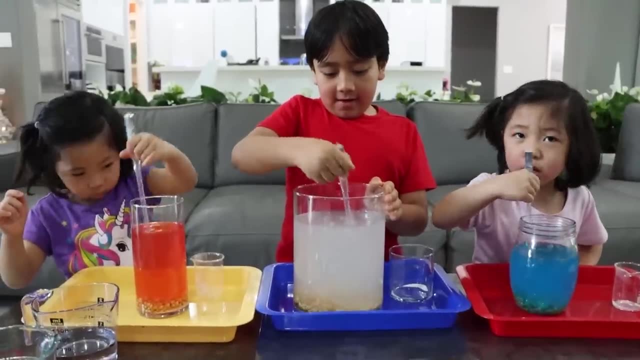 Emma's agitating, Everybody's agitating. I already done that. I made a small whirlpool. Oh, that does look like a whirlpool. It's like my whirlpool. It's like your swimming pool. Yeah, you're right. 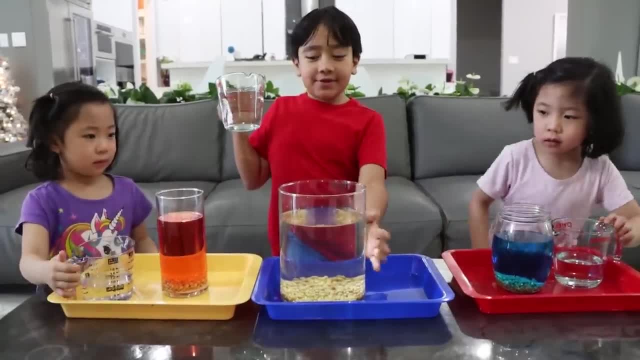 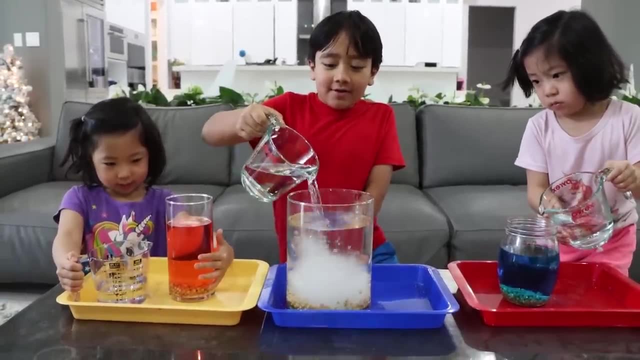 Next up is the vinegar. So if you do something like this, use two cups. If you're doing something like these, then use water. That's right. Might be a little bit of explosion. Go, Explosion, explosion, Whoa. 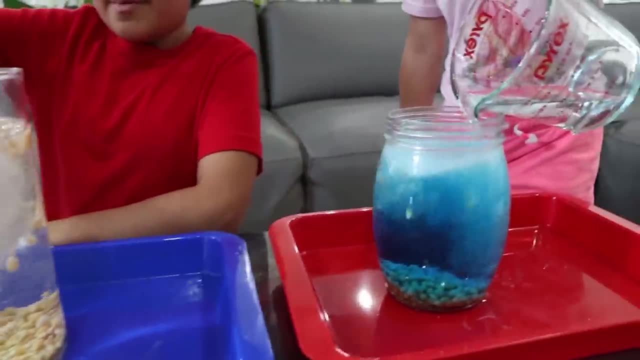 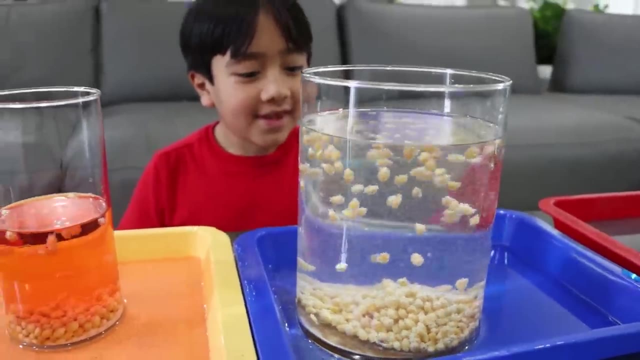 They're moving around. They're just going up and down. They're a little bit more. Mine's not moving. Mine's not moving. Do you see, Ryan? do you see how the popcorn is dancing? Yeah, And I can make it dance more by spreading it. 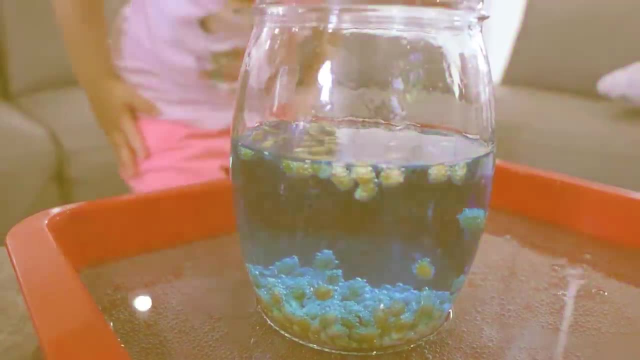 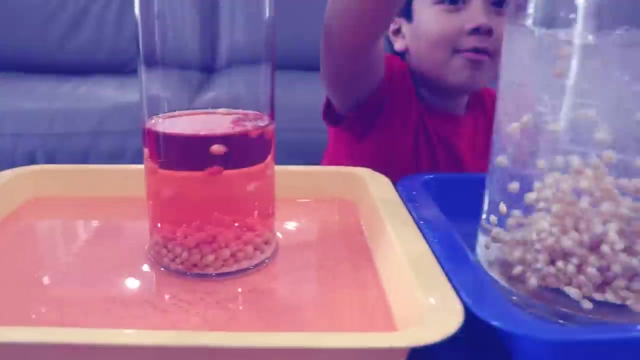 Emma's too. See it, You guys saw. you see, Emma, do you see how yours is going up and down? Look how many of mine. look how many is dancing? Ryan, it looks like we're tornado. Yeah, Tornado of popcorn. 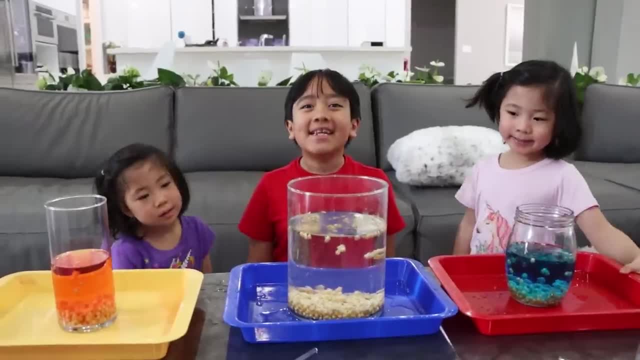 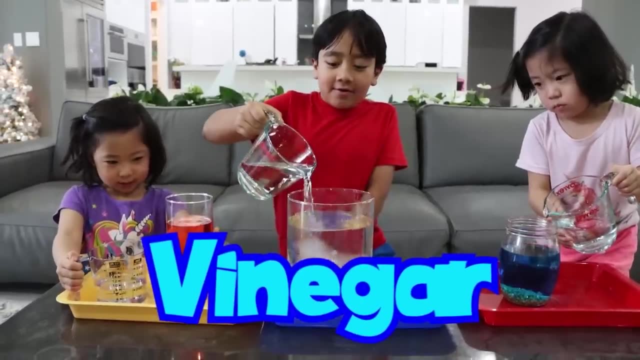 And Kate, yours is too. Look, Kate, see, it's going up and down. You want to use mine, Emma? Okay, guys, here's how it happens. So when you mix baking soda, which is a base, and vinegar, which is an acid, 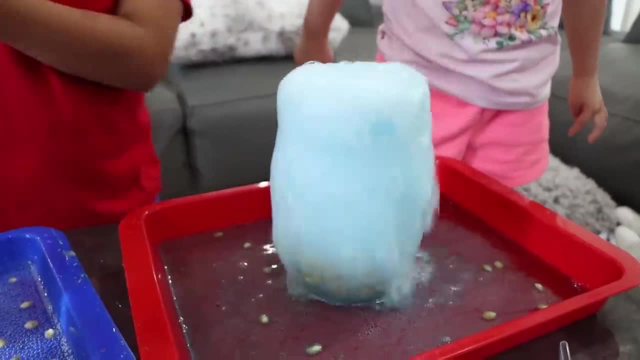 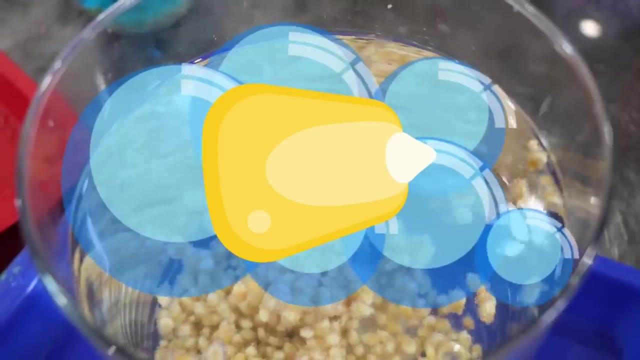 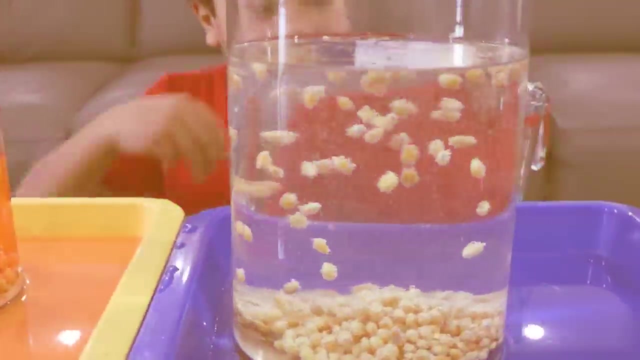 a chemical reaction takes place, Carbon dioxide bubbles are produced, which are the bubbles that you see lifting the corn to the top. Once the bubble pops, the corn falls back down, And this happens over and over again, so it looks like the corn is dancing. 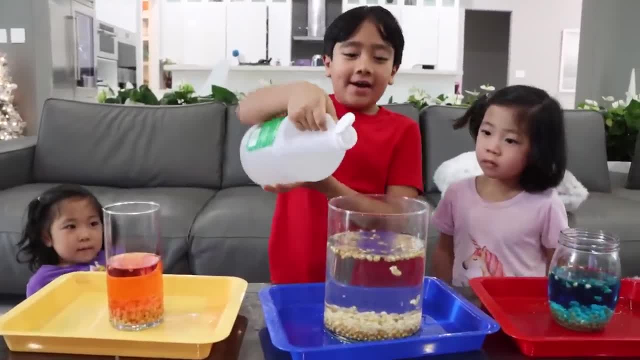 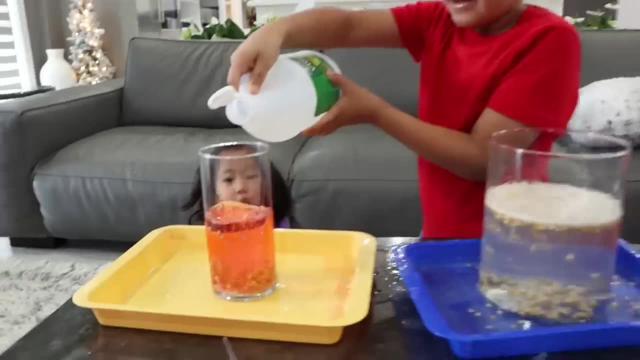 How cool is this? Now we're going to add some baking soda and vinegar for fun. So first we're going to add the vinegar. Whoa, Whoa, whoa, whoa, Whoa, whoa whoa. I didn't know that would happen. 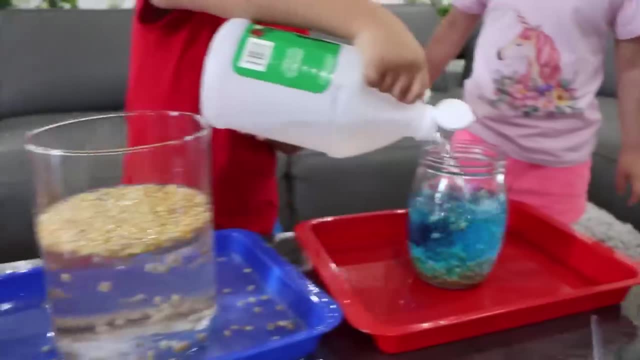 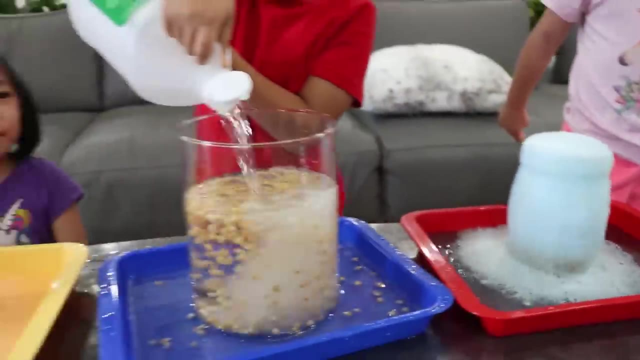 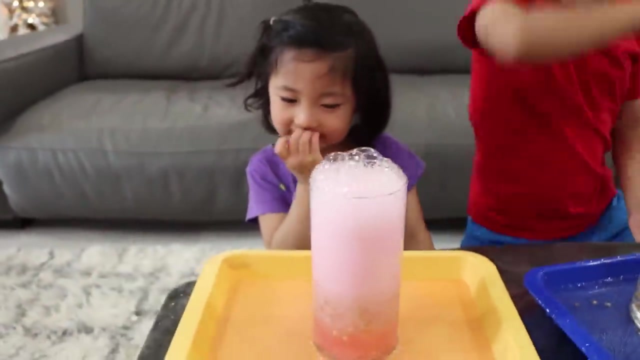 Whoa, Whoa, Here we go. Whoa, More, more, more, Bam, More, more, more. I want more of mine, More Whoa Mine exploded. so much at the first one. Look, almost all of them are at the top. 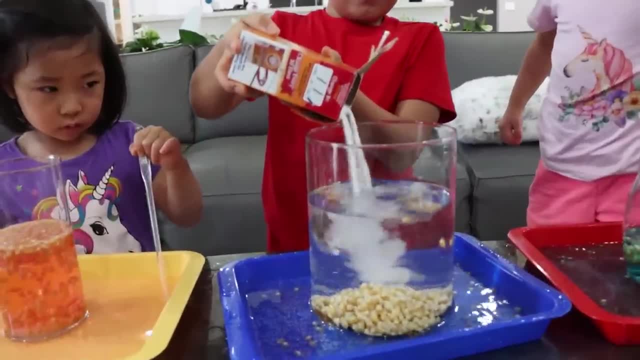 Okay, I'm going to add in some baking soda too. Okay, okay, maybe like that much. I don't want to do it myself, I don't want to do it myself. Okay here. So you guys all see the bubbles and fizz and carbon dioxide gas forming. 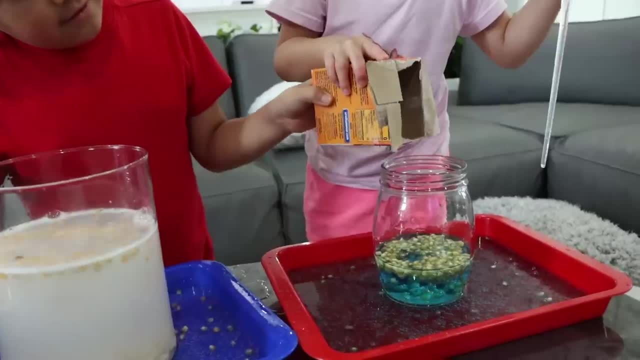 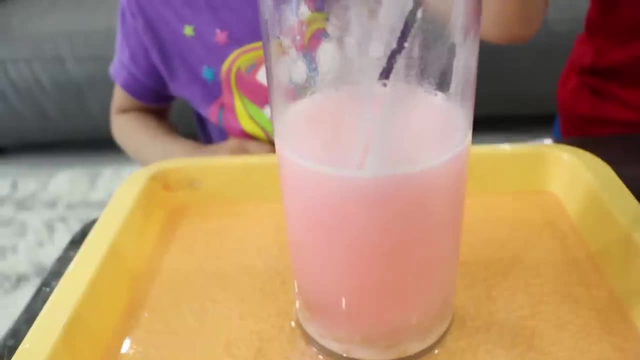 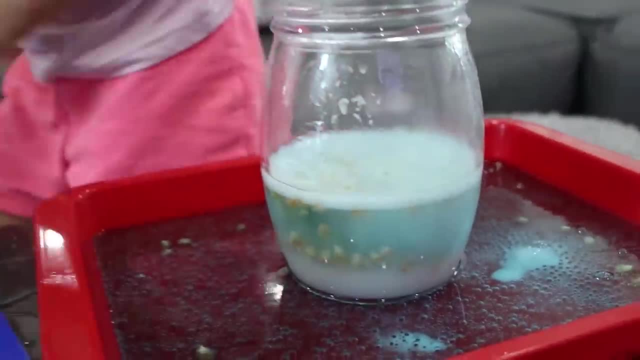 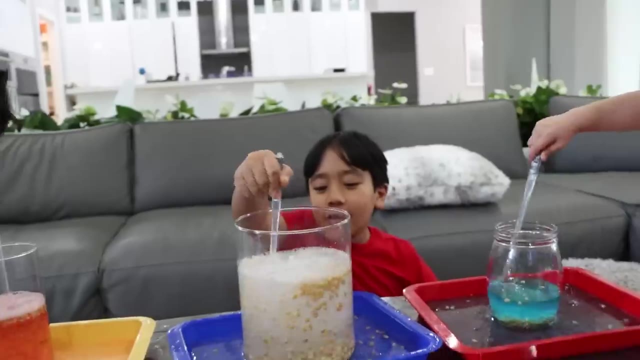 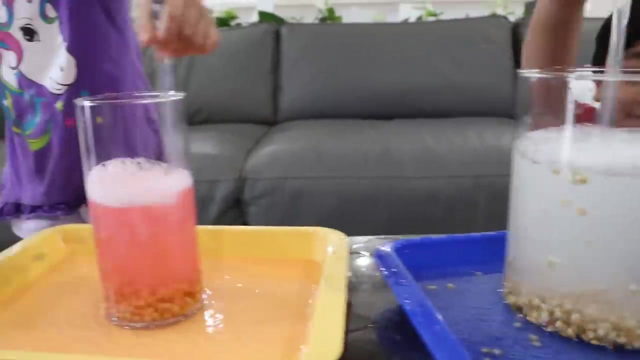 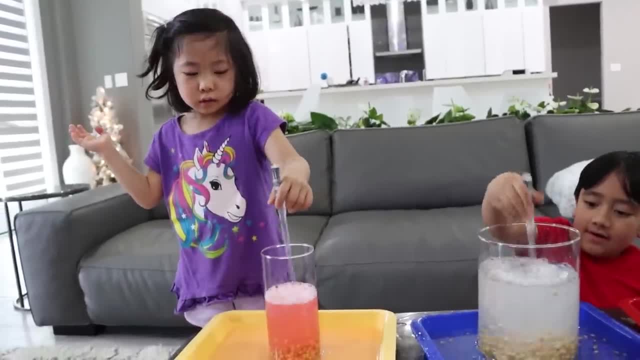 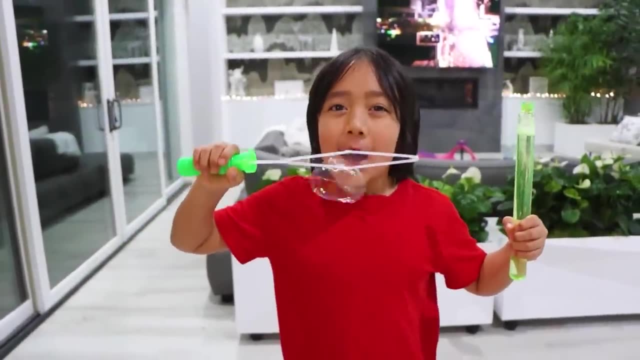 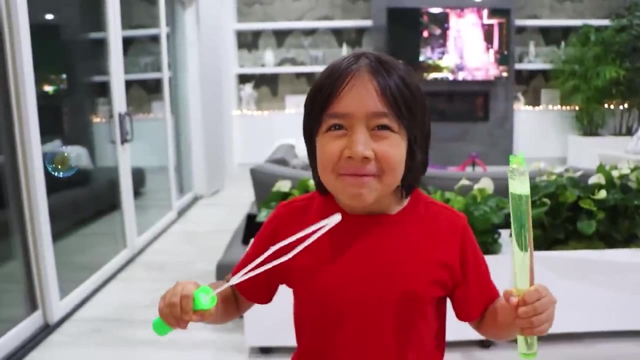 Is Colonel Tornado real mommy? Yeah, Do we get it in action right now. Oh, Ryan, That's cool. Hey guys, are you tired of bubbles that always pop? Oh, Today I have a solution for you: Non-popping bubbles. 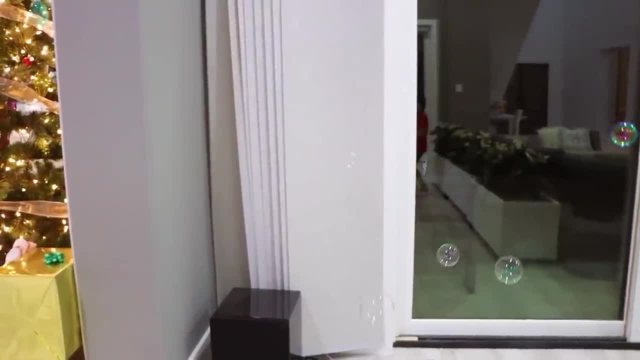 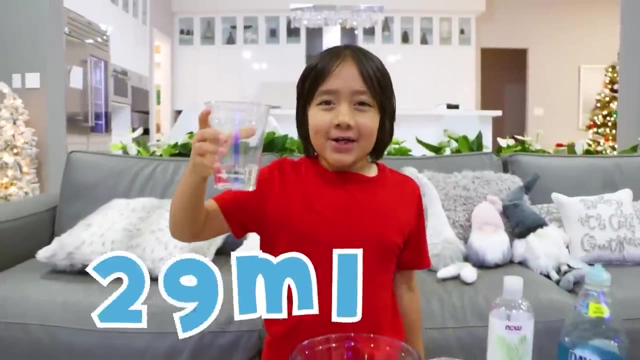 Let's go. Hey guys, today we're gonna make bubbles that don't pop, but always ask a parent for help. So first you need 100 milliliters of water and then 50 milliliters of glycerin. 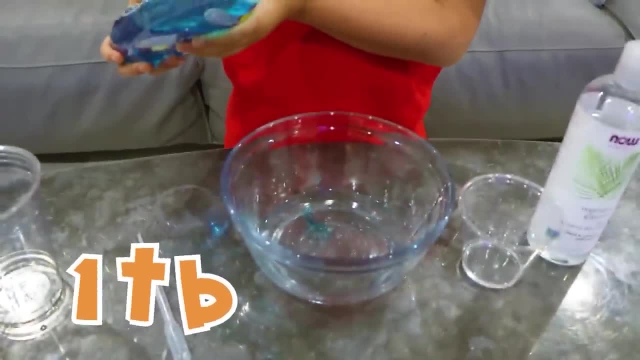 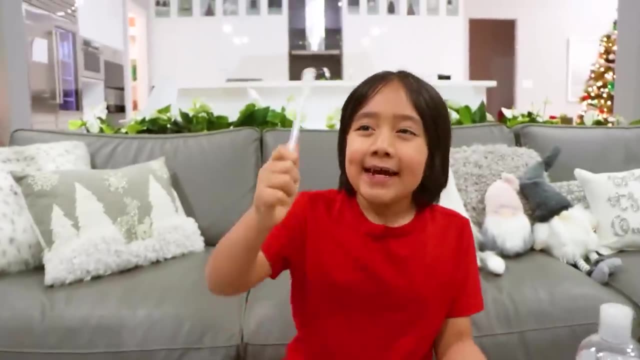 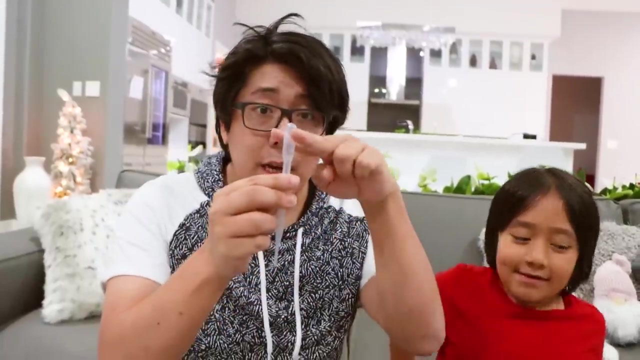 and a squirt, or one tablespoon of Dawn soap. Next let's agitate. or another word for mix. Next, get a pipette and cut it right here. I'm gonna ask my daddy to help me. Hey, Ryan, All right, so we're gonna cut right here. 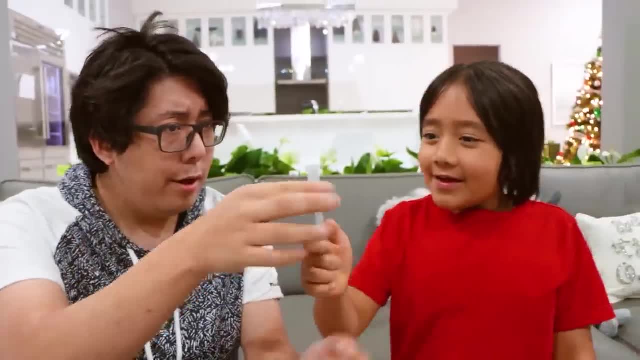 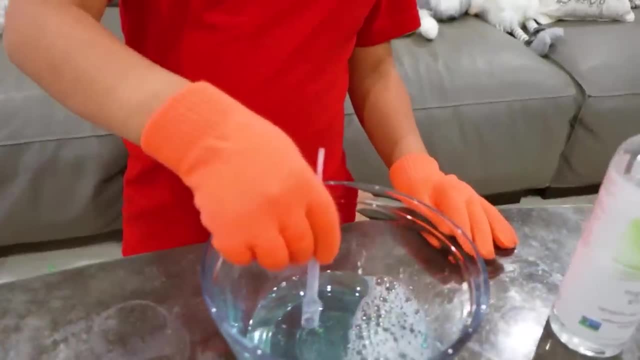 All right, I'm gonna cut this for Ryan Boom. Is this what you wanted? Yeah, Next you need some woolen gloves, and then you take the pipette, dip it in the water and glycerin, and then 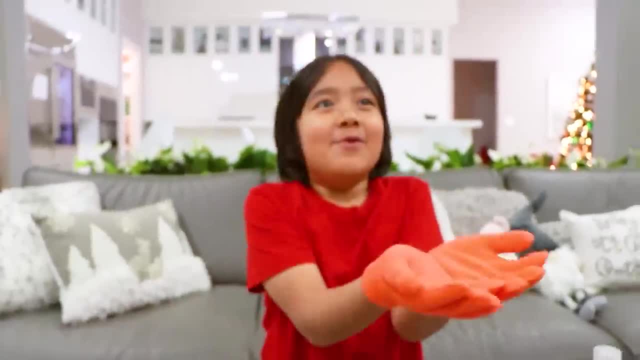 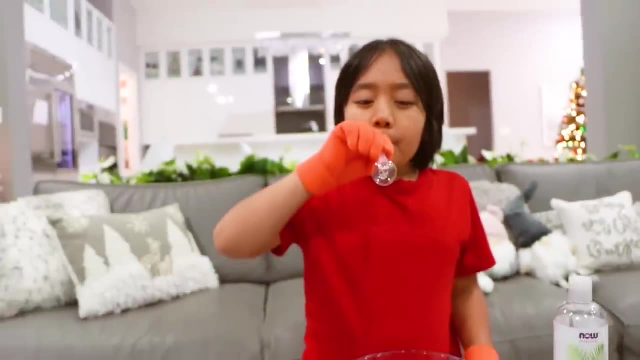 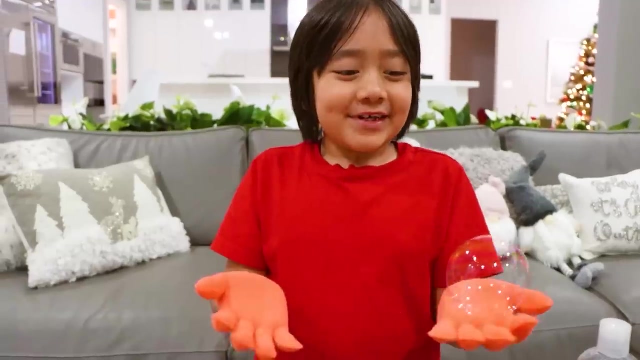 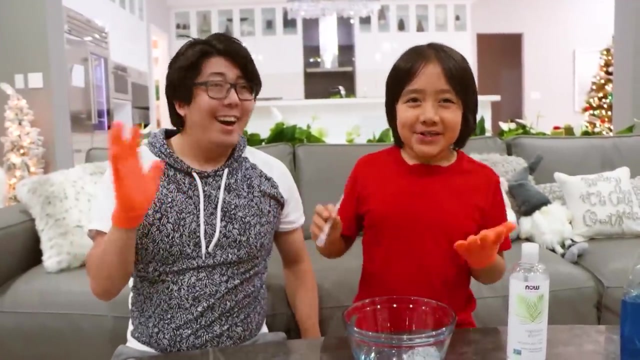 There you go. Let's try that again. Okay, guys, we're gonna see until it pops. Oh, it already popped. Now me and daddy are gonna throw the balls to each other until it pops. Whoa, whoa. Okay, Stop popping. 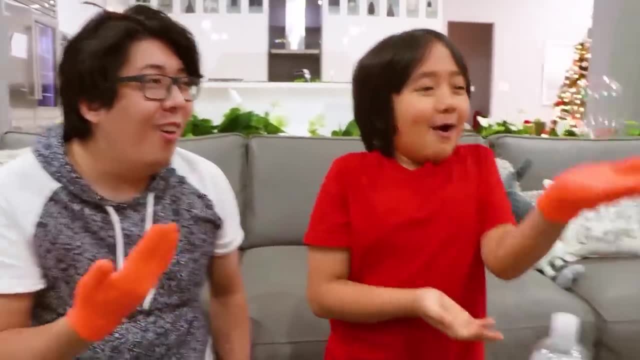 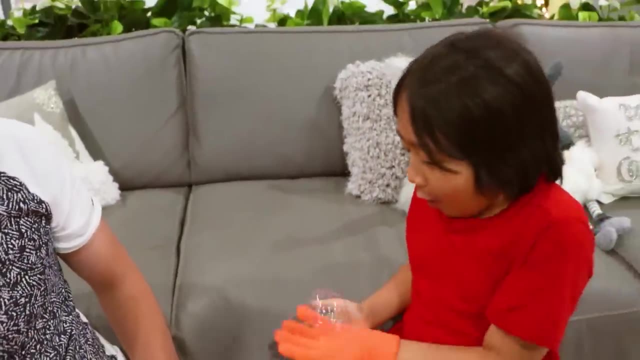 Stop, Whoa Whoa. it's bouncing. Whoa whoa, whoa Whoa, oh oh, Whoa, oh no, I almost tread my real hand. Yeah, make sure you use your glove Whoa whoa. 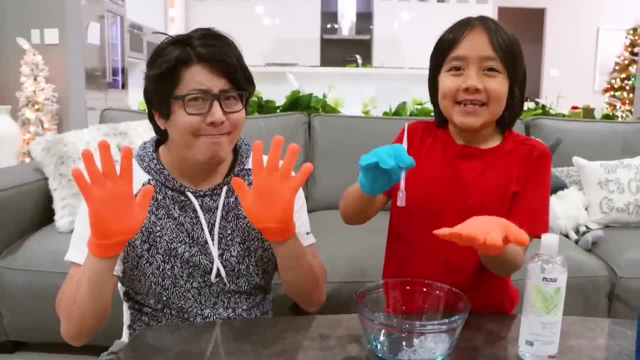 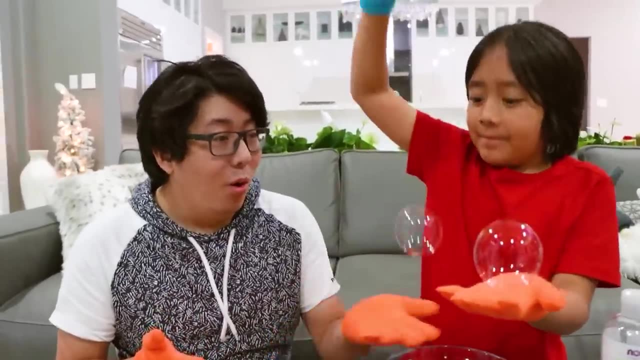 I popped: Okay, guys, now I'm gonna make a bunch of bubbles and I'm gonna see how much me and daddy can hold. Gonna break the world record. Whoa, Whoo, Oh, whoa, whoa, Whoa, come here. 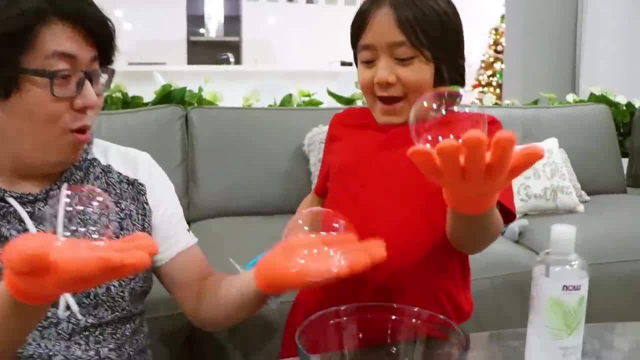 Oh, the balls adapt. Woo, Whoa right, Whoa Ryan, that's huge. No, But it bounced on your tummy. It bounced on my tummy. Can I put it together? Oh, Oh, Oh, Did you guys see it? 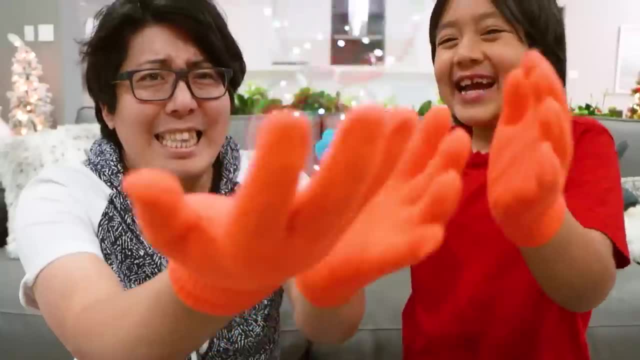 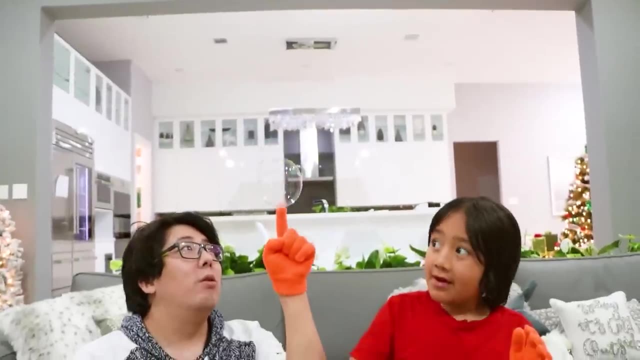 It became one. Wait, so can we combine ours? Yeah, Oh, never mind. Oh, no, It's running away. Huh, Ah, it popped. Ah, Or you can just bounce it with your Oh, never mind. 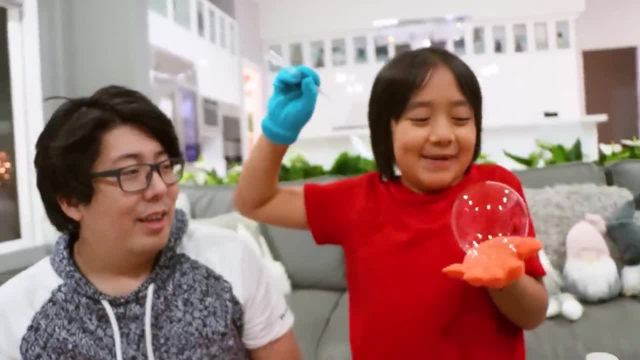 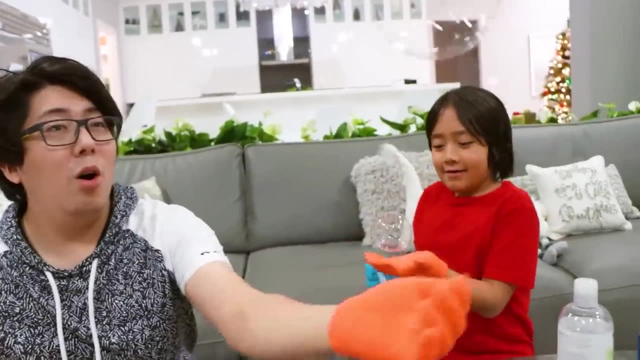 Oh yeah, Oh Well, Zeddy made a giant one. Nice, Here you go. Oh, Whoa, Whoa, Whoa, Whoa, Whoa. Can I throw mine at yours? Yeah, Let yours pop. 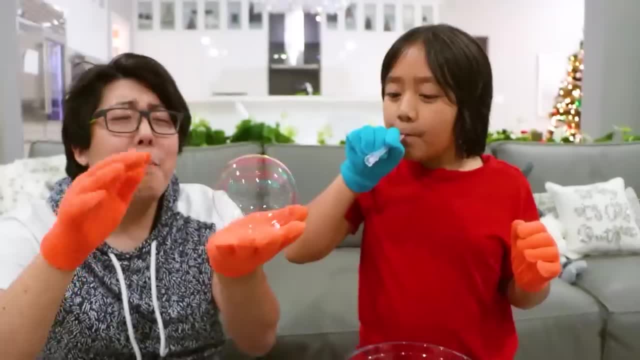 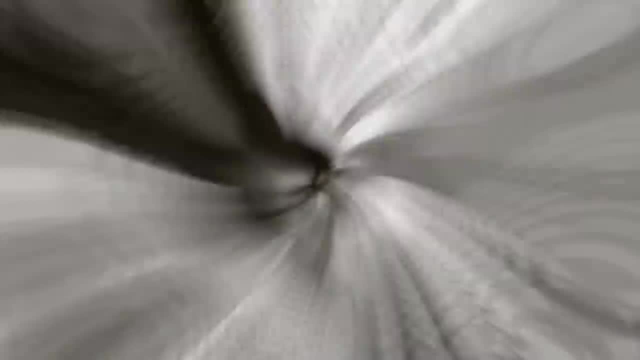 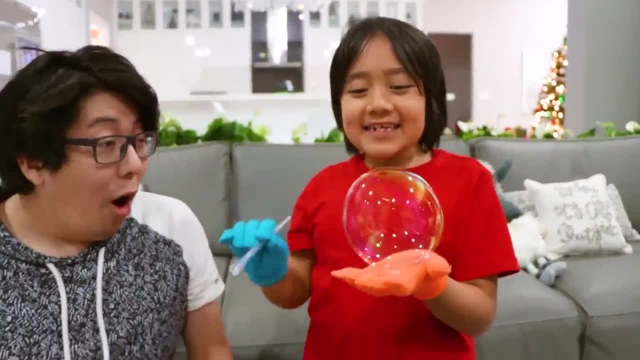 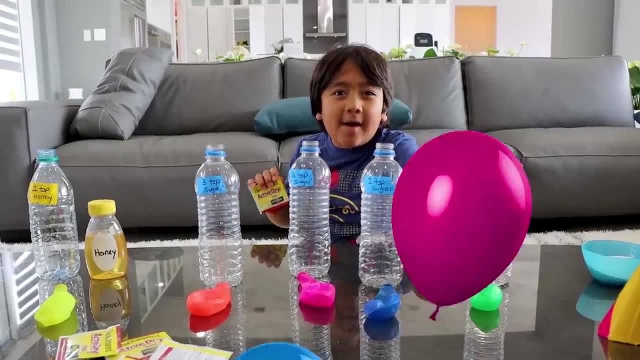 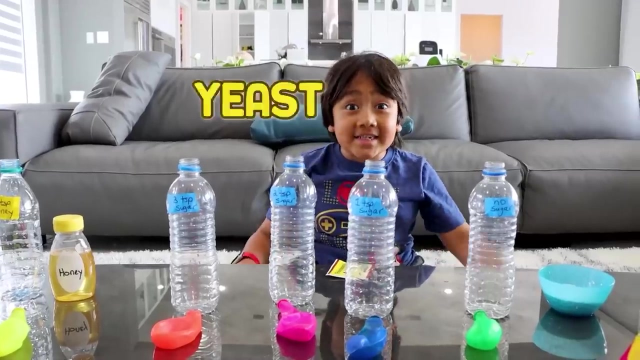 Oh, Oh, Okay, guys. so that's how you make a not-popping bubble. Hi guys, Today we're going to do the balloon blown up by yeast experiment. First, we're obviously going to need yeast. Did you know that yeast is a living organism like us, and we can activate them using sugar? 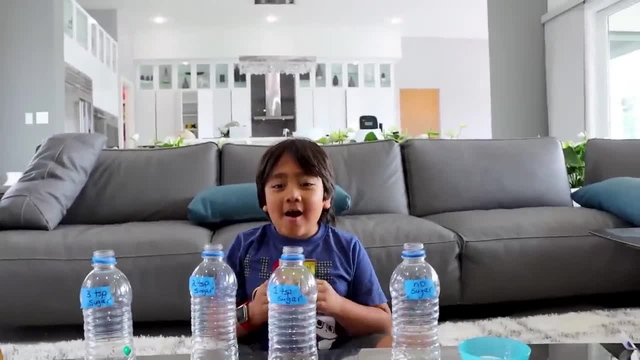 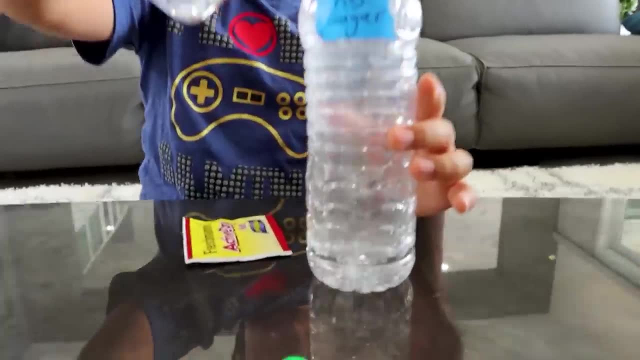 Yeah, so we're going to do an experiment to see how much sugar we need to blow up the balloon, Okay, Okay, so fill the bottles with one inch of warm water. Perfect, Now, it's an inch. Now let's do the other bottles. 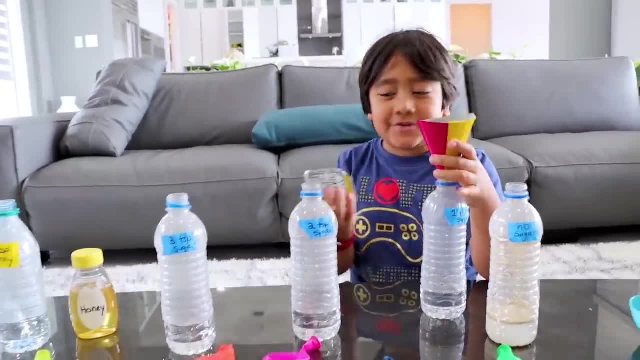 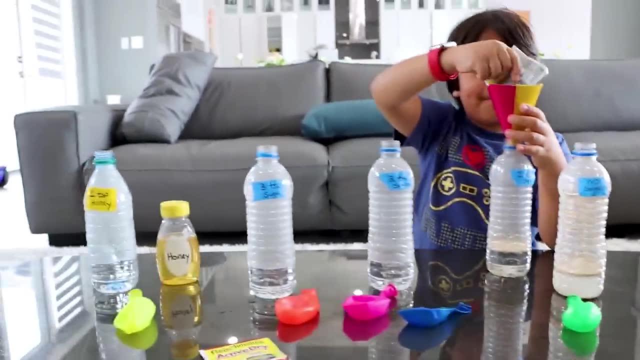 All right, we're going to keep going and add the yeast to all the bottles. Oh, A lot more yeast, Yeah, so we actually have used five bottles. The reason why is this: one: we're going to have no sugar. one teaspoon of sugar. two: 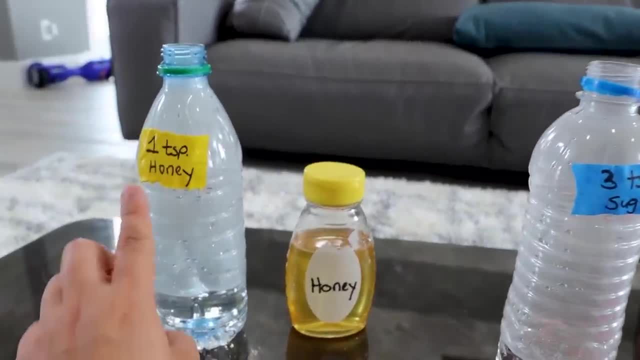 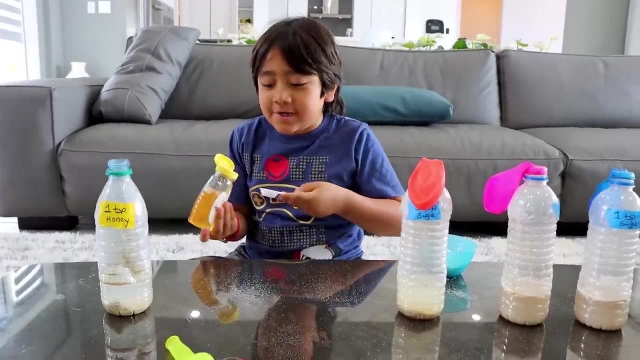 teaspoon of sugar. three teaspoon of sugar And this one. instead of sugar, we're going to use honey. Yeah, to see if it works and how much of a difference it makes. Over here, we're going to use honey instead. 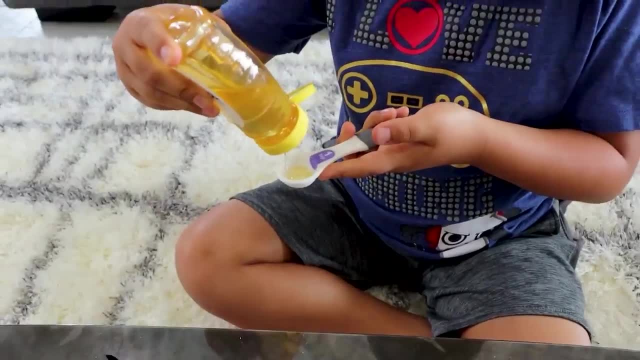 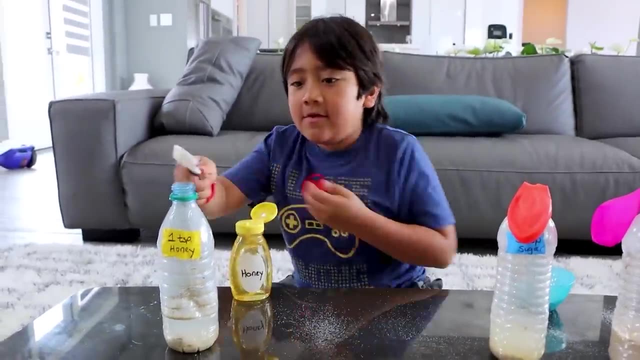 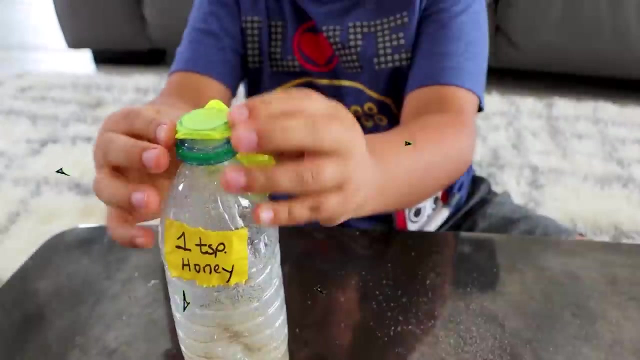 Yeah, we're going to use one teaspoon of honey. Whoa, this is a lot of honey. You think that's one teaspoon? Mm-hmm. Okay, It goes down. Okay, let's put this on. There you go. 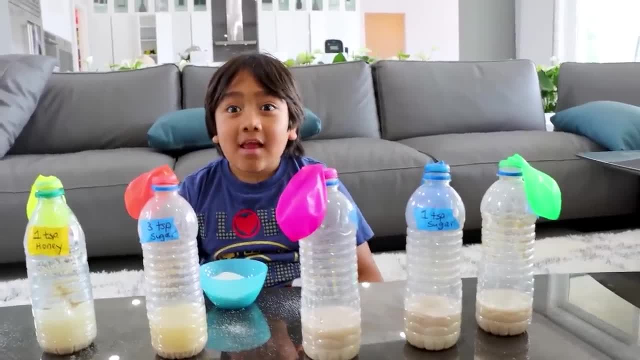 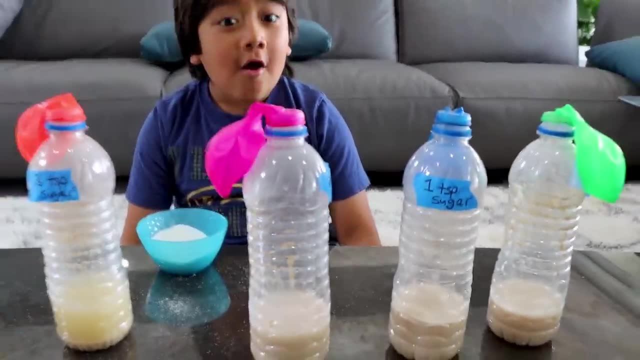 Okay, Yeah, Yeah. so Baker, also put yeast into the bread and the bread will rise, just like how the yeast will also rise up this balloon. Okay, Okay, Whoa, Whoa, Whoa, Whoa. look Ryan. 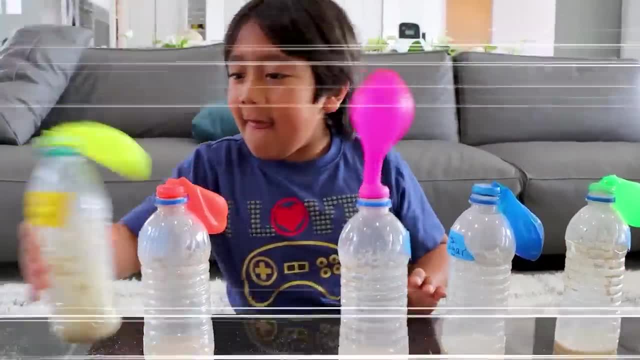 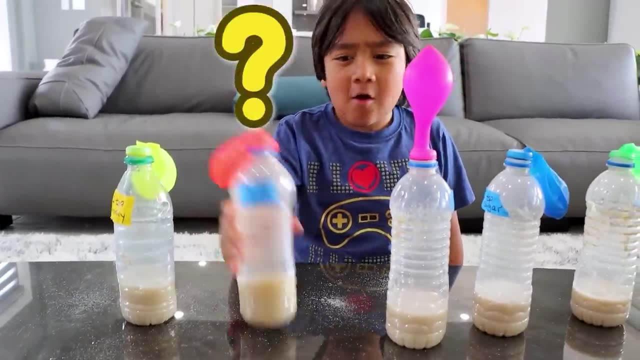 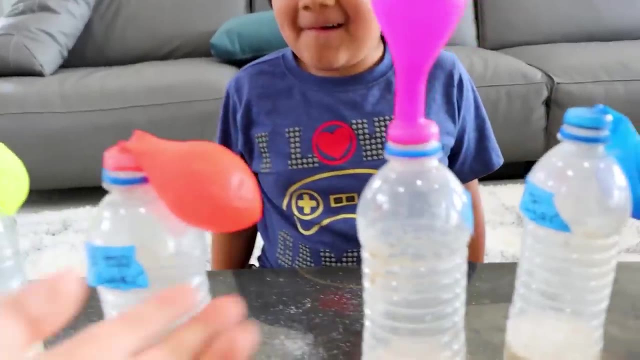 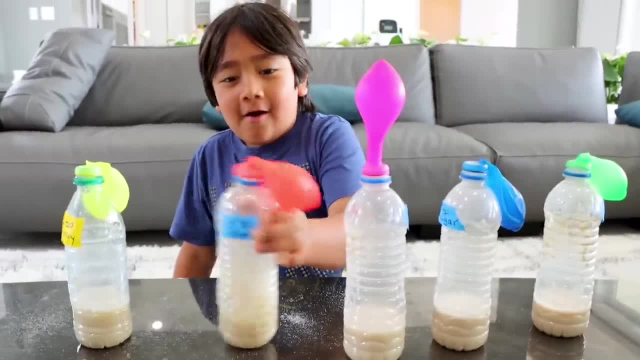 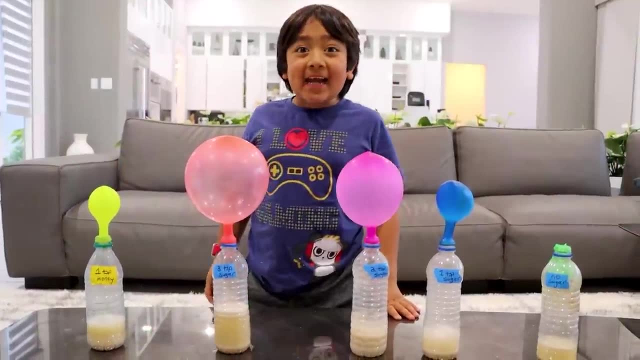 It's starting to. Maybe it just takes more time. Yeah, I guess we'll find out. All right, We will be back. Yeah, One hour later. Hi guys, now we're back. All of the ones with sugar and honey worked. 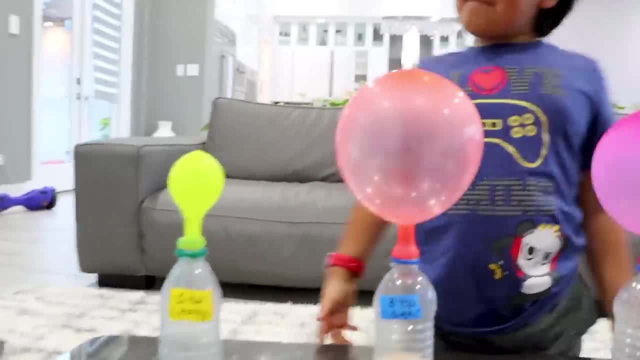 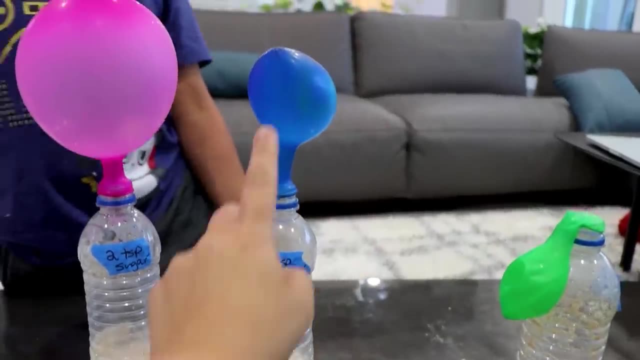 Yeah, Actually, what do you? One worked a little bit, Yeah. so what did you notice, Ryan? So the one without any sugar did it work? No, No, The one with one teaspoon of sugar worked a little bit. 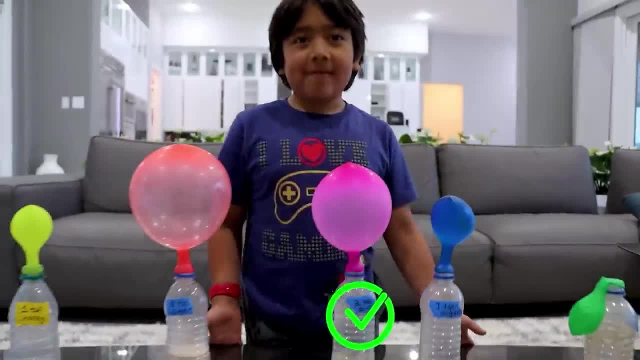 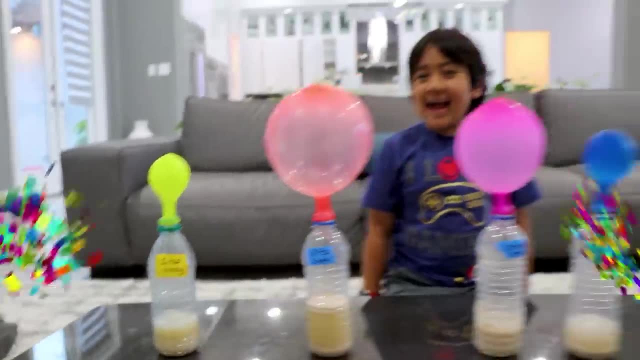 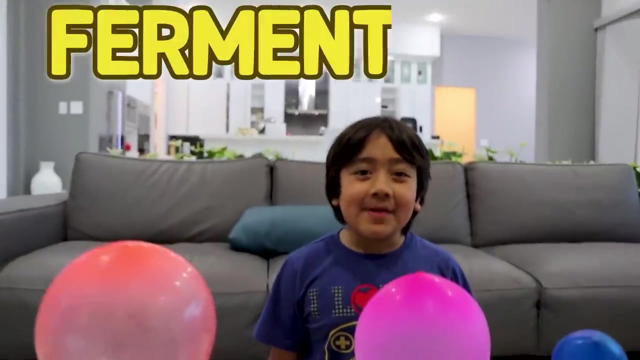 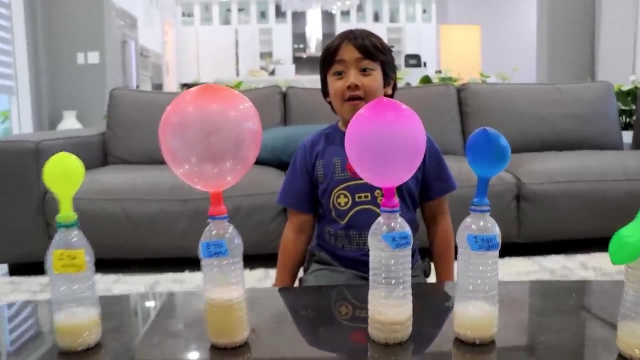 Yeah, teaspoons of sugar. it's a little bigger, yeah, and the one with three is even bigger, yeah. so did honey work? yeah, yeah, so there it is. so this process is called fermentation. can you say it fermentation? fermentation, that's right. so the yeast feed on the sugar, and then what came out of it? what's in here? gas, gas, what kind? 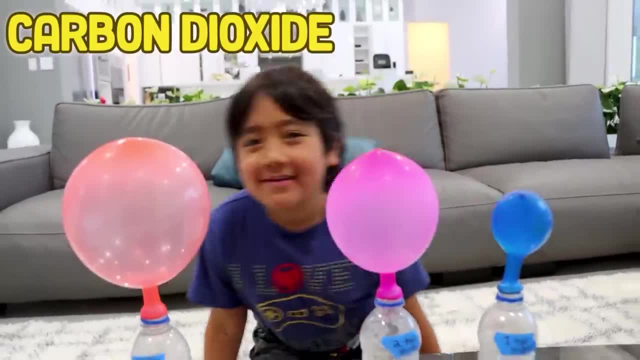 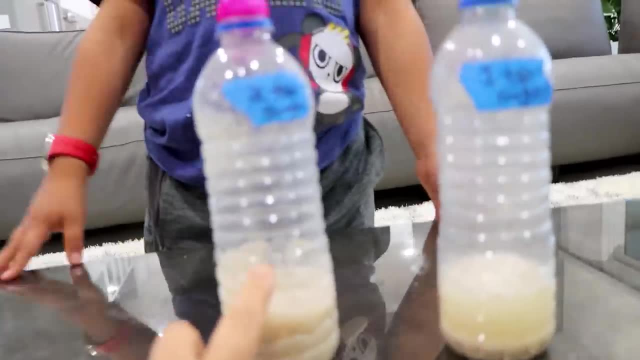 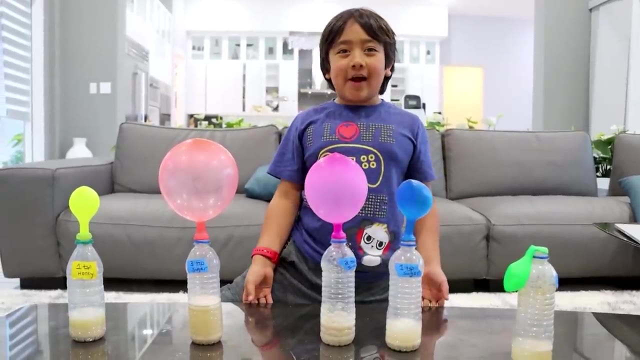 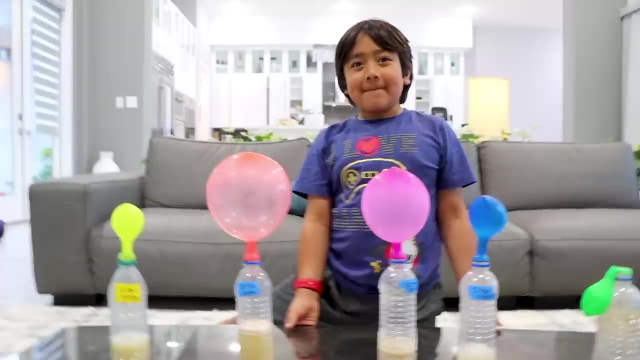 of gas. yeah, carbon dioxide. carbon dioxide gas, that's right. yeah, it also releases an alcohol called ethanol, but ethanol stays down here and the gas goes up into the balloon. maybe you guys should also try this out. but instead of one teaspoon, do like one tablespoon. yeah, lots of honey, right? so instead of honey, 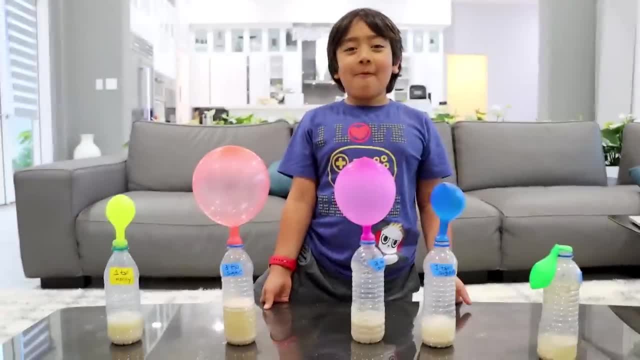 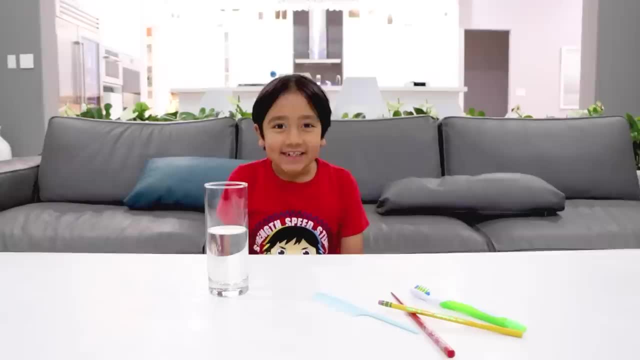 also. maybe you could use like syrup or anything that's sweet. what about syrup? please Salt. What do you think salt will do? right, Yeah, if you guys test it out, let us know. Hey guys, today I'm gonna show you three really cool water refraction tricks. 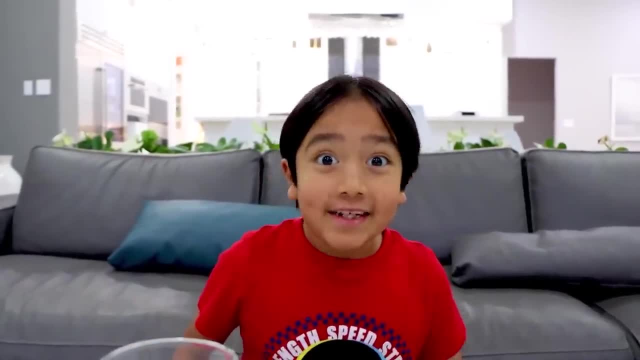 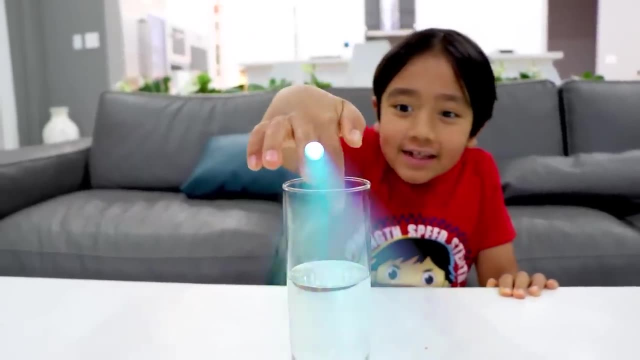 What is refraction, you ask? Well, refraction is the bending of light while it passes through a new medium. So the light is going through the air and then suddenly it goes into the water. All you need is a glass of water. 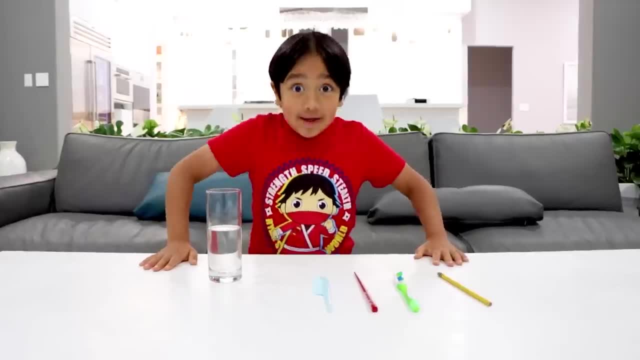 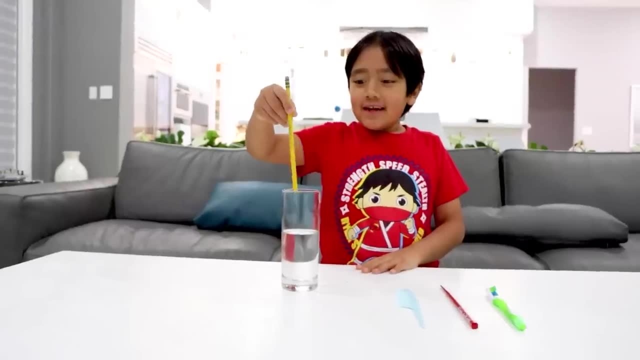 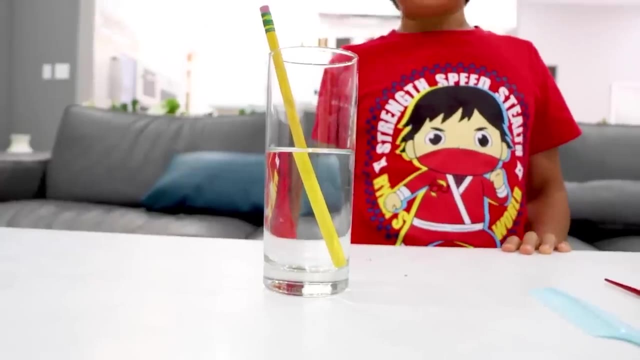 and some objects around the house. It could be anything, but these are the objects I chose First. let's try it with a pencil. So see, it's going here, and then it bends And it looks a lot bigger too. Guys, did you see how the water 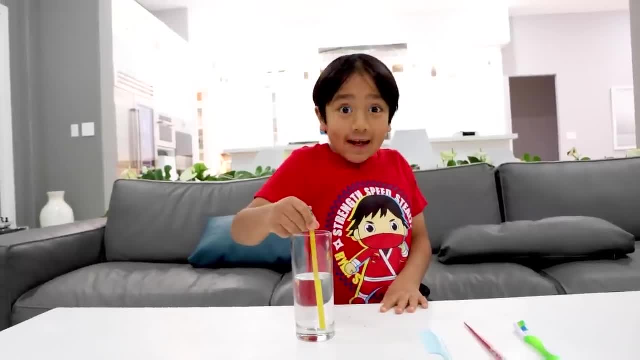 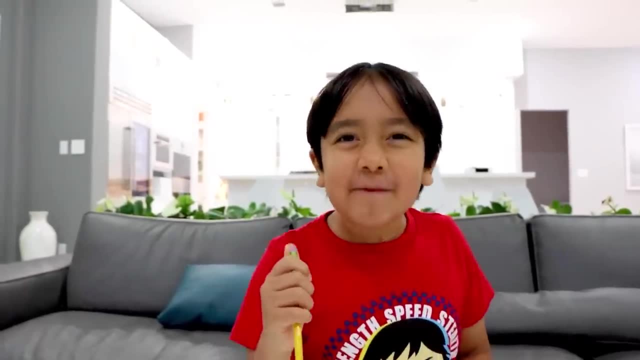 makes it look like the pencil is bent. That's really cool right? Well, my pencil isn't actually bent, it's just refraction, It's bending of light. Okay, let's test out other objects to see if it works too. 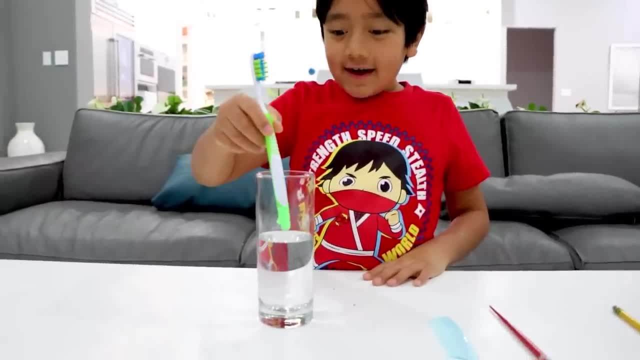 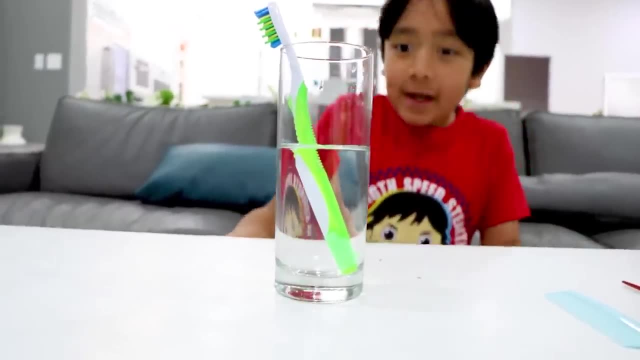 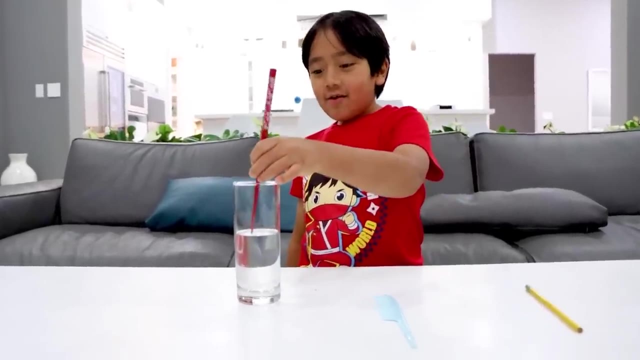 Let's test out this toothbrush. Okay, Whoa, it looks so much bigger And it bended too. That's so cool. but what about Chopstick? Okay, here's the small part. It's getting bigger, bigger, bigger. 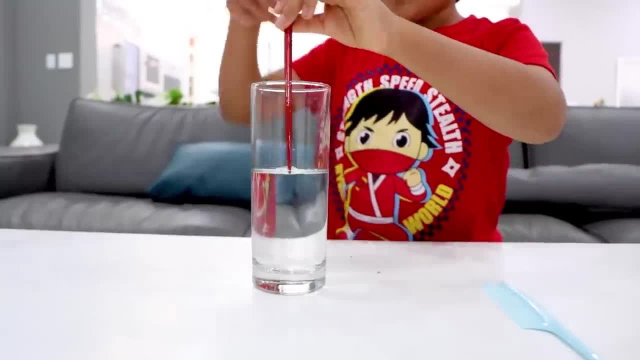 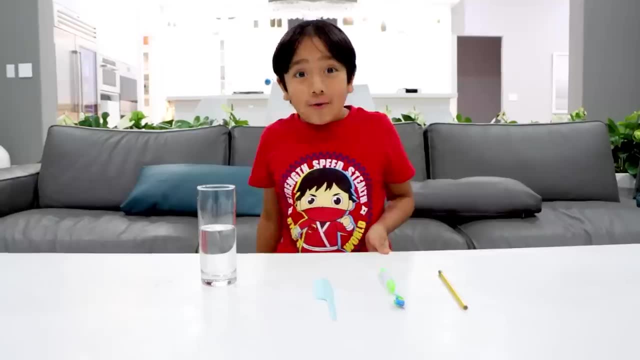 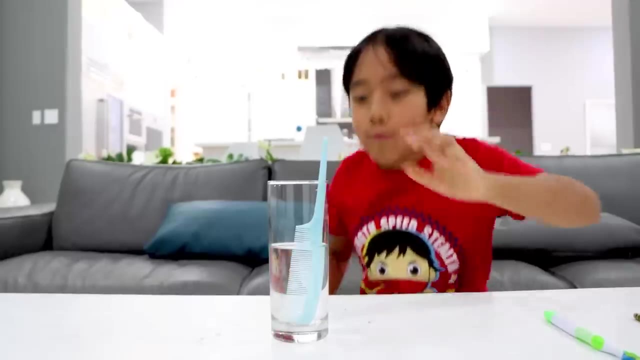 Boom, Whoa, that's super big. Let's try the other part. that's already big. Whoa, it's bending and it's super big. Okay, what about this cone? Whoa, Whoa, that's so cool, it's bending. 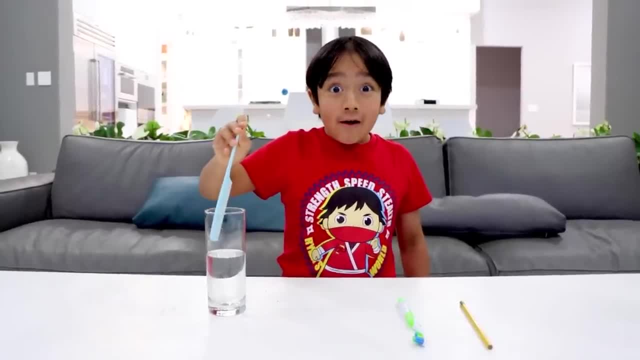 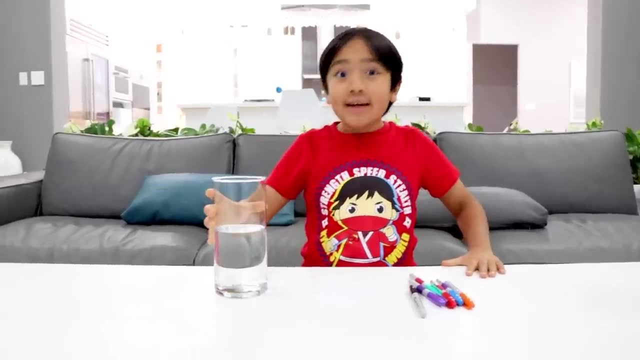 So why did it look like the object bends under the water? Because of refraction, Because of refraction, Because of refraction. On to number two. So for the next trick, you're gonna need a glass of water, paper and some markers. 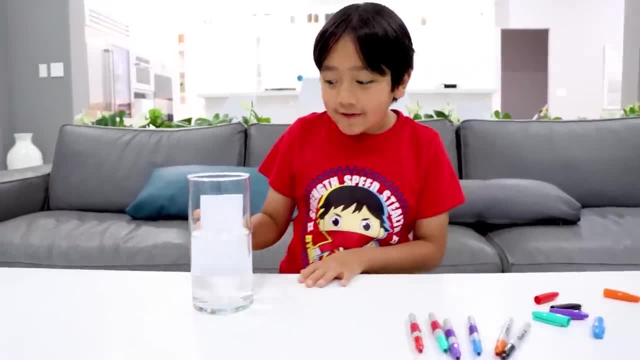 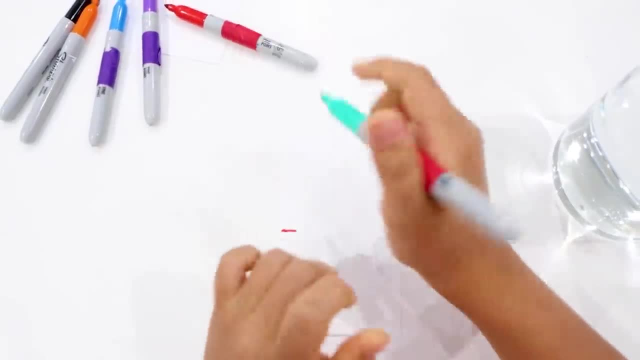 Okay, guys. so for this one, I'm gonna draw it and put it on the other side, and something cool will happen. I'm gonna draw an arrow with multiple colors, So first red and then pale purple and then blue. 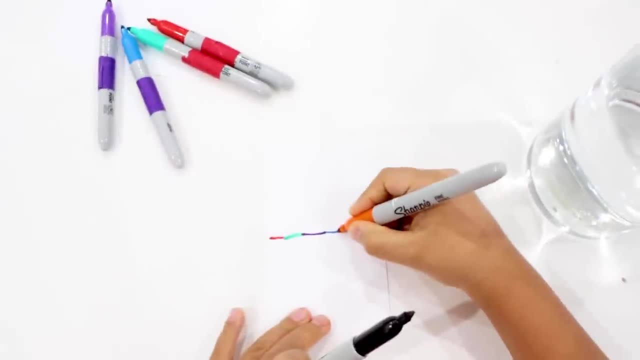 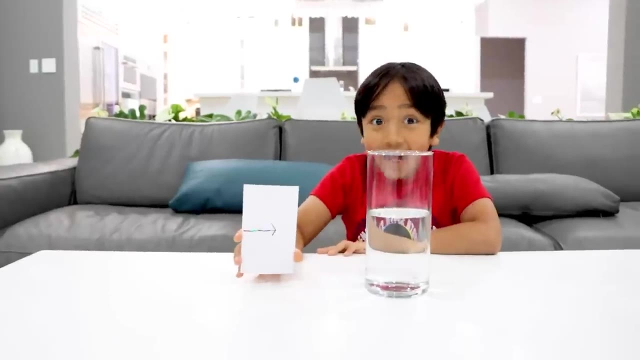 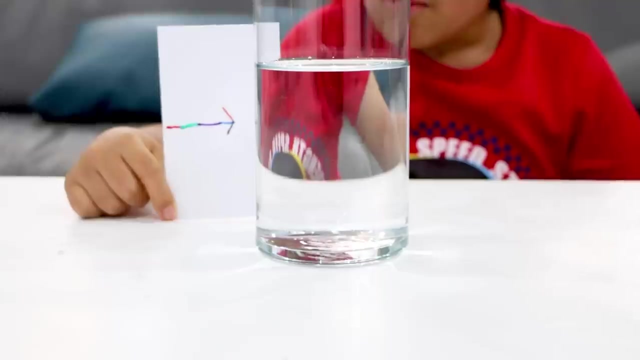 and then orange and then blue, and then yellow, and then orange and then blue, and then orange and then blue. So you guys see that this is an arrow. Well, look at what direction it's pointing at. It's pointing out that way. 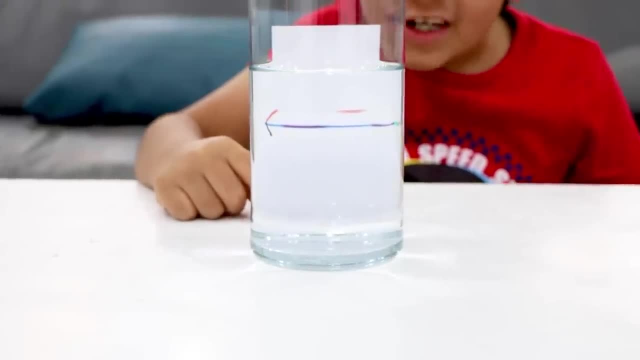 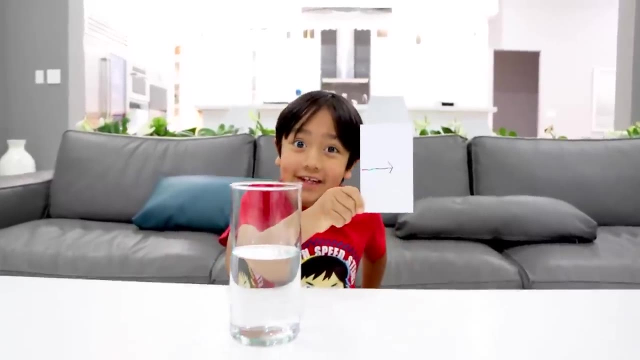 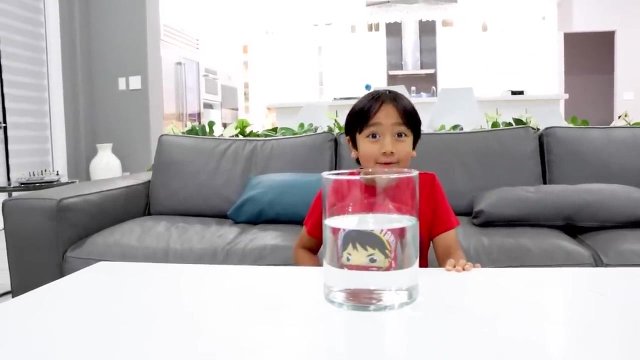 When you put it behind the water, it points the other direction. so it's reversed, Isn't it cool? Well, that's just refraction, Still pointing the same way. now, Before I show you refraction trick number three, here's a bonus one. 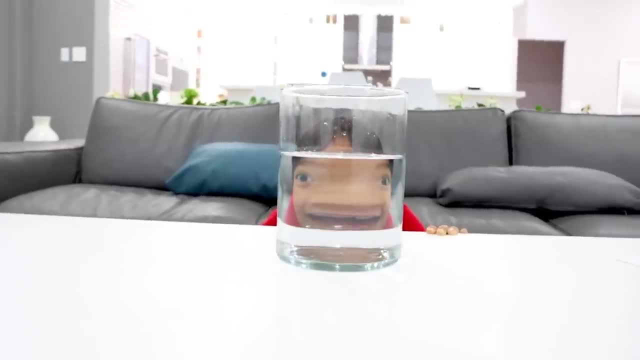 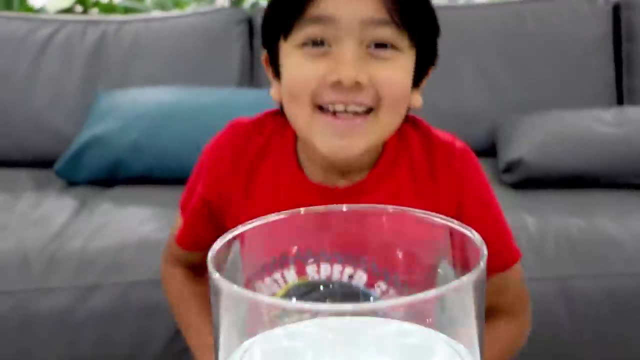 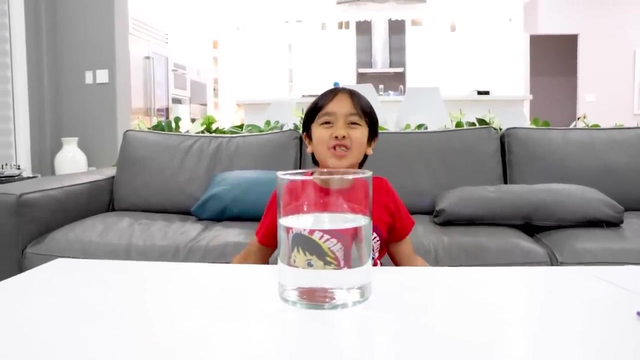 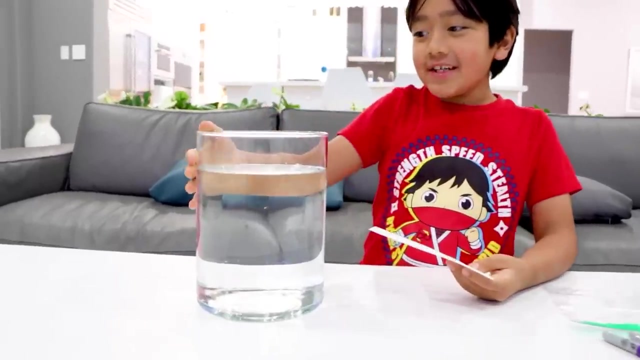 Look what happens to my face. Hi, what's up? Oh yeah, peace. Aww, Now I'm all better again. See, now my face is normal. It's just refraction. Now for trick number three. Okay, so for number three you need obviously. 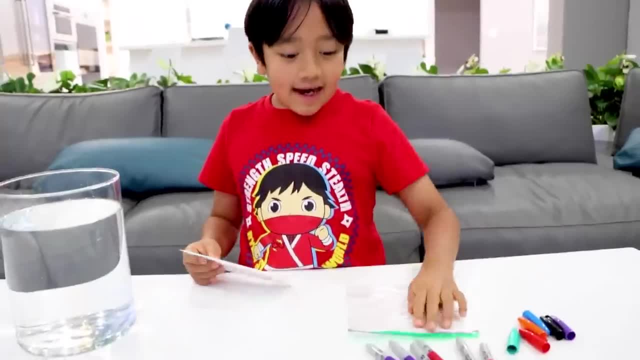 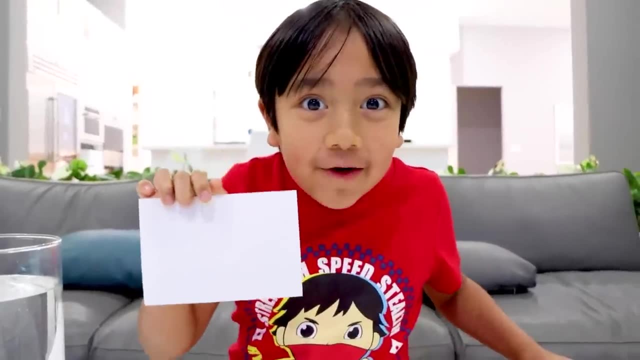 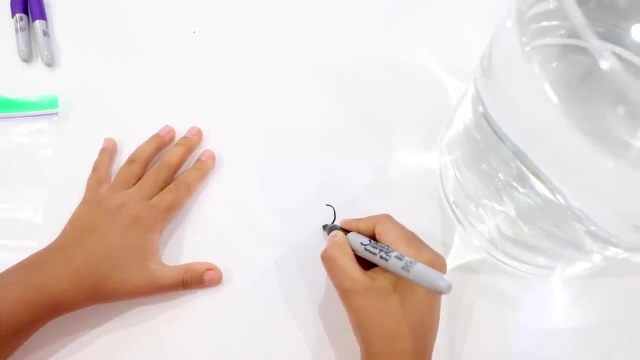 a container of water, some paper and a zipper. You need a Ziploc bag. First step: draw something on here. Draw whatever you want to disappear. Okay, I'm gonna draw a fish Like this, and then a little bit more. 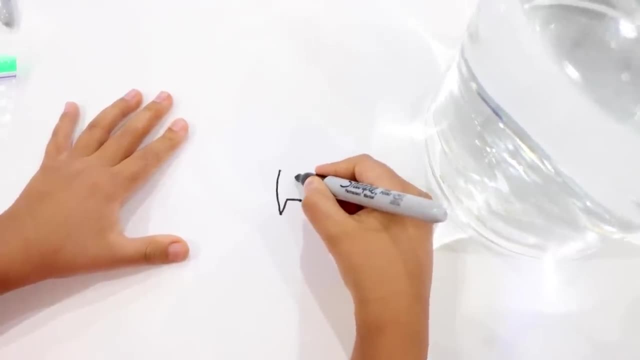 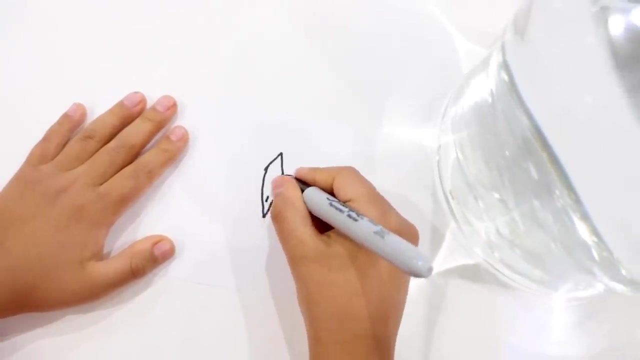 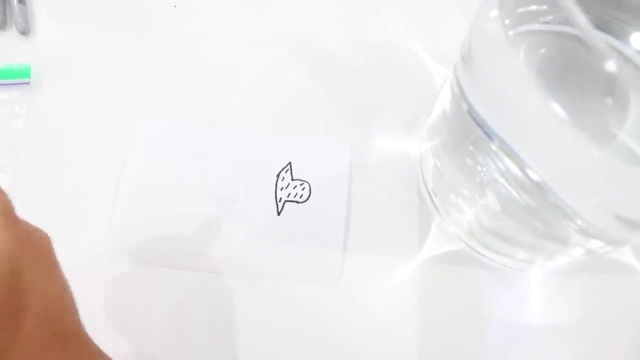 Here, bam, and then here here, here, bam. perfect fish. Okay, I'm gonna draw its scales like this. that Okay, there you go. Then I'm gonna draw an end. Is it perfect? Definitely draw a good fish. 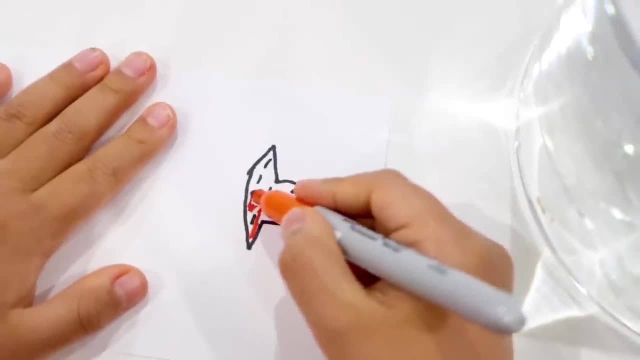 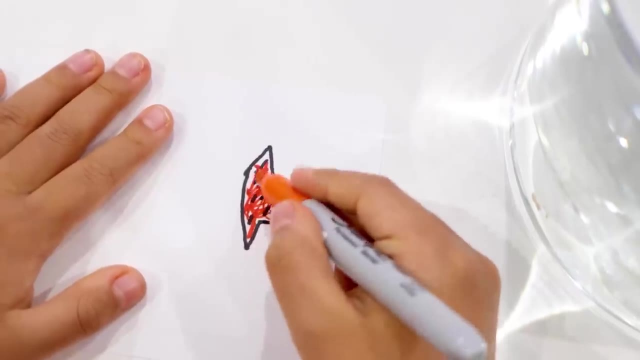 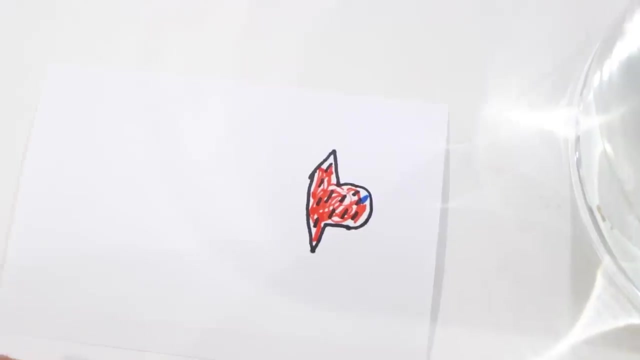 Okay, and then I'll put an eye on this side And then I'll put some running away, some running away dashes. Then you're gonna put it in a Ziploc bag and then put it in a zipper bag Like this, and then I'll put it in my bag. 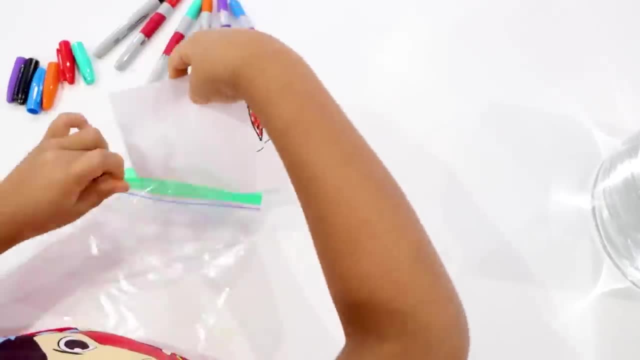 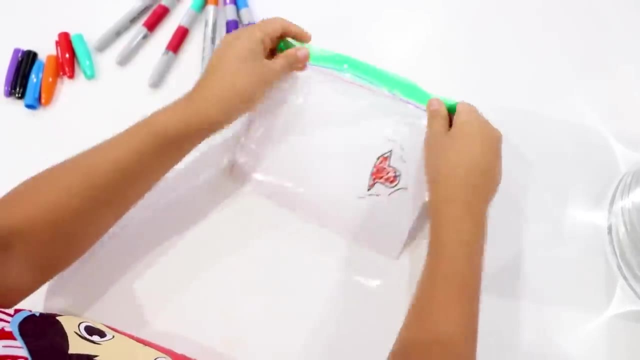 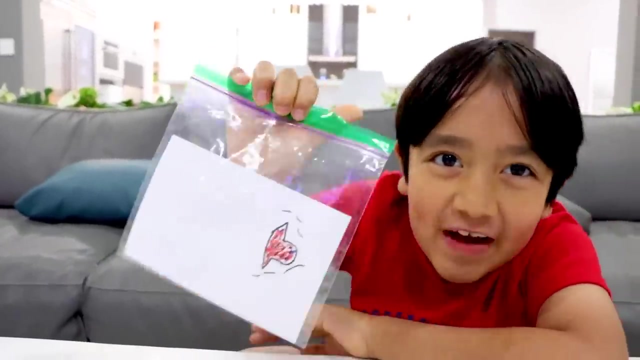 You can put it in any bag. You can put it anywhere- Ziploc bag, Okay, like this. Okay, now I'm done with my fish and I put it in. so now we're gonna draw a shark chasing the fish- Super good shark like this. 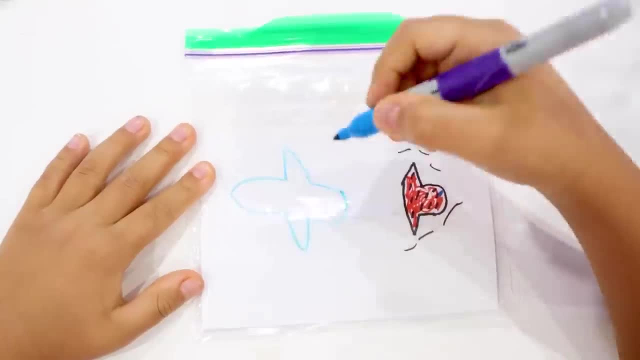 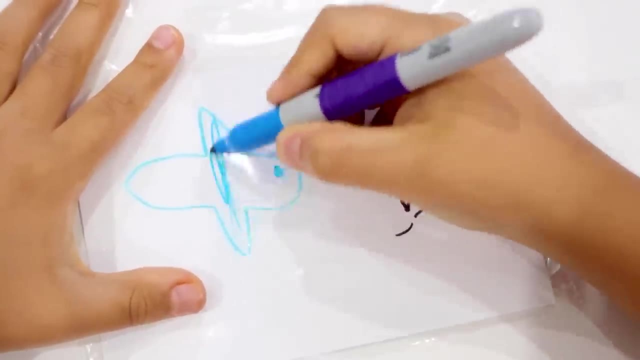 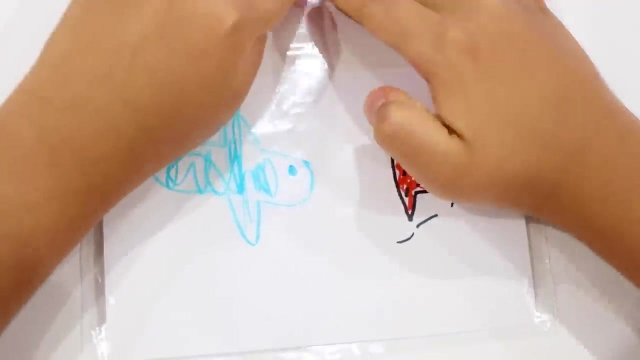 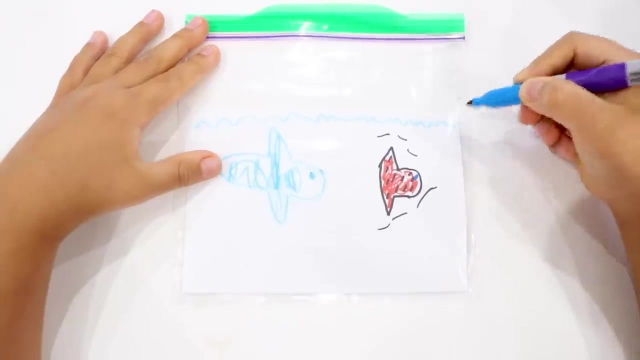 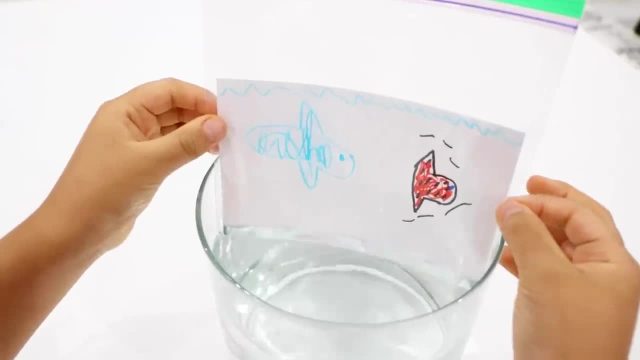 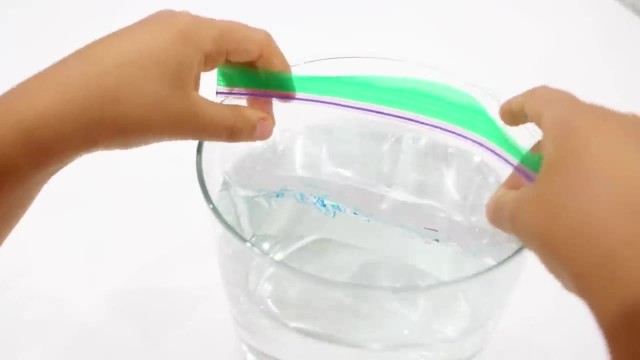 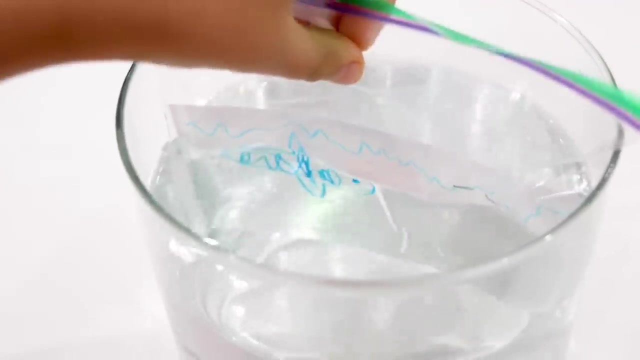 This is what happens when you put it in the water. So the shark is just chasing the fish and then, Boom, fish is gone. Oh, This fish is still here. now it's gone. now it's back. now it's gone. Now it's back now.